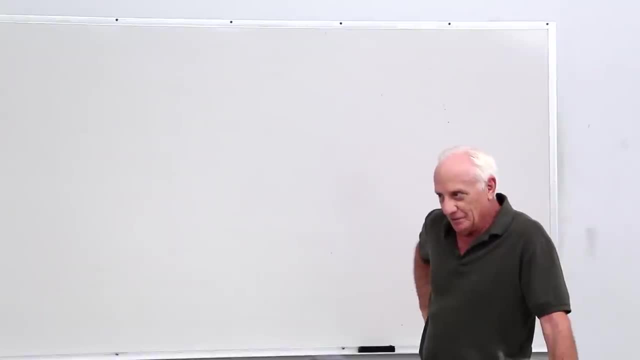 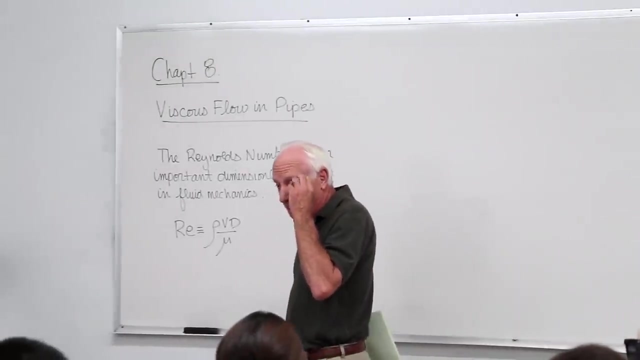 The Reynolds number is probably the most important fluid parameter. It's a dimensionless parameter In fluid mechanics. it's abbreviated capital R, lowercase e, Reynolds. It's defined as the density times the average velocity. B is the average velocity. D is the diameter of the pipe. Typically it's the inside diameter of the pipe, In this case flow inside of pipes. 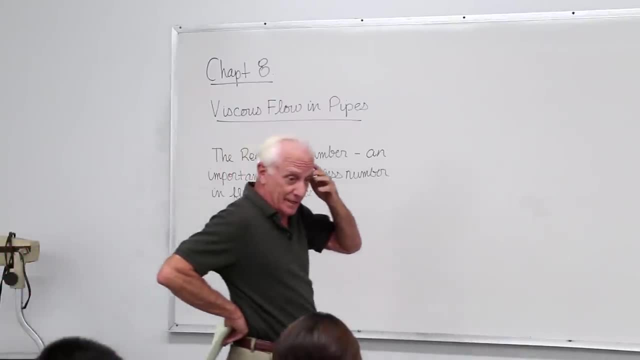 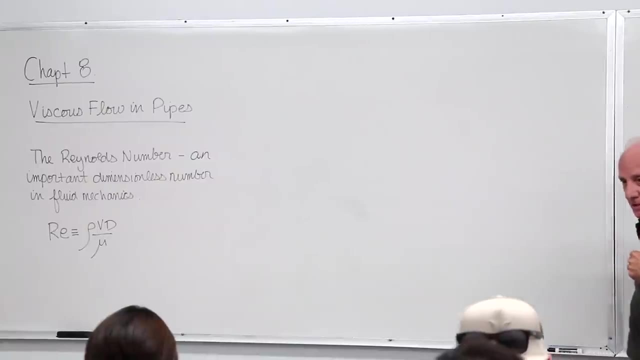 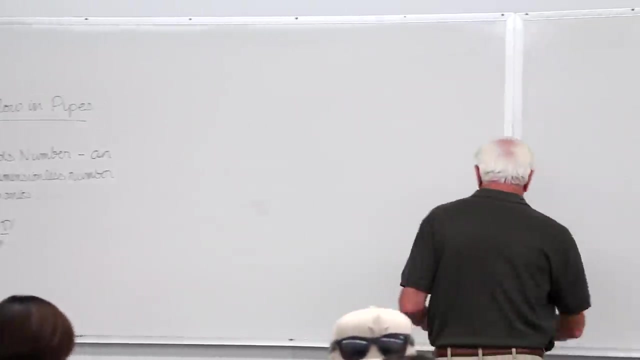 And mu is the viscosity of the fluid in the pipe, Rho is the density of the fluid in the pipe. If you go through those dimensions, you'll see that it is dimensionless. So it's a dimensionless parameter. Now the reason. well, I'll just put some units up here for it, just so we show. 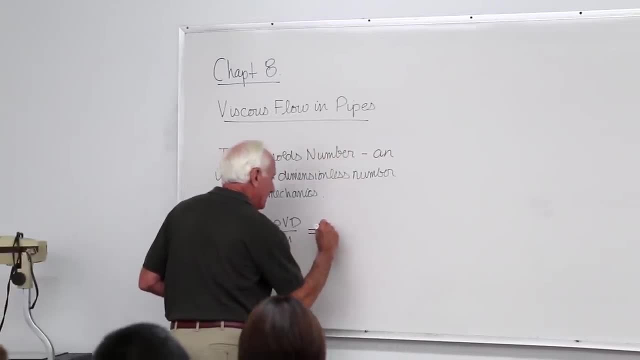 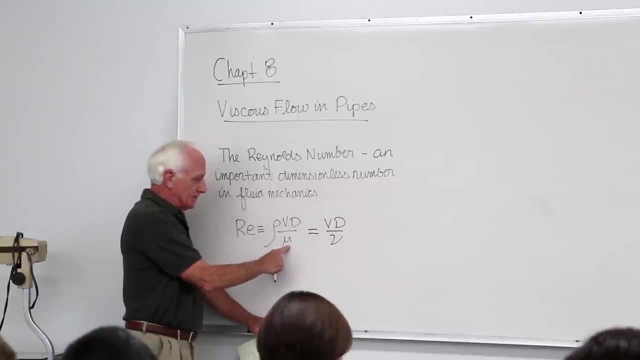 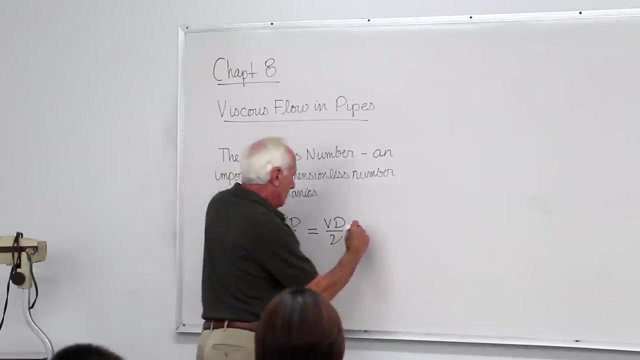 By the way, you can rewrite this guy as VB over nu, because don't forget chapter one. Kinematic viscosity is equal to absolute viscosity divided by the density. Okay, So either one of these two. Velocity, let's just say feet per second. 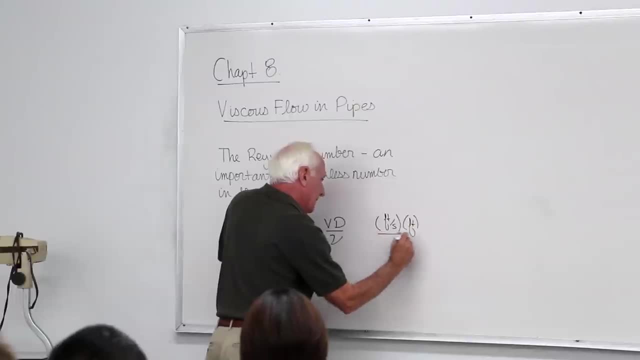 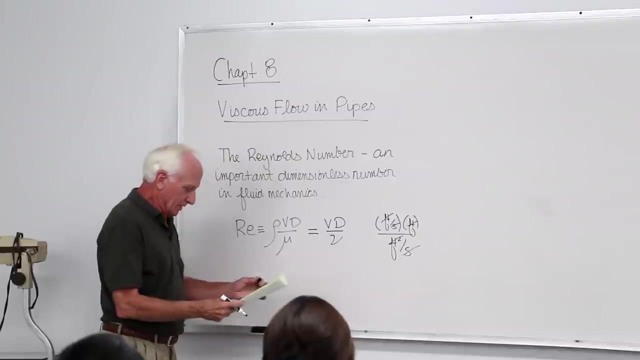 Dimer of the pipe in feet, The absolute viscosity inside the cover of the textbook, Feet squared per second. Cancel, cancel, cancel, cancel, cancel. Yep, it's dimensionless. Okay, Now we can also talk about why it's important. 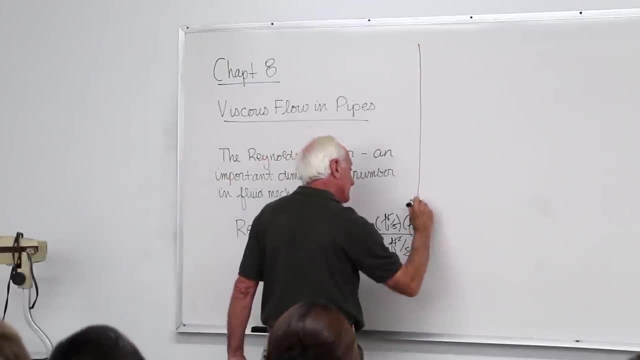 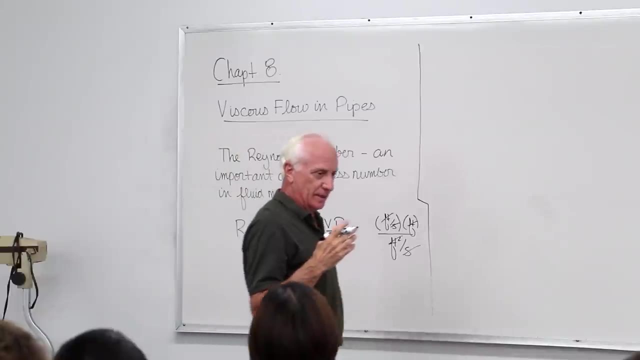 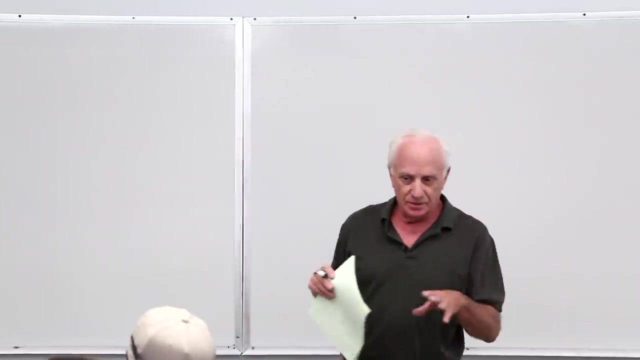 For one major reason in fluid mechanics is it tells us whether the flow is what we call laminar or turbulent. There can be two types of flow in a pipe. We divide it that way. We say either the flow in a pipe can be laminar or it can be turbulent. 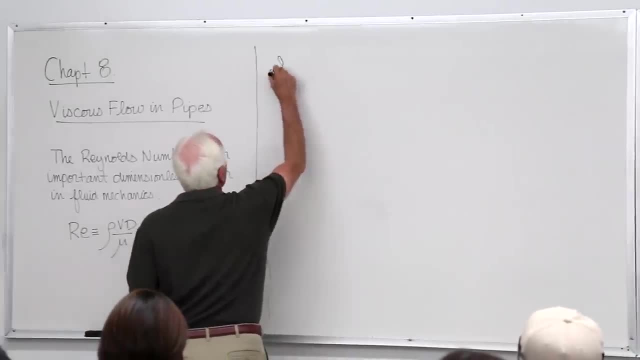 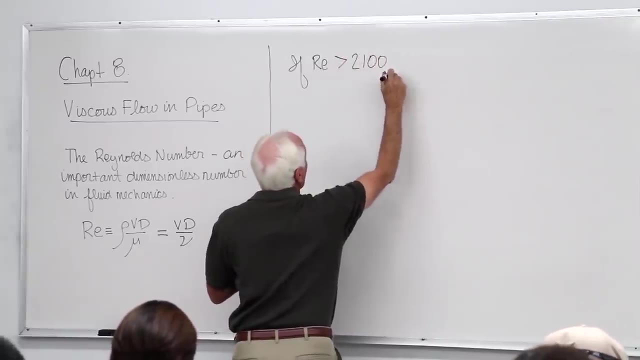 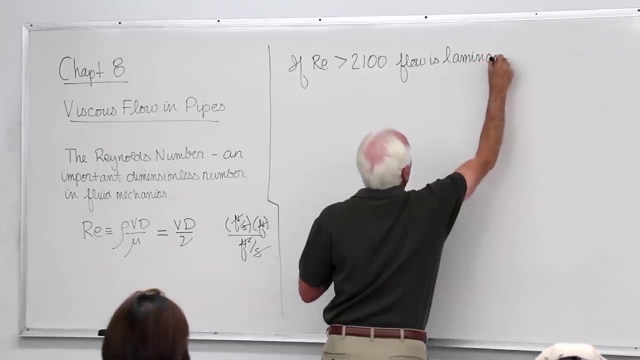 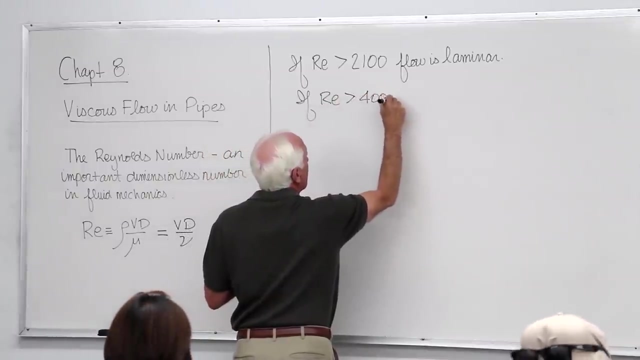 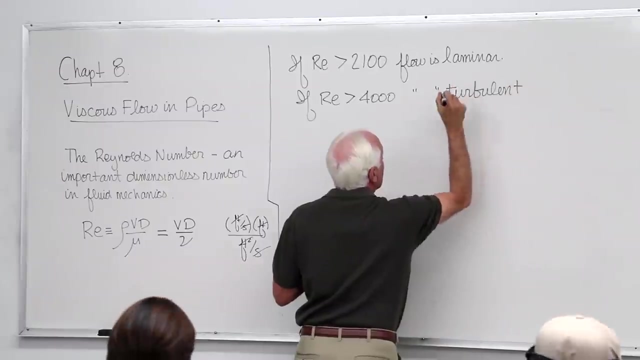 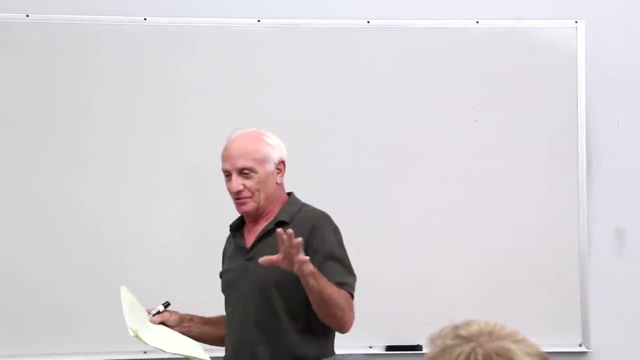 So if the Reynolds number is greater than 2,100, flow is laminar. Now, if we say that the flow is has a Reynolds number greater than 4,000, the flow is turbulent In between those two numbers. it's a transition zone. 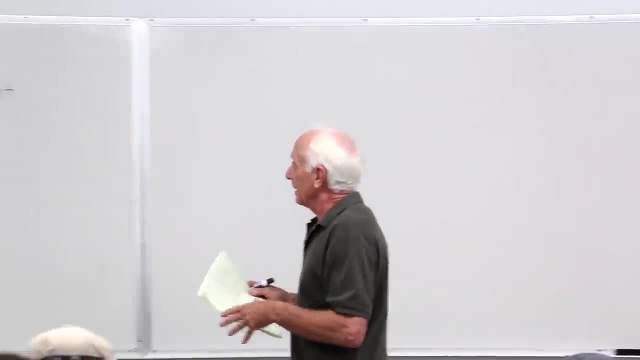 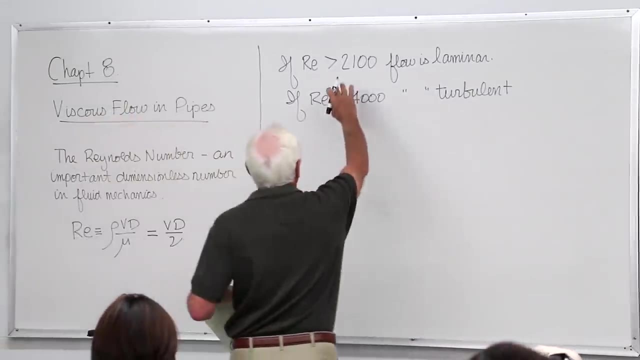 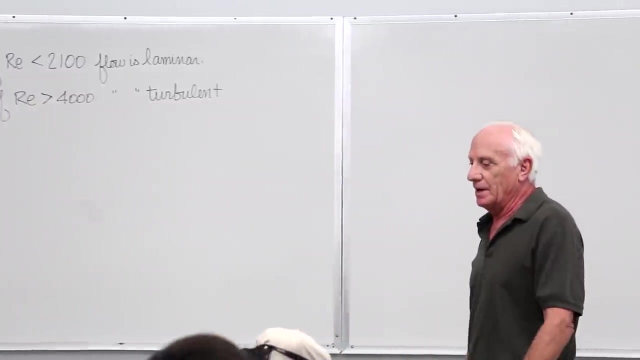 We'll wait until Monday to talk about that. Between 4,000 and 2,100.. Do you mean that a Reynolds number is less than 2,100? Thanks, So there's that little gray area, The gray area 2,100 to 4,000.. 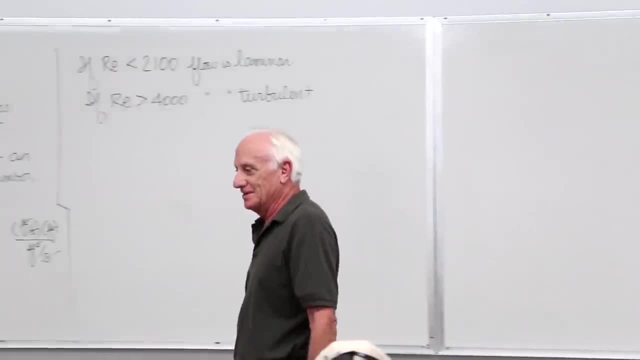 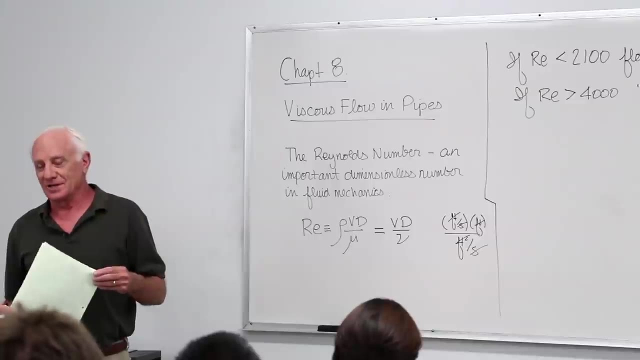 It's called the critical region. The critical region where sometimes we don't know if the flow is laminar or turbulent. So we'll discuss that later. We'll discuss that on next Monday. For right now, the two zones: Okay. 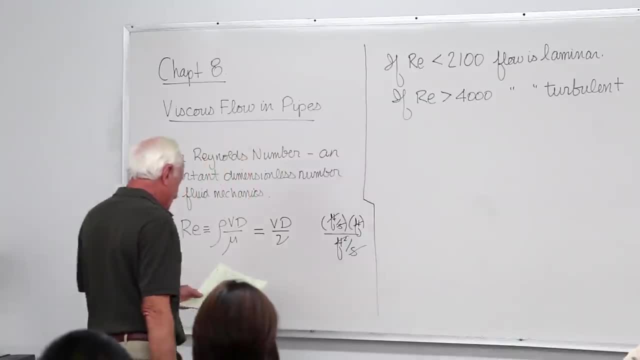 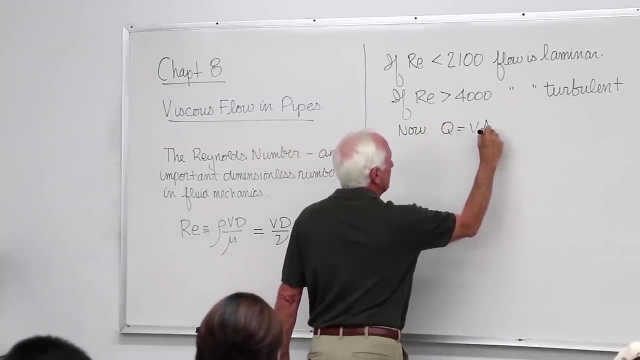 If we want to rewrite the Reynolds number, we can change the velocity in terms of the volumetric flow rate. So now we're going to say Q equal V times A. So wherever you see a V in the Reynolds number, put a Q over A. 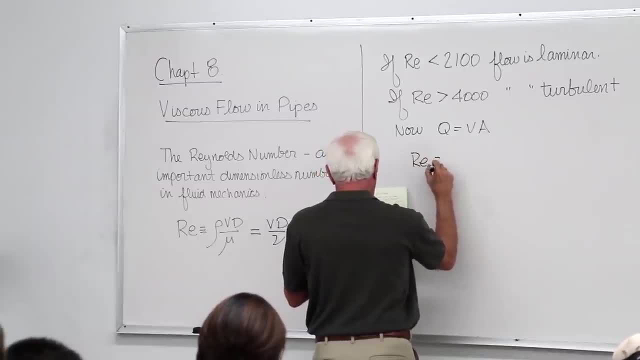 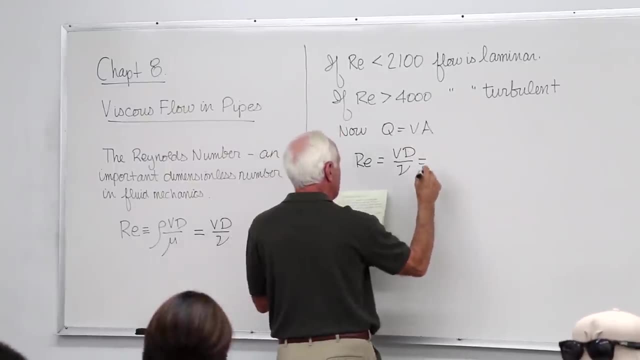 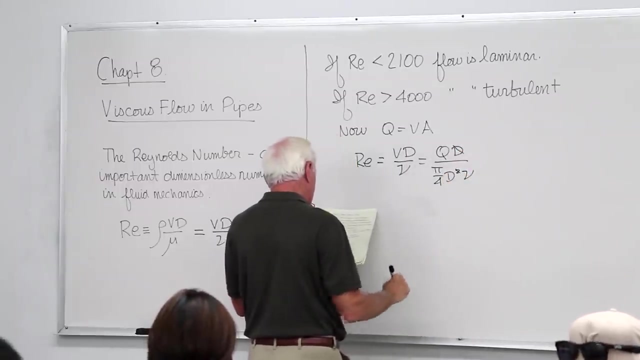 So we have the Reynolds number equal VD over nu. So put it in terms of the velocity Q over A. The area of a circular pipe: pi over 4D squared Kinematic viscosity: nu- VD cancels. 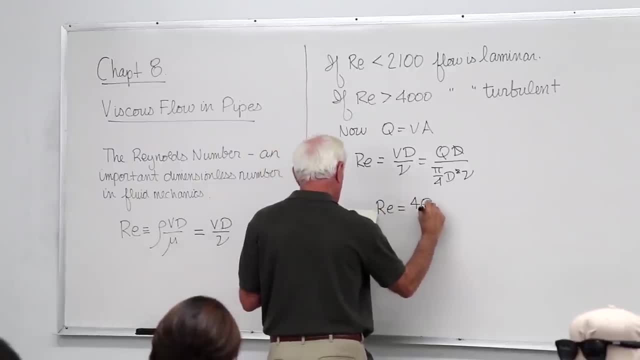 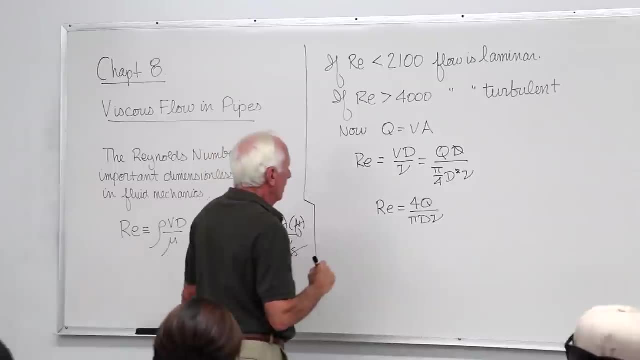 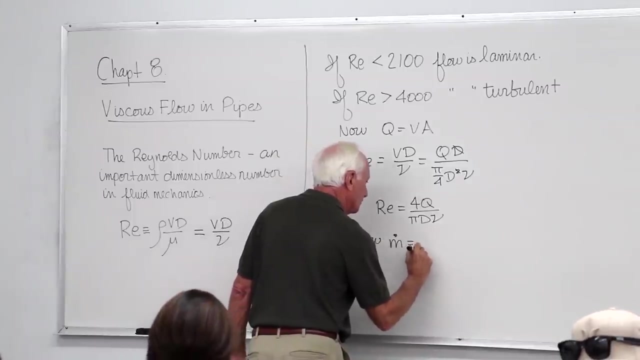 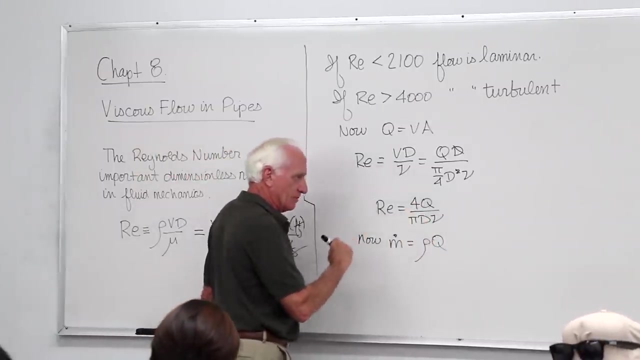 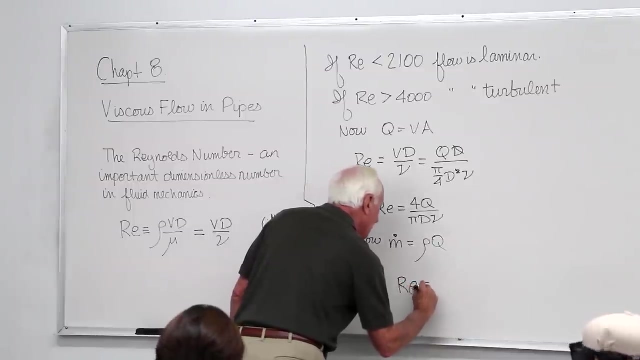 So Reynolds number 4Q over pi D nu. We can now say that M dot is equal to rho times Q. So where we see a Q in the Reynolds number, replace it with an M dot over rho. So we get the Reynolds number. 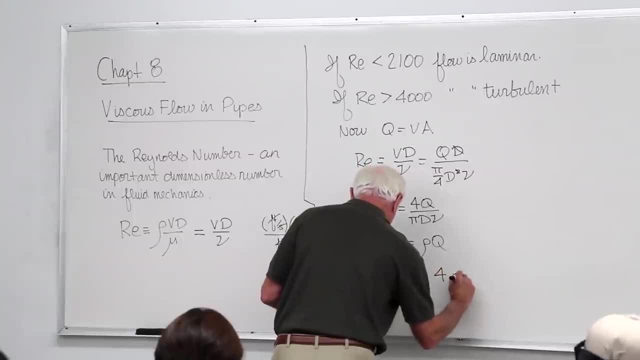 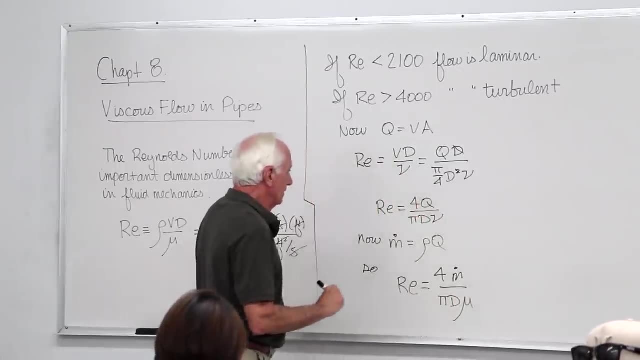 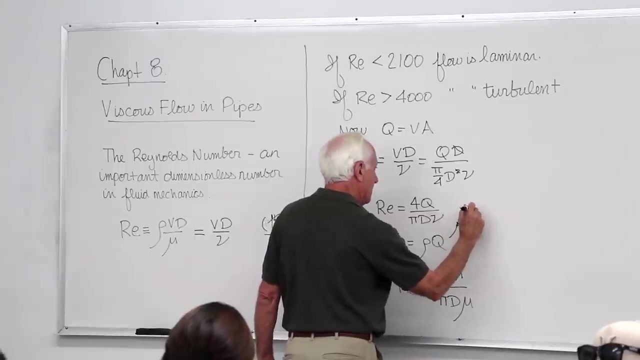 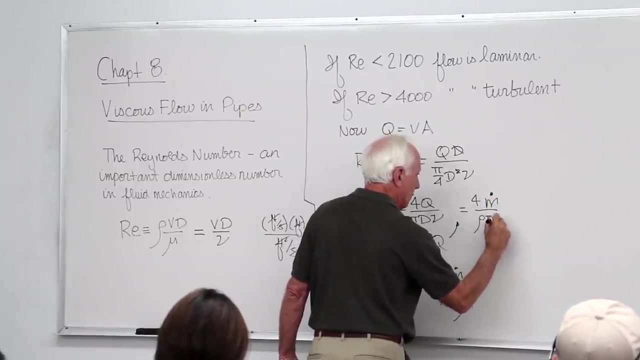 Comes out to be 4M dot over pi D Over pi D mu. Put that into here and you can see what we get. here We get 4Q is M dot over rho, But this guy times, this guy is mu. 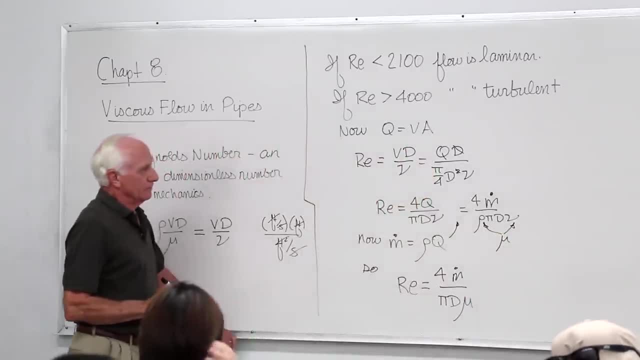 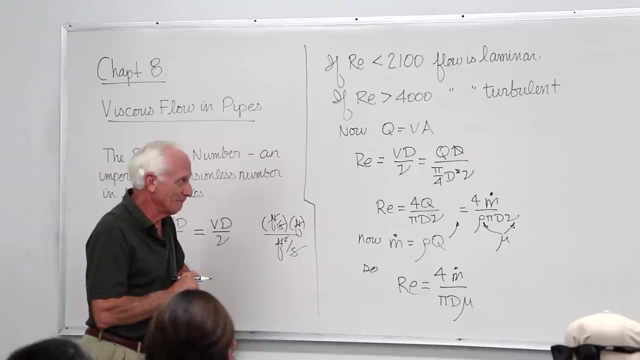 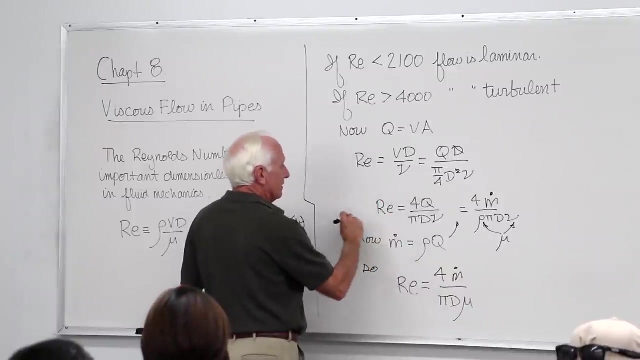 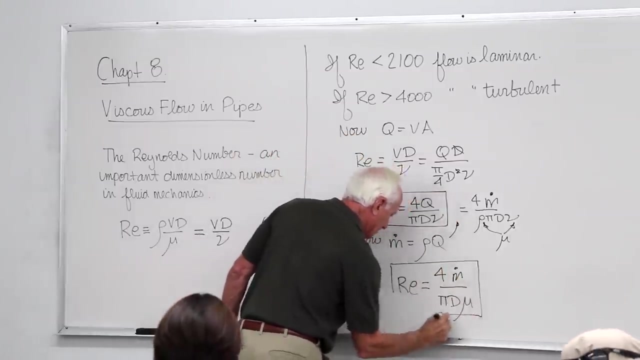 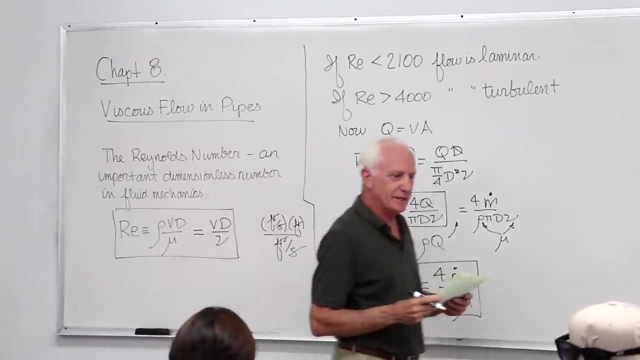 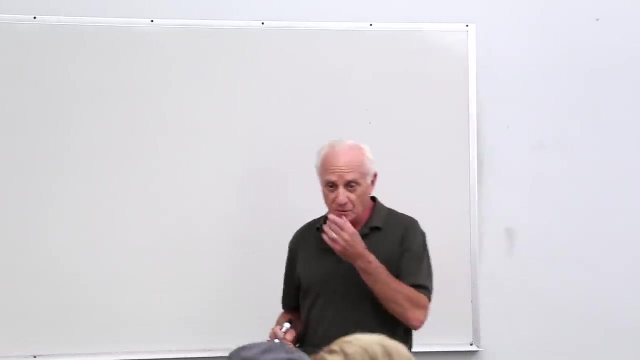 And Nu nu is equal to mu over rho, chapter one. Okay, So now there are different definitions. this was the one definition, this is one And this is one definitions of the Reynolds number. It depends on the problem you're working, which one you 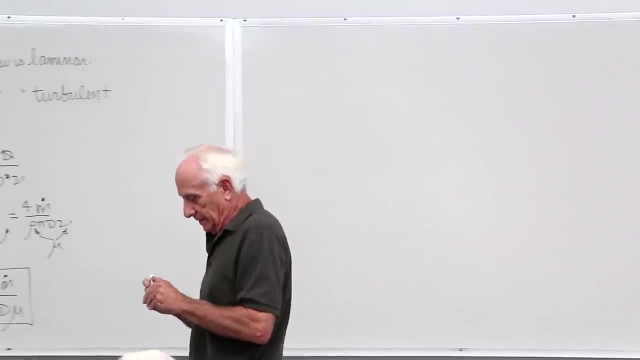 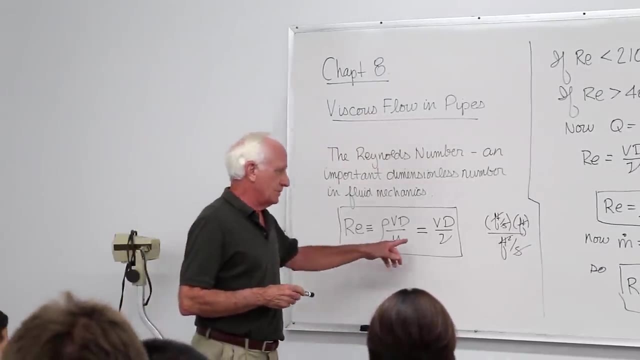 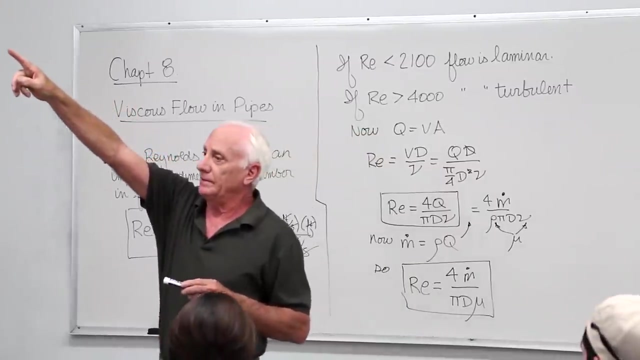 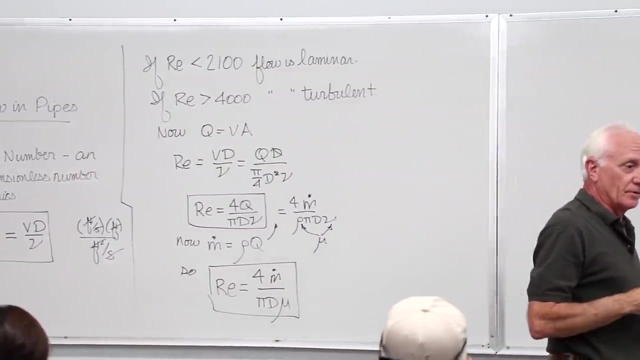 might want to use. For instance, if somebody tells you the velocity in a pipe is 10 feet per second, you'd probably use this one. If you work in the HVAC industry- heating, ventilating, air conditioning- they typically say CFM. CFM, that's volumetric flow rate. 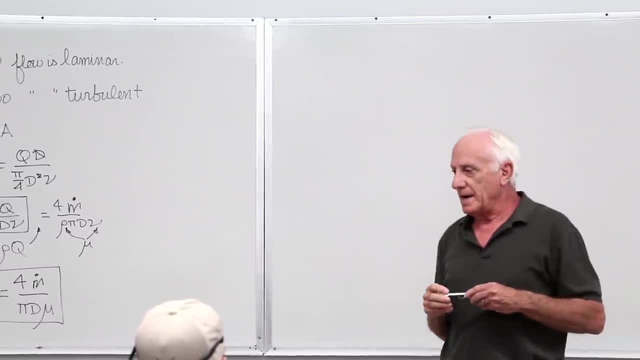 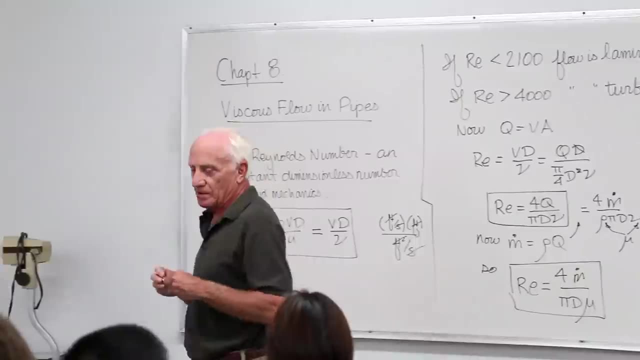 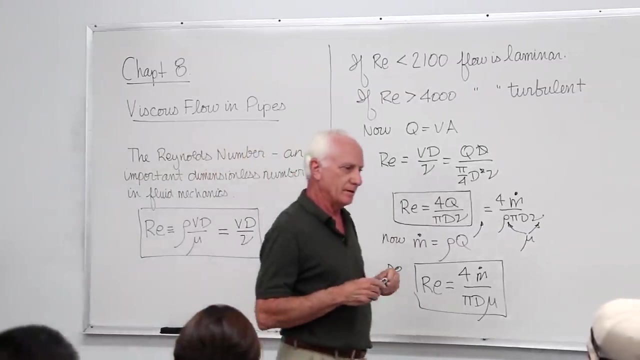 Q volume per ton. If you've got a pump rated at so many gallons per minute, GPM, that's Q, So you'd probably use that definition. Why calculate V if you don't have to? If somebody gives you Q, put it in there. And then, of course, if you're working for Edison. 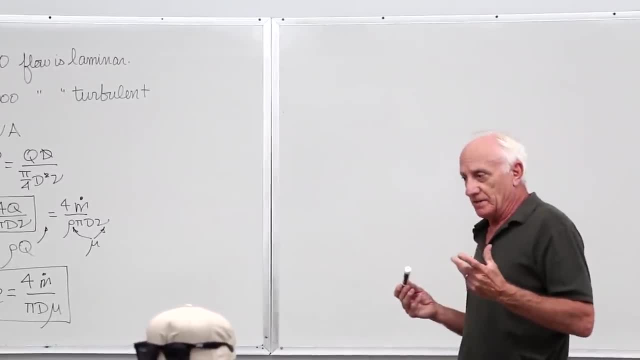 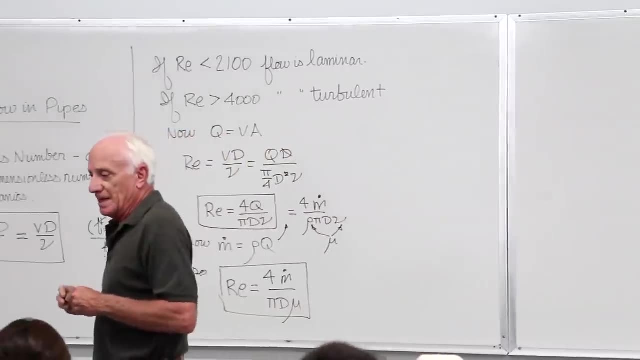 in a power plant- a steam power plant, you'd probably use that definition. Why calculate that? They typically specify the flow rate in pipes or a petrochemical plant: Kilograms per hour or pounds mass per hour. Okay, M dot, Those guys would probably use this definition. 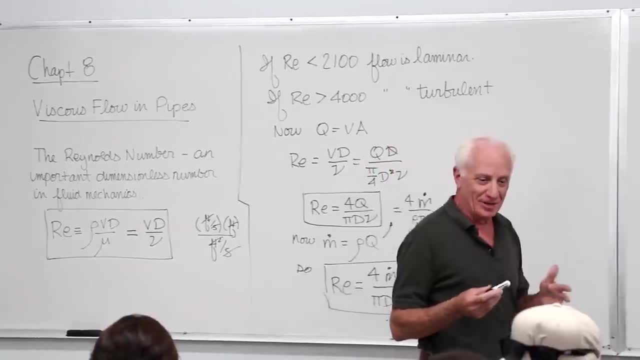 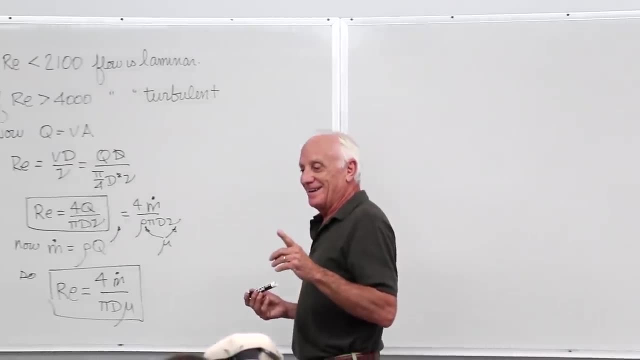 of the Reynolds number. So it depends on what area of engineering you're in, who you work for, which one's most convenient. But generally, generally, nobody's kind enough to give you V. Nobody says the velocity of the gasoline in your gas station is going to be V, So you 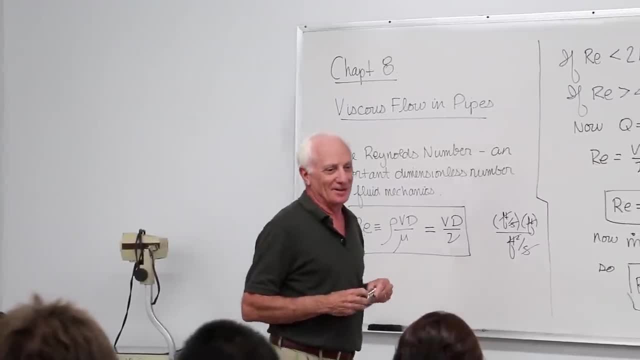 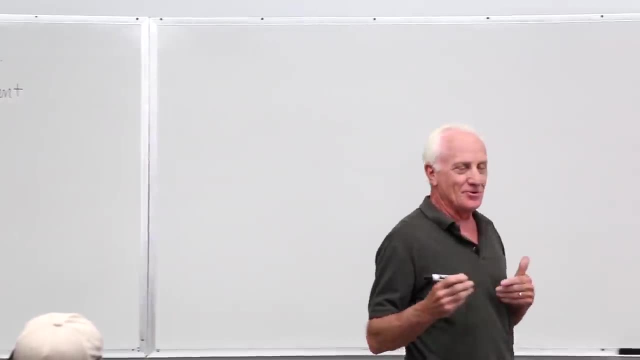 know if your gas line in your car is so many feet per second. No, they don't do stuff like that. They might say gallons per hour or whatever, So normally people give you a Q or an M dot in the real world. But this is the classroom and not the textbook, And we'll 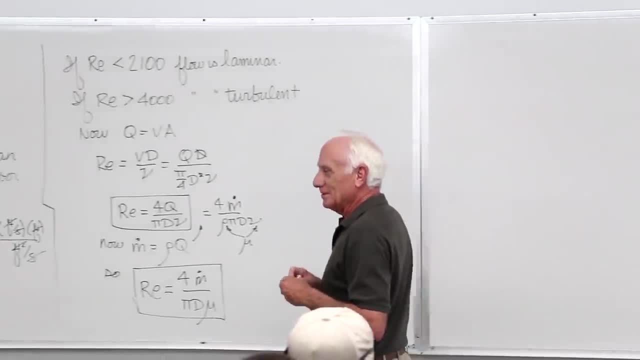 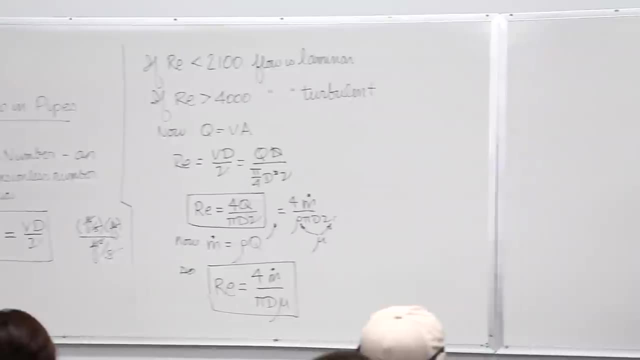 work with the velocity first, because that's the simplest way to go. So, but there's three definitions. They're all dimensional, They're all equivalent, They're all the Reynolds number. This is the rules. Okay, Now some of those guys up in your attic, in your home. they're 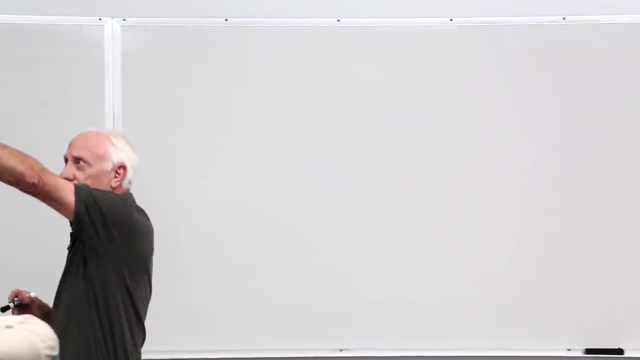 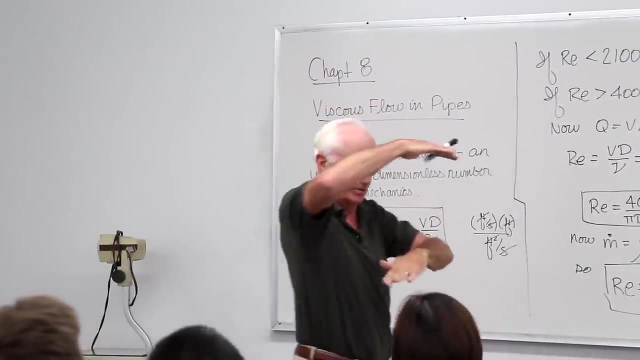 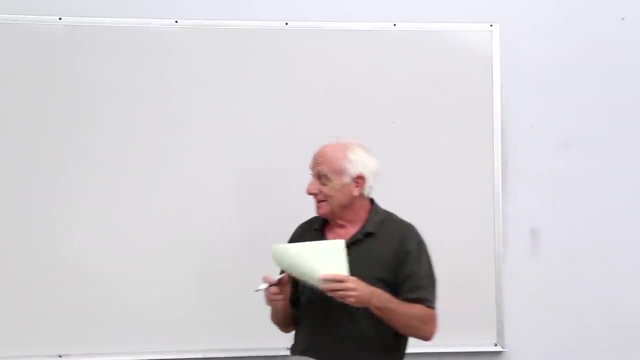 probably round, But in commercial office planes sometimes they're rectangular. These ducts, if you take a look, get the insulation. I look up there they're rectangular ducts, big ones, carrying the HVAC air. So what if a, what if a duct is not circular? And a lot. 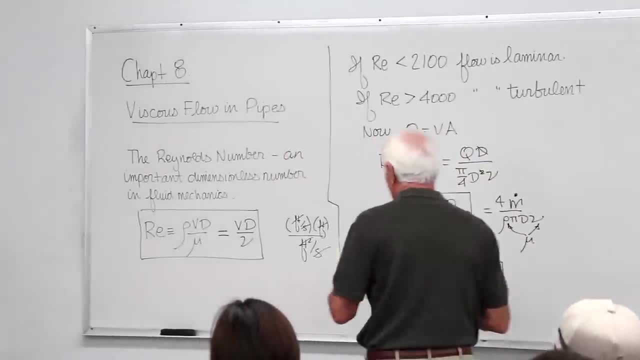 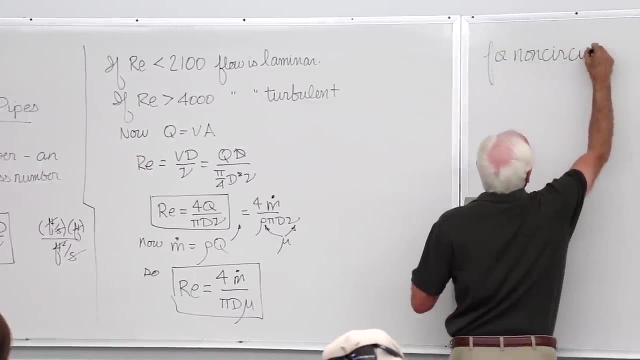 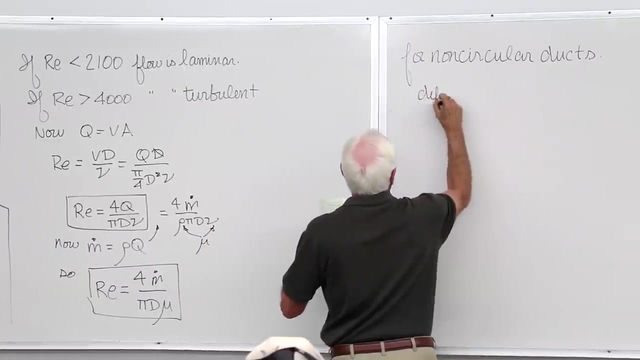 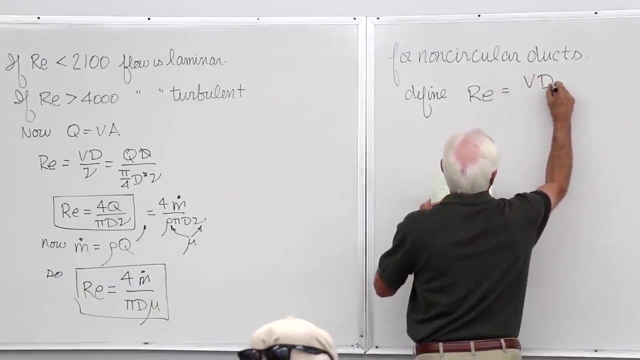 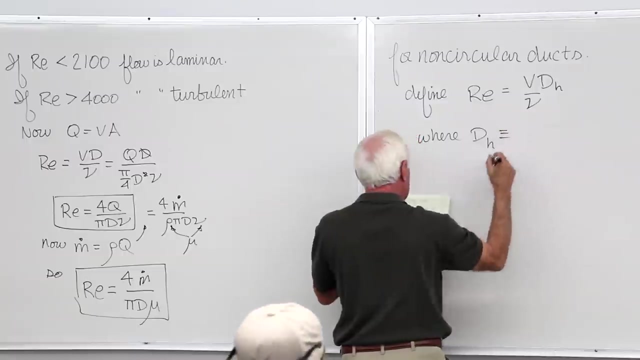 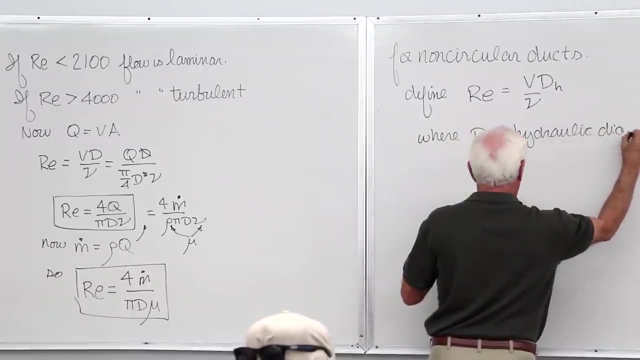 of ducts in the real world are not circular, Okay. So non-circular are non-circular, Okay. Next, we define the Reynolds number as VDH over nu, where DH is defined as the hydraulic diameter, And that's equal to VDH over nu, And that's equal to VDH over nu, And that's. 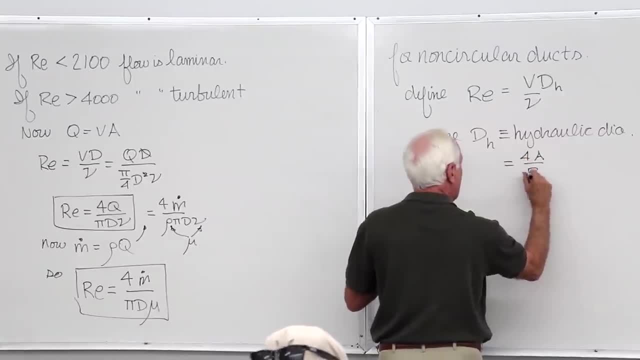 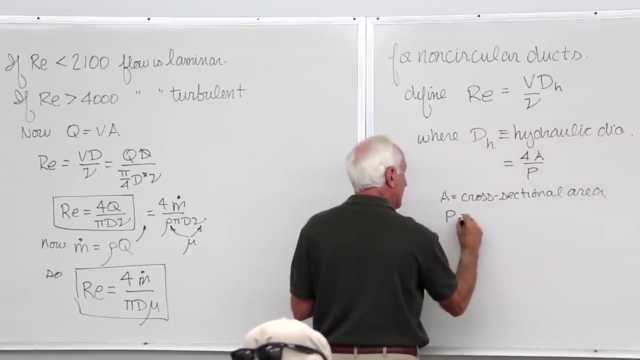 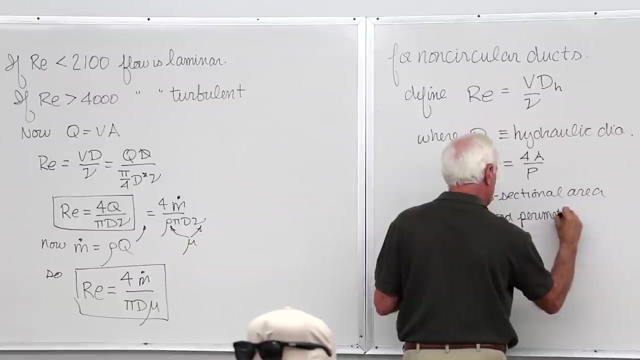 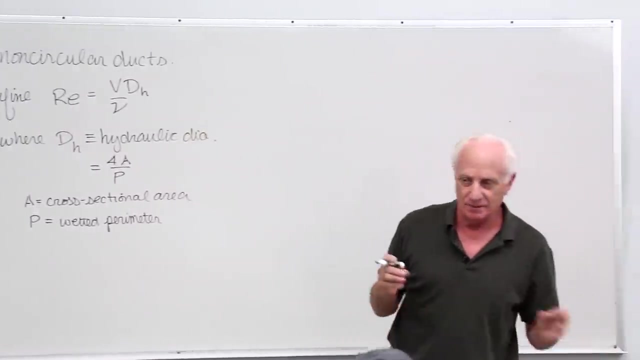 equal to four times the cross-sectional area divided by the perimeter. A equal cross-sectional area, P is defined as the wetted perimeter. The wetted perimeter And that's equal to VDH over nu. The wetted perimeter is defined as the perimeter where the fluid touches the 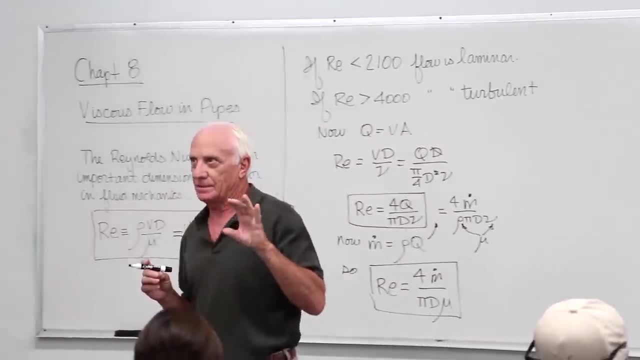 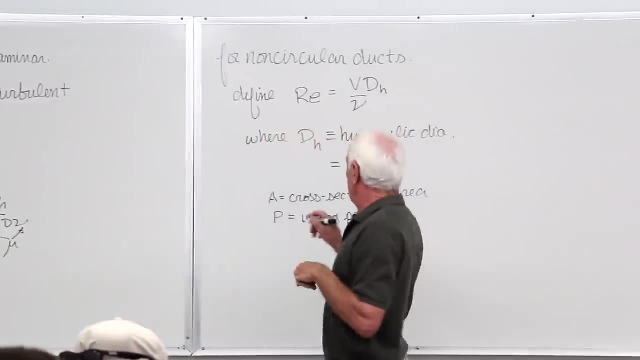 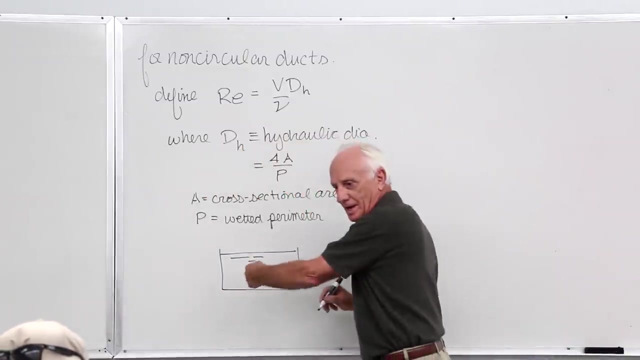 wall. If you've got a circular duct carrying air, the air touches the whole perimeter. If you've got water in an open channel, like sometimes you have in civil engineering, water goes this way: open channel flow- cross-sectional area. I got it Length times height- cross-sectional. 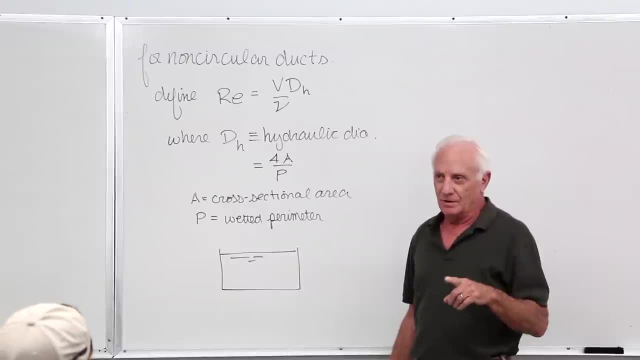 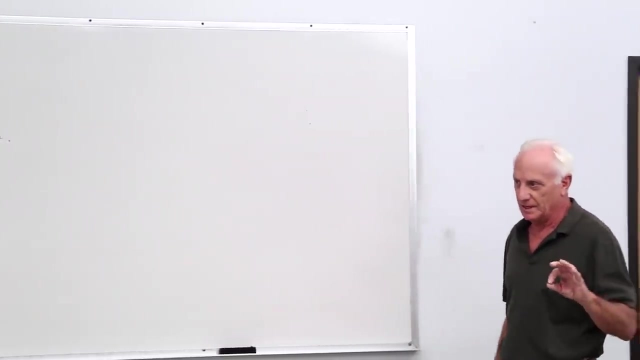 area, Wetted perimeter. okay, here it comes. Where does the water touch the perimeter of the area? Right, left side, the bottom, the right side? no, That's called the wetted perimeter, Where the fluid touches the perimeter of the cross-sectional area. Okay, So we can define. 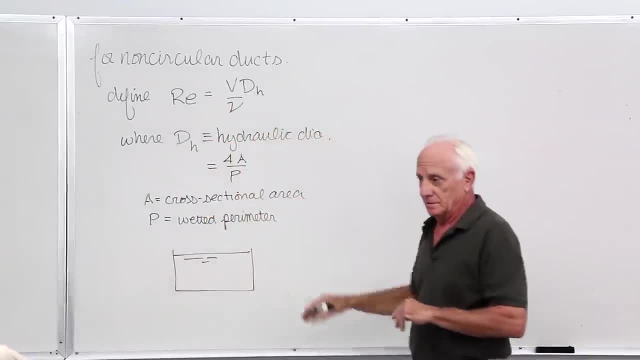 Reynolds number for circular ducts and also for other shapes. Could it be triangular? Well, of course it could. There's definitely a difference between a circular duct and a wetted perimeter. Of course it could. This definition works. The cross-sectional area. 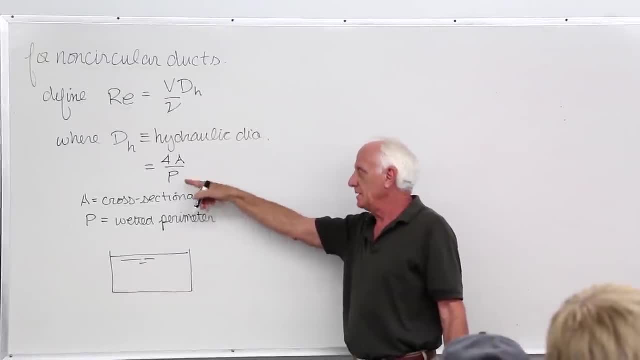 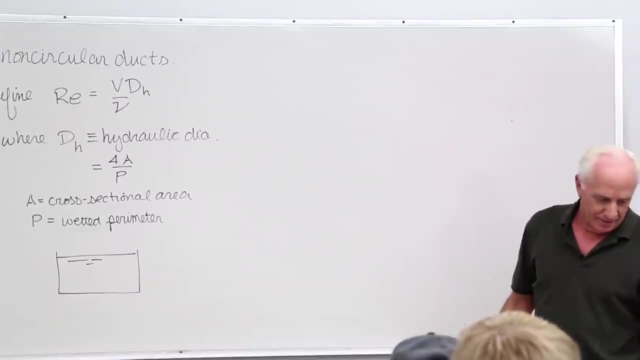 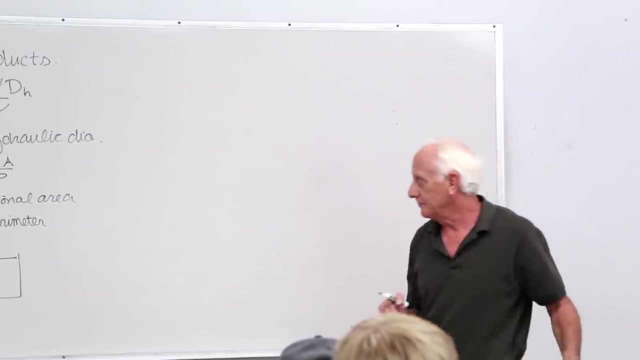 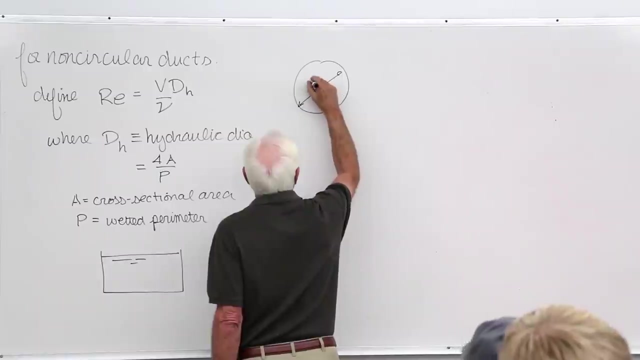 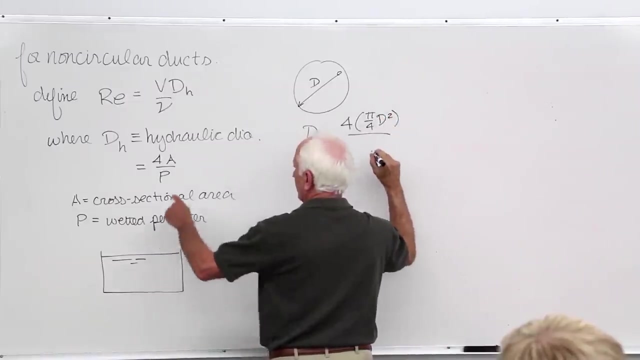 of a triangle divided by four times that divided by the wetted perimeter, where the fluid touches the perimeter of the cross-sectional area. Okay, So I'm sorry, Let's try it for a circular duct. I got it: Hydraulic diameter four times the area divided by the perimeter. Guess what If you? 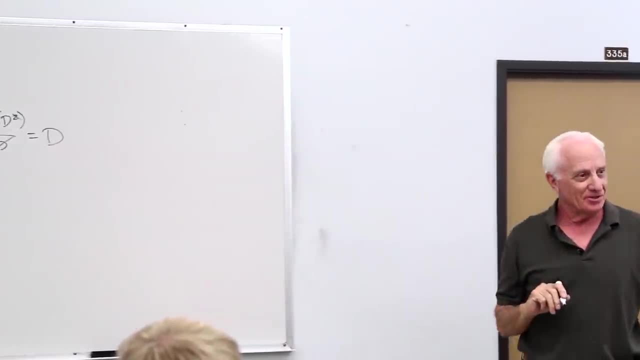 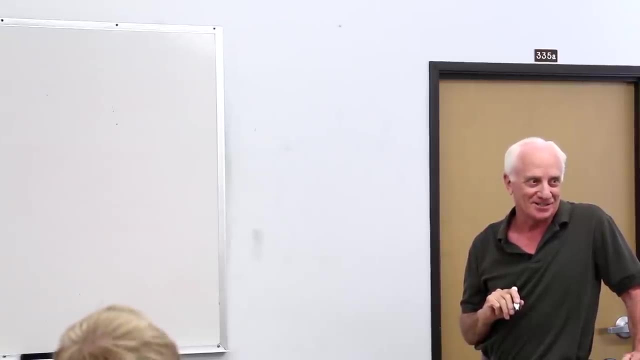 define it like that. with a four, guess what you get for a circular duct Hydraulic diameter. You better get it. You better get it. You want to have the diameter there as a circular duct the same as the duct diameter. If I don't put four in here, guess what I get for the diameter of that thing up there. 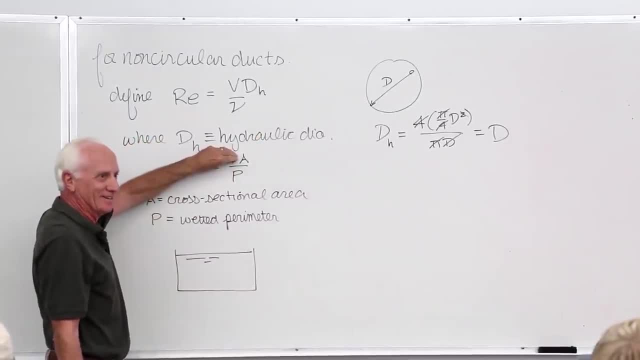 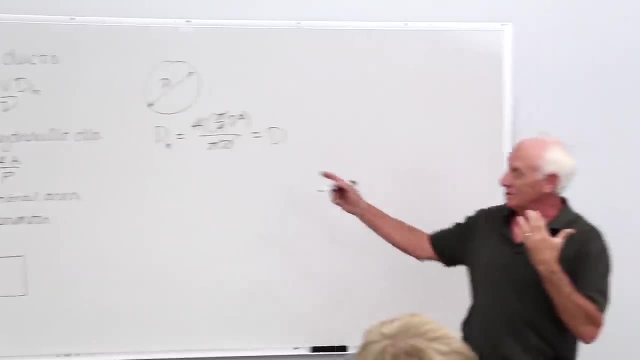 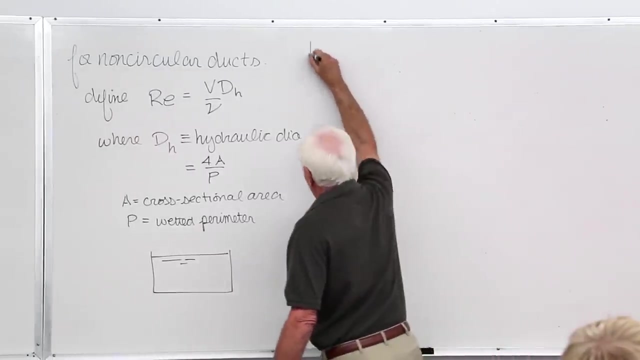 One-fourth of the actual diameter. That's not good. That's not good. Look over here. That's the diameter, So you need the four to make it correspond for a circular duct. Okay, So that's why they do the four in there. Okay, Now let's talk about how the flow of 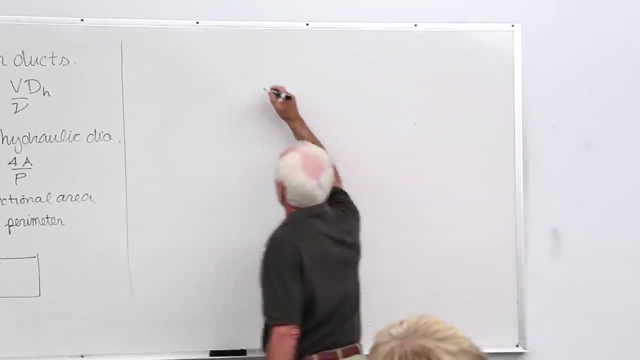 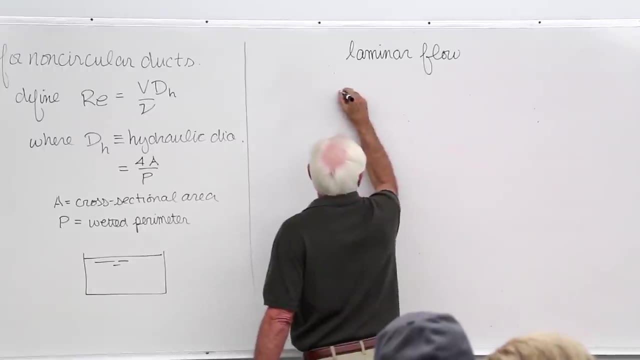 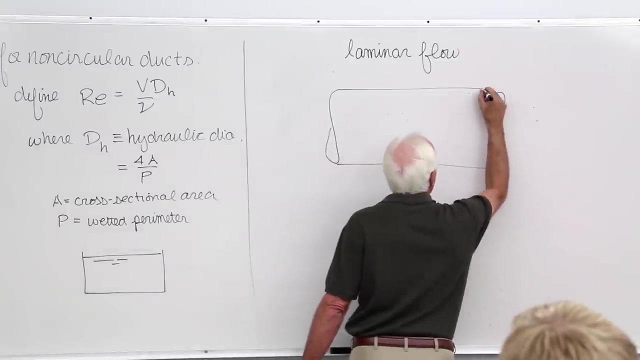 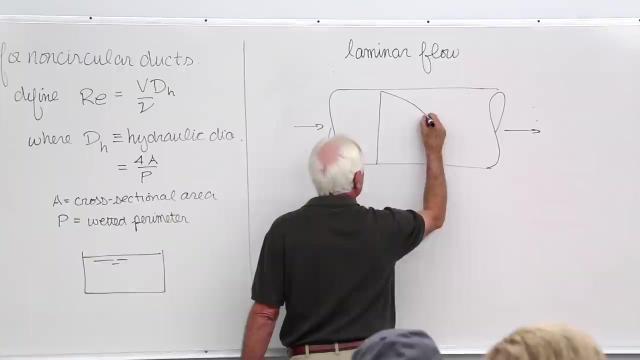 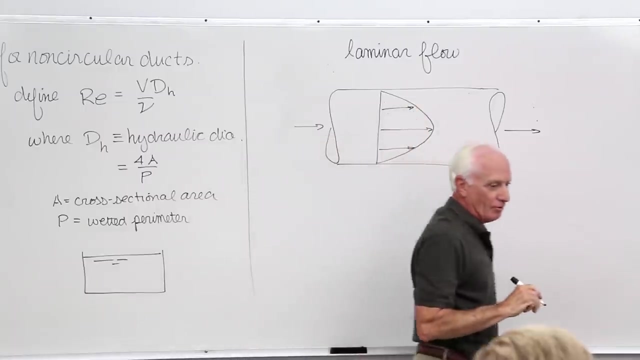 looks if it's laminar or turbulent. First of all, take laminar flow. Okay, Here's the pipe carrying the fluid And it flows going left to right. They call this the velocity profile. Okay, This is the velocity profile. Typically, again, we use lowercase u for the x direction. 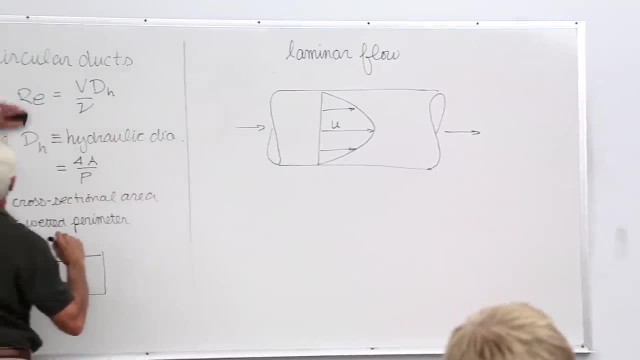 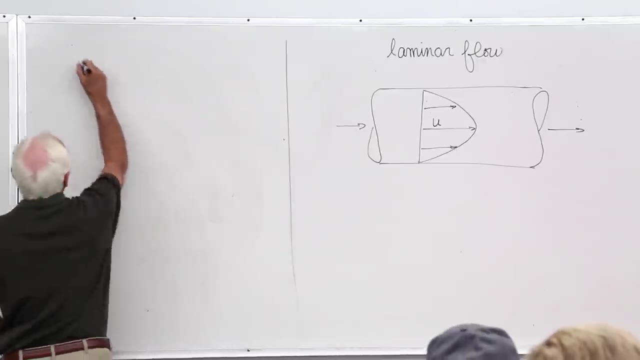 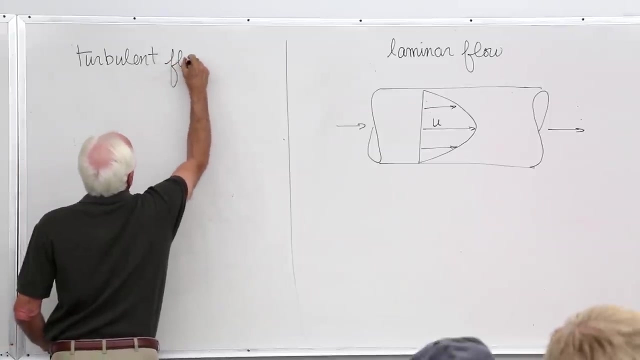 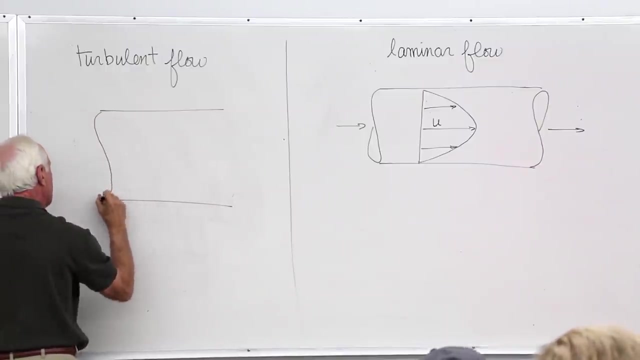 Now I'm going to contrast that side by side here with the turbulent profile. Then we'll talk about the profiles. Okay, The velocity profile for turbulent is not the velocity profile. The velocity profile for turbulent is different than that for laminar. 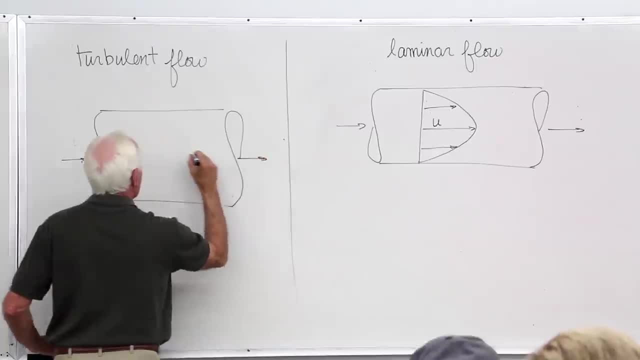 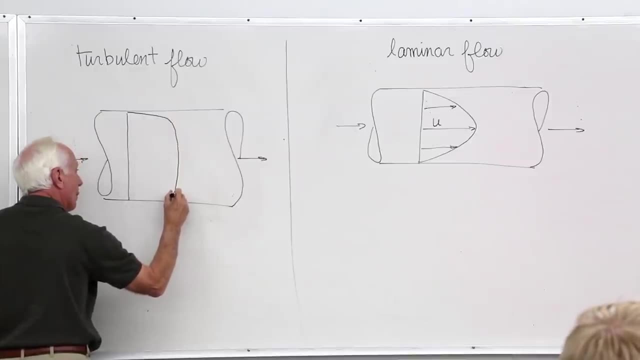 Again, flow is left to right. Turbulent profile is fairly flat across the middle, Fairly flat, Very steep at the walls of the pipe, Very steep at the walls of the pipe, But in the middle part of the pipe it's fairly flat, called uniform, Very near to the pipe. Okay, Now let's talk about the 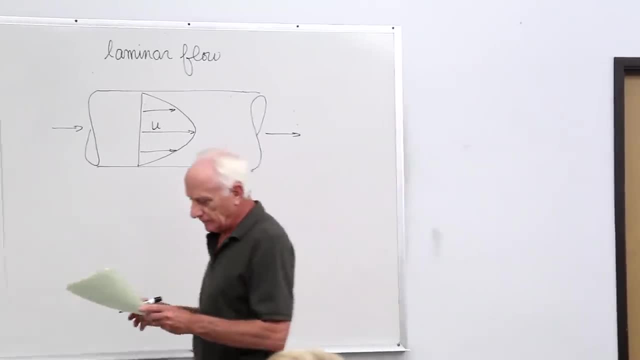 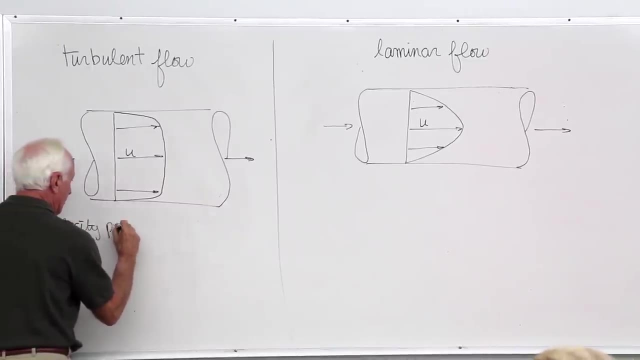 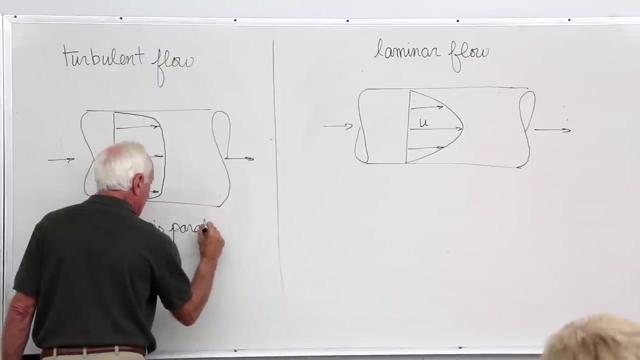 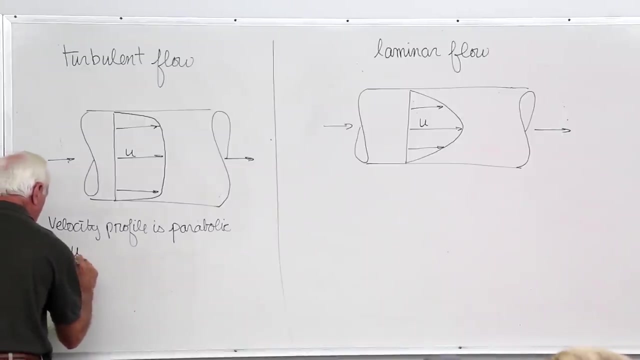 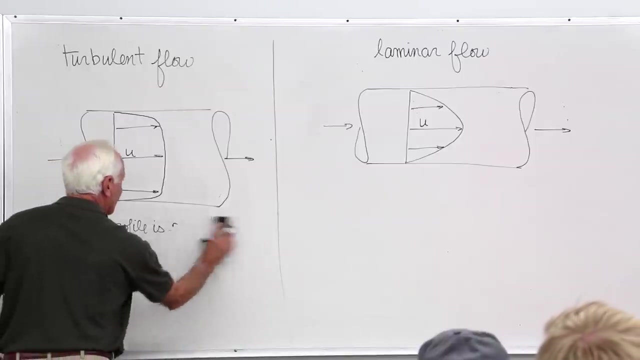 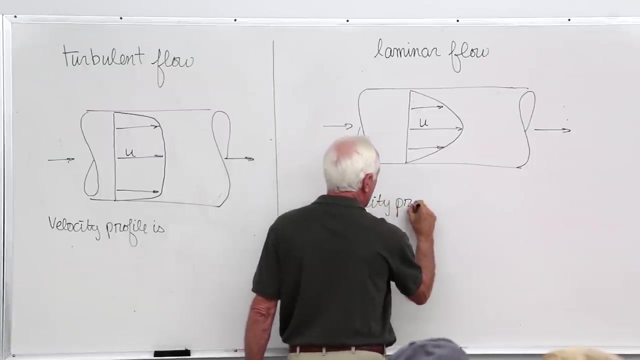 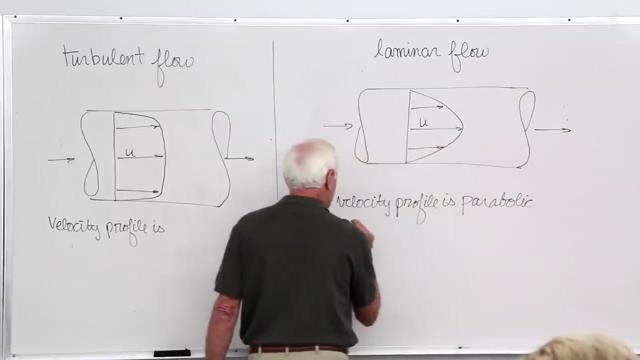 uniform, Uniform, Very nearly uniform And laminar flow. velocity profile is parabolic, The velocity u over the maximum velocity, That's for laminar Right. Yeah, Let's just change one word, There we go. Velocity profile is parabolic And u over 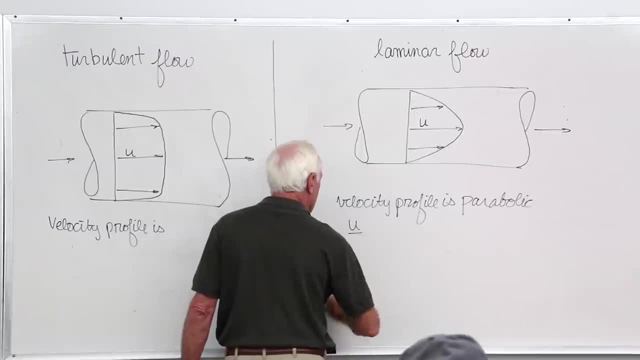 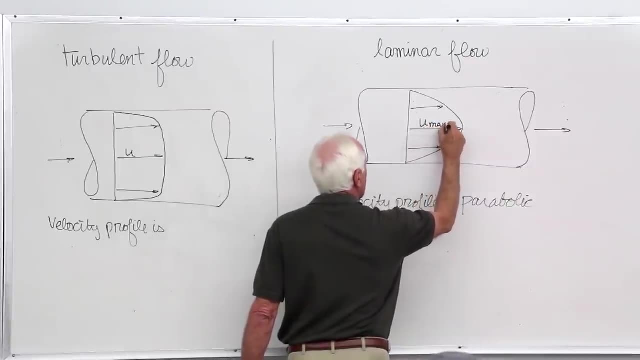 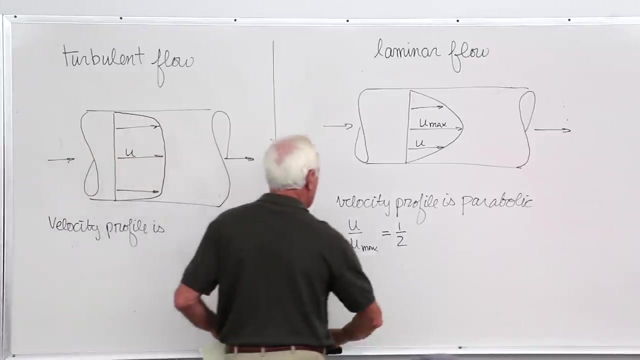 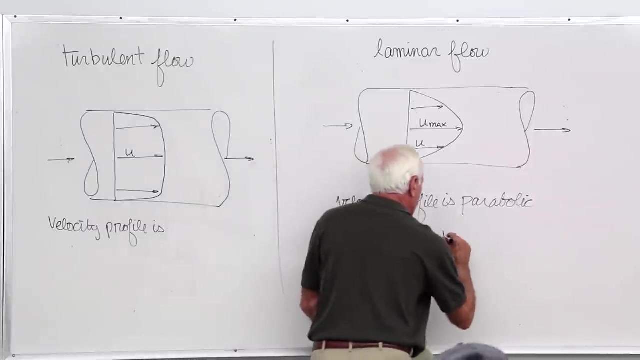 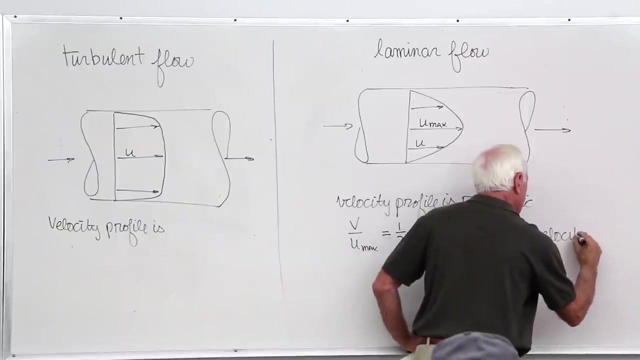 u max. Let me change my picture a little bit there so I can show that better. This is u max at the center line Right And u is the velocity at any radius. r- Okay, U over u max then is equal to one-half. So the velocity at the center line is one-half of the average. Let's make this the average. Call it capital V A little u depends on r, but capital V is the average. 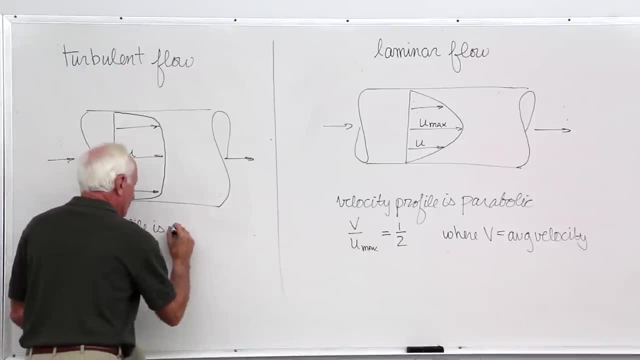 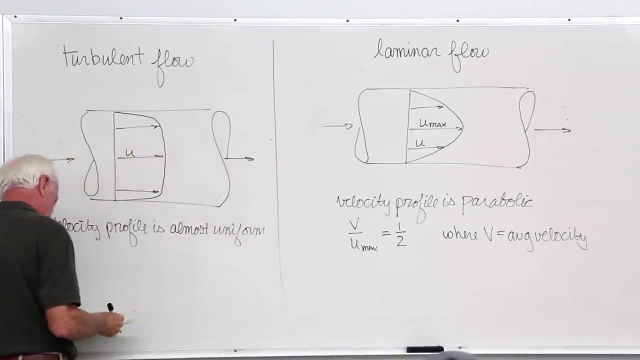 Okay, It's almost uniform, Very near to the surface. here, Left side is the right off- șq- and left side is the left side Right. This is what we're looking for. It's almost uniform. So the center is almost uniform. 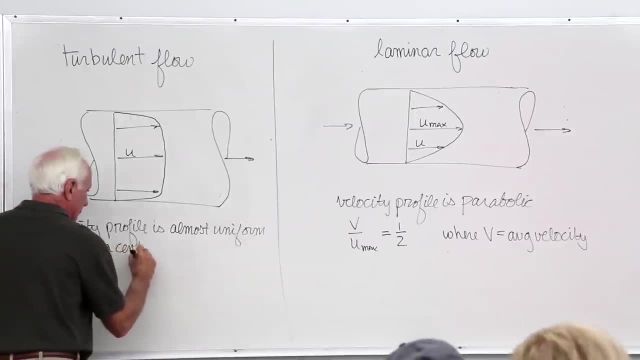 We're looking for that standard r Here. We're looking for that standard r Right The center here. velocity profile: it's almost uniform Over the central region of flow. Here It's very steep near the walls. Now here's the flow. 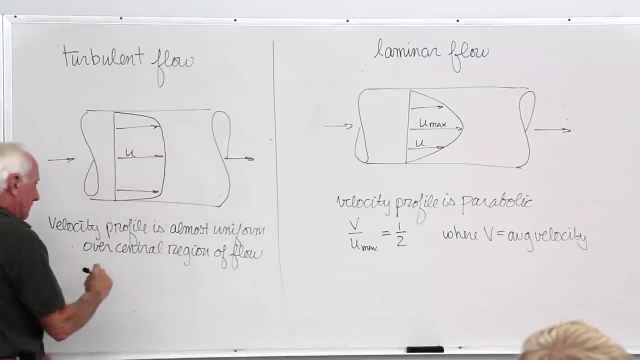 So it looks like, You see, There's just a little bit of a quarter. There's a little bit of a quarter down here. The wall is flat, here The floor, this wall is flat, So the flow gets quite steep. It's a very steep near the walls. 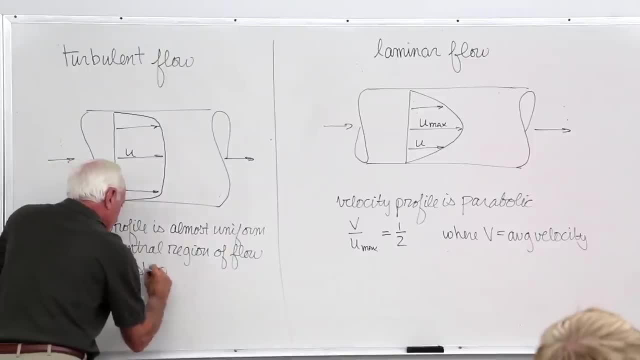 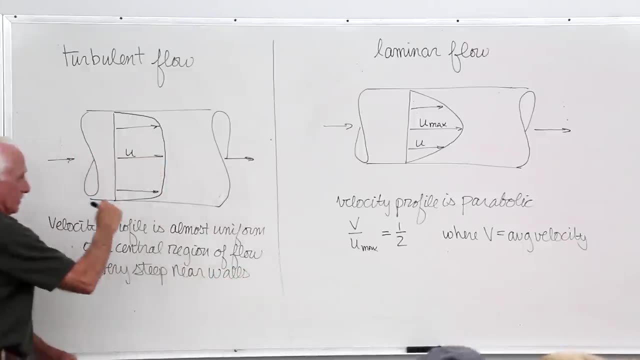 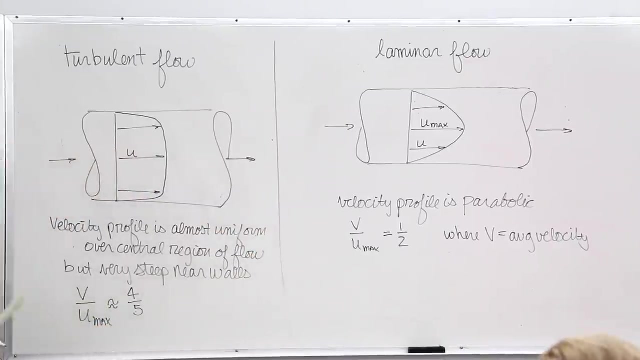 Very steep change in velocity of the balls. In this case, the average velocity divided by the maximum velocity is somewhere around four fifths. It depends on a couple things that are a little more complicated, but roughly four fifths. This guy over here is one and a half. 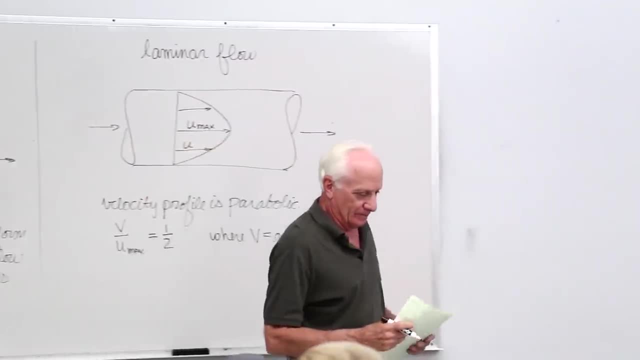 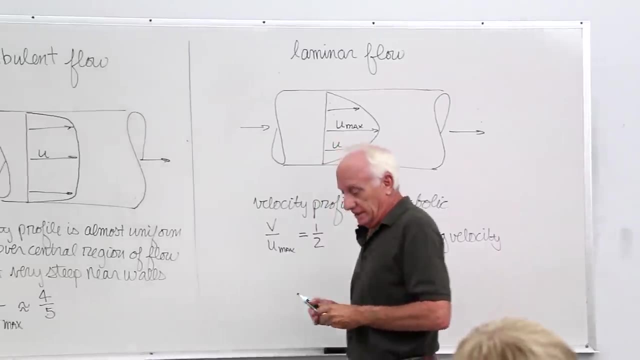 We can get an idea of which one has the greater shear stress. The shear stress is proportional to the velocity gradient at the wall and the velocity gradient in turbulence. So we can get an idea of that. The shear stress is proportional to the velocity gradient at the wall and the velocity gradient. 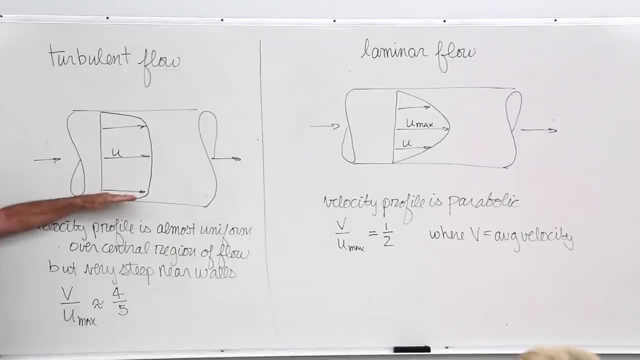 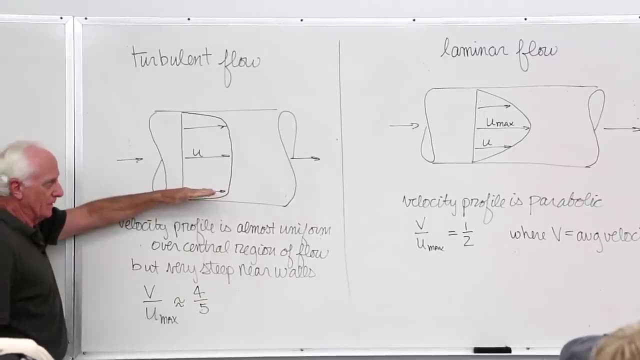 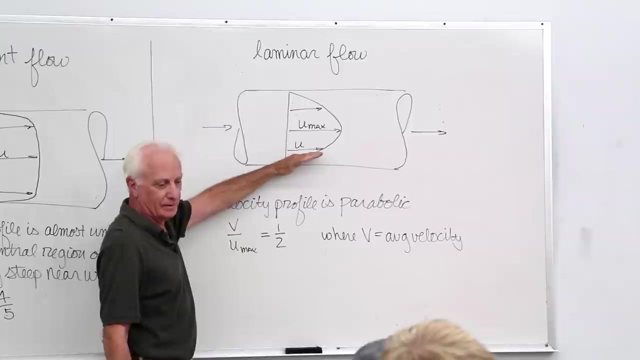 in turbulence. Turbulent flow is very steep. There's a big change in U with respect to radius. Big change. The UDR is a big number. That means the shear stress is very big In laminar flow. there's a smaller change in U with respect to R at the wall. 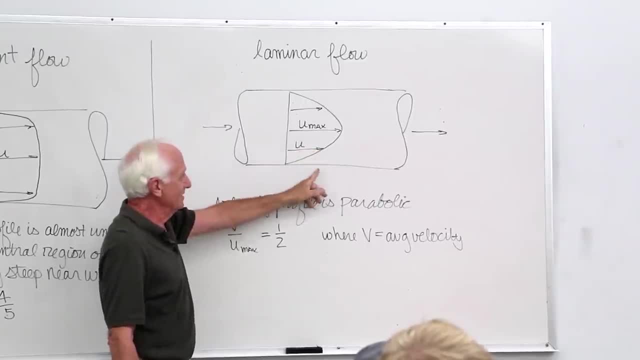 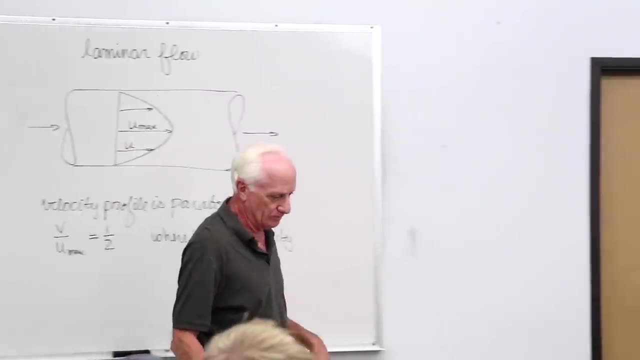 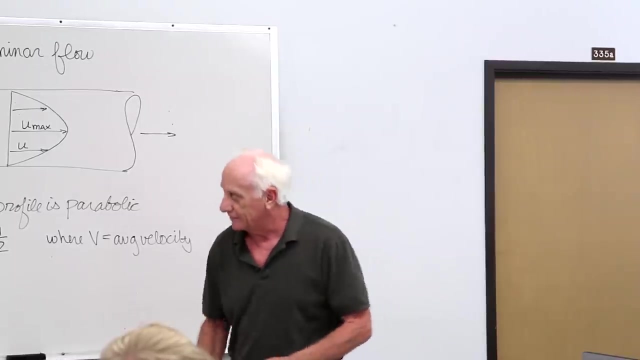 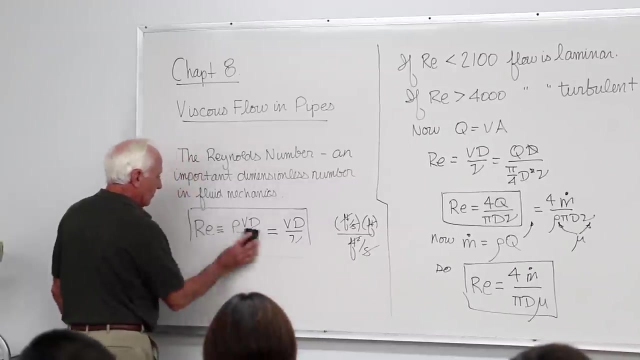 Tau equal U DU DR. Okay, This guy has a smaller shear stress. This guy has a bigger shear stress. That's one of the things that happens with turbulent flow. Okay, now the next thing is looking at what happens when flow enters along the pipeline. 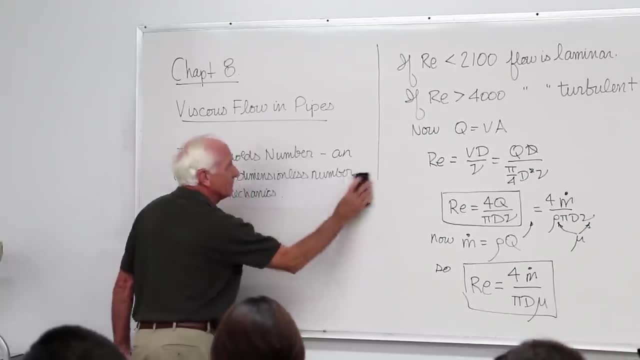 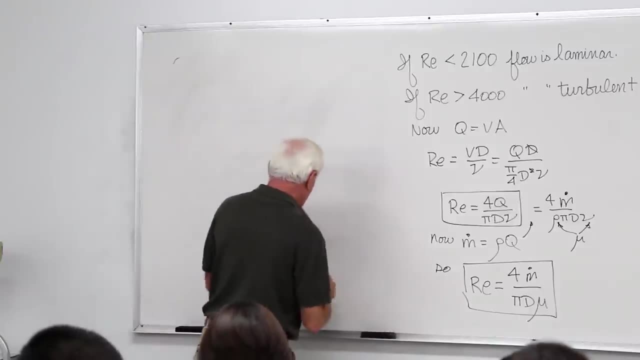 So from the reservoir. So let's look at that. It's called the entrance effect, So I'll make a sketch of what's going on. The flow then is entering from a large reservoir where the velocity is assumed to be zero. And then the flow is entering from a large reservoir. 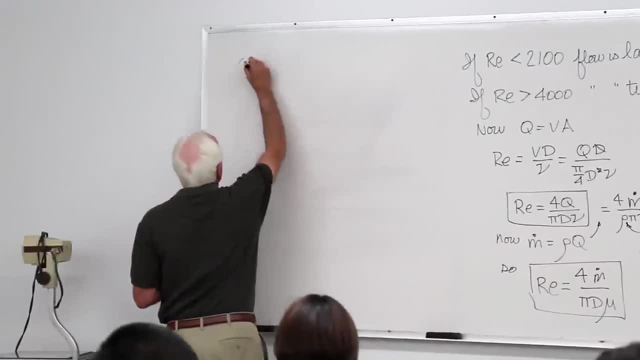 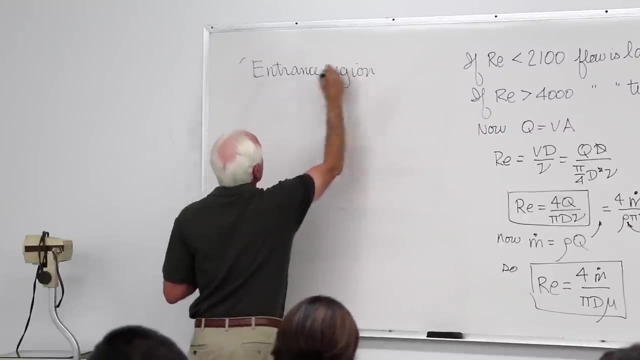 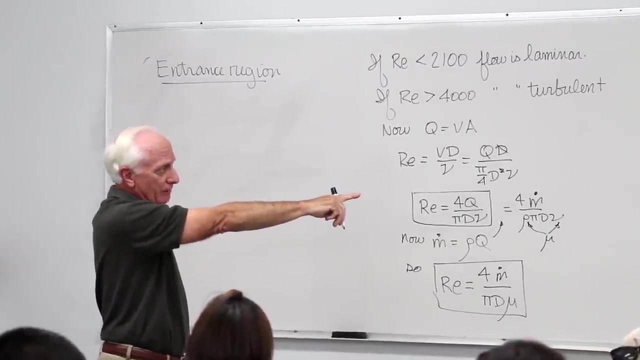 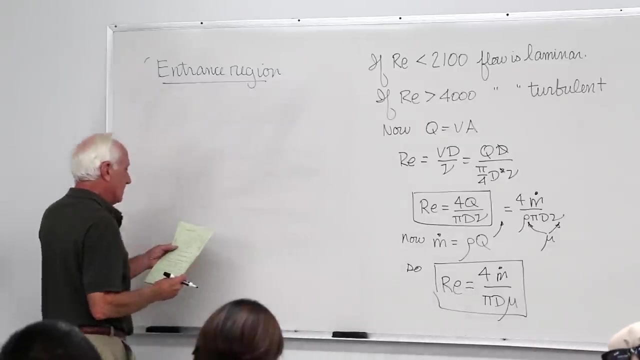 And then the flow is entering from a large reservoir. So see that zero. By the way, we'll prove for parallel flow that. We'll prove that in about 20 minutes. So you'll see where that comes from The entrance regions. 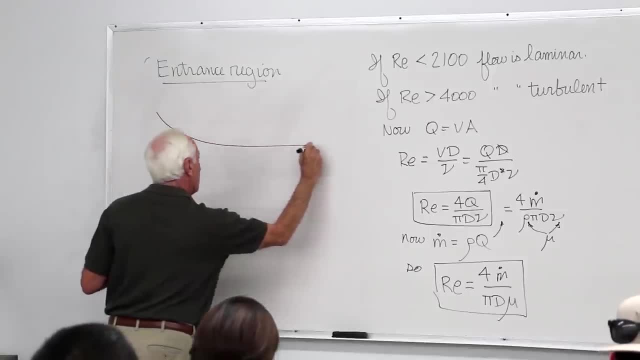 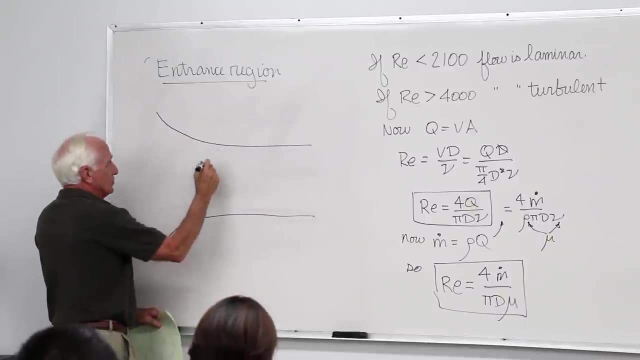 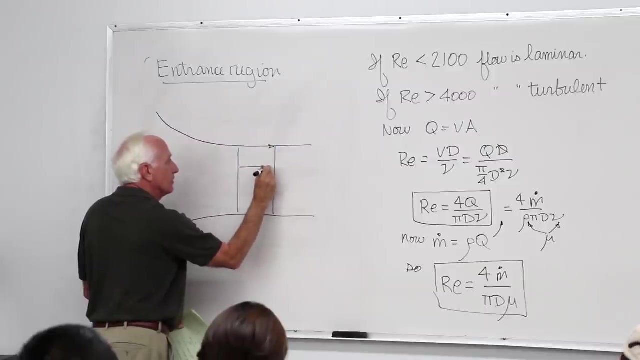 So here the flow enters from a large reservoir and then from a large reservoir, a large reservoir. We're going to assume that the flow comes in with a uniform velocity profile. So it looks like this Again: what's a velocity profile mean? 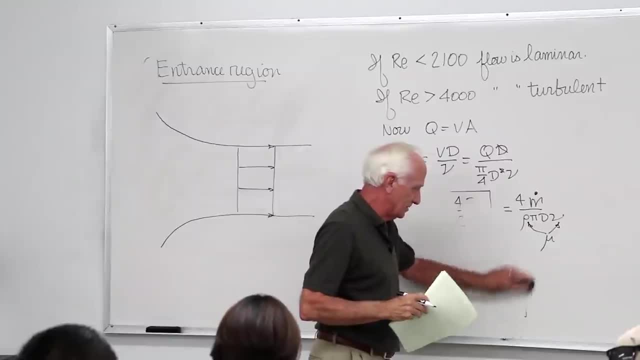 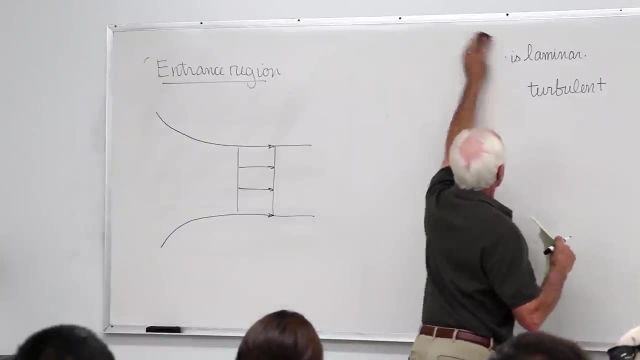 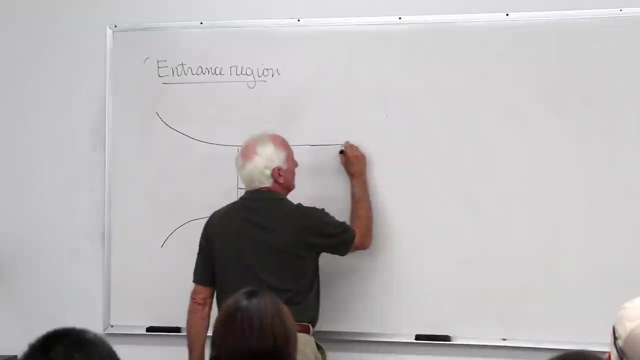 It means the velocity as a function of some coordinate distance: x, y, z, radius. That's called a velocity profile. When the flow comes in we assume it's uniform. When it gets down here further, it starts to look more like this At the wall: the 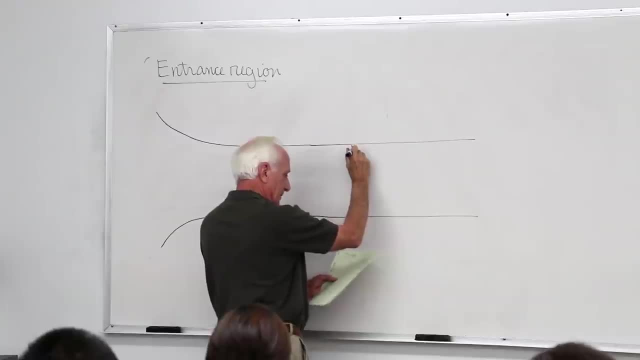 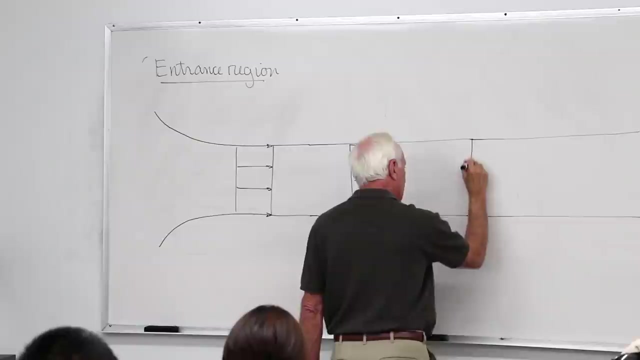 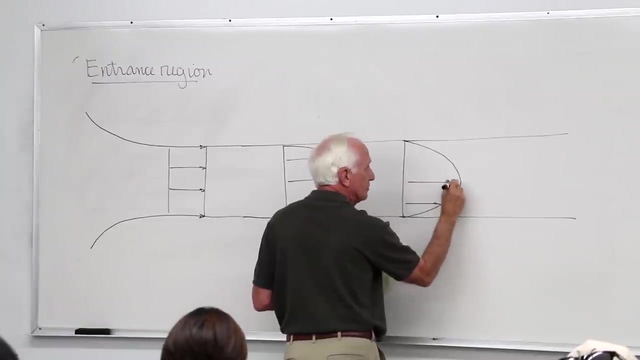 wall starts to slow it down. so it looks something like this: And you go further down and it looks something like this until finally it gets to be parabolic. If it's laminar flow, We're going to assume this is for laminar flow. And if you go, 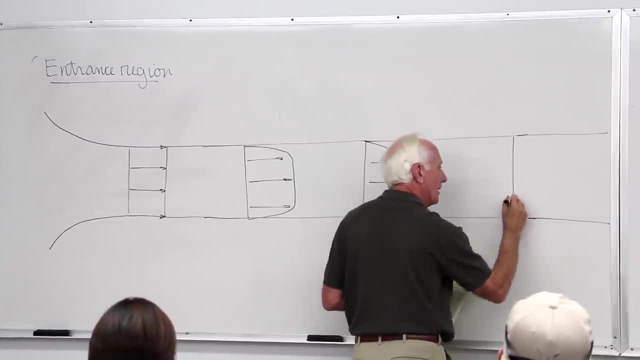 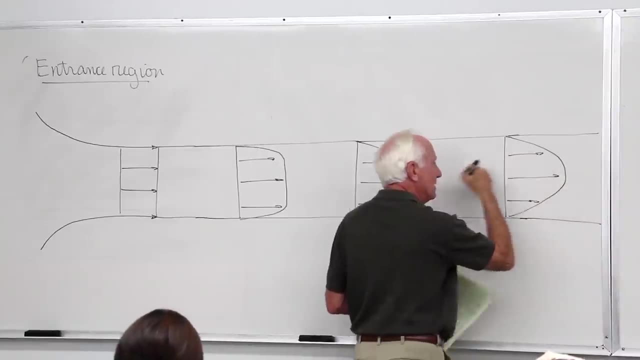 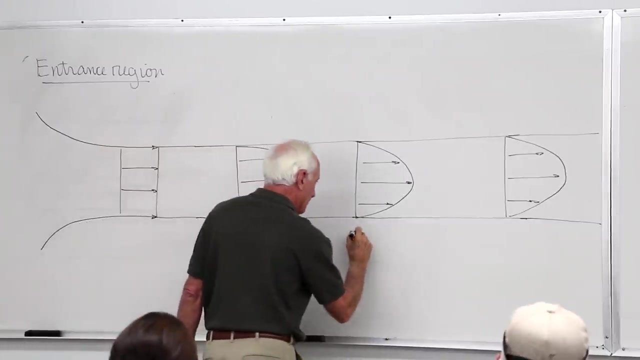 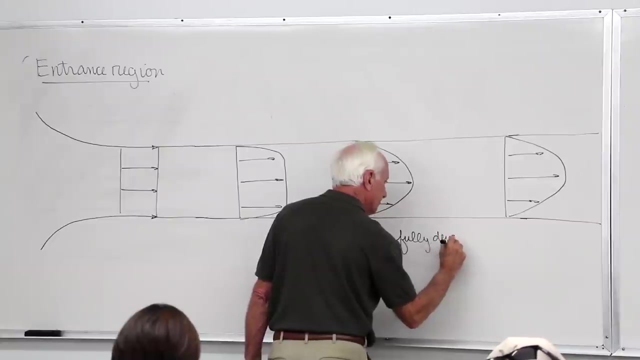 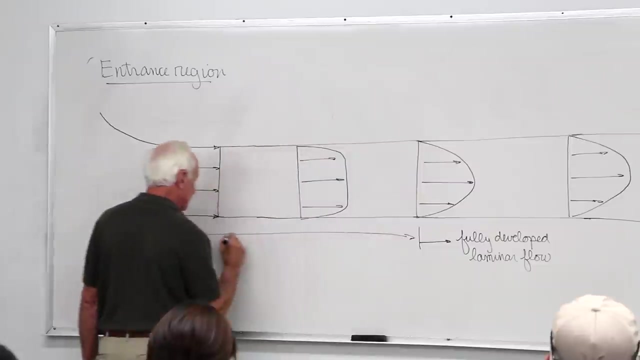 further down it stays parabolic. Once it reaches that parabolic shape, we call that fully developed flow. So from this point on down it's fully developed laminar flow. This region from the entrance here is called, of course, the entrance region. 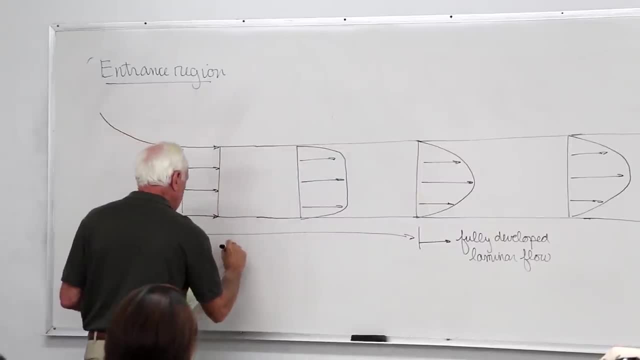 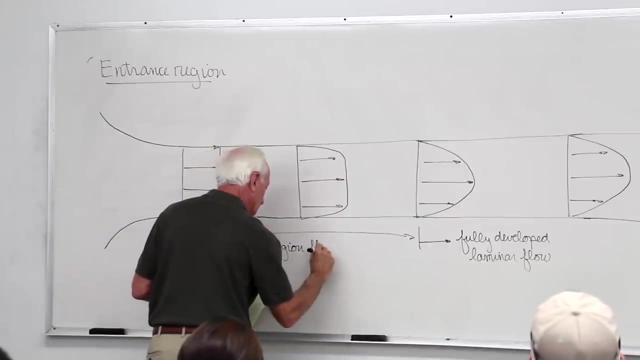 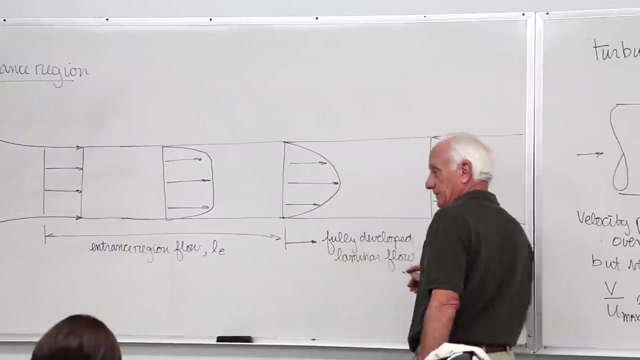 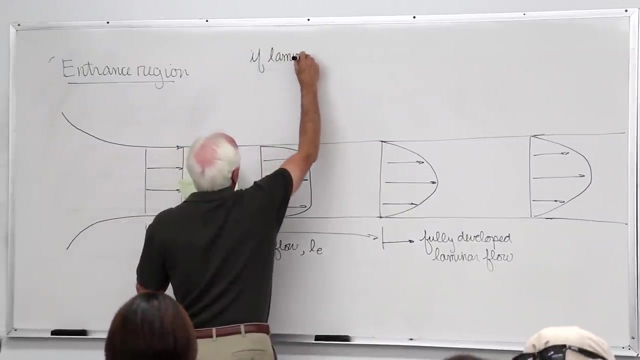 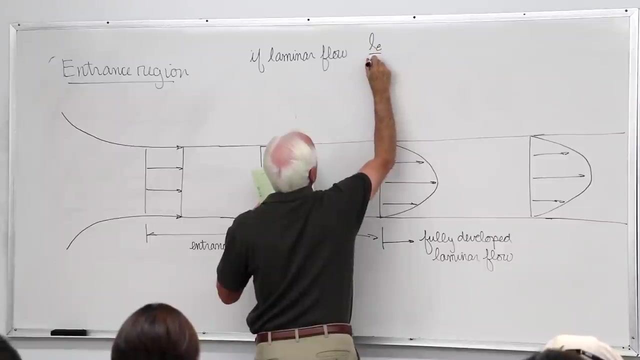 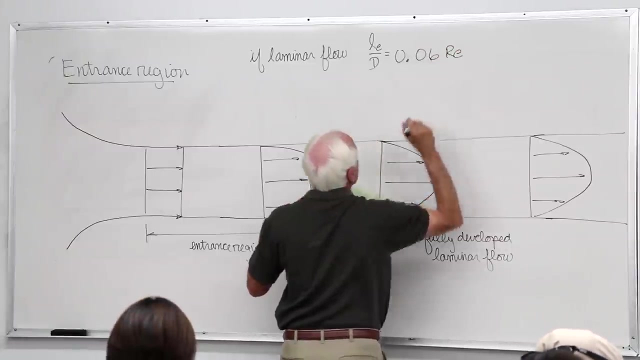 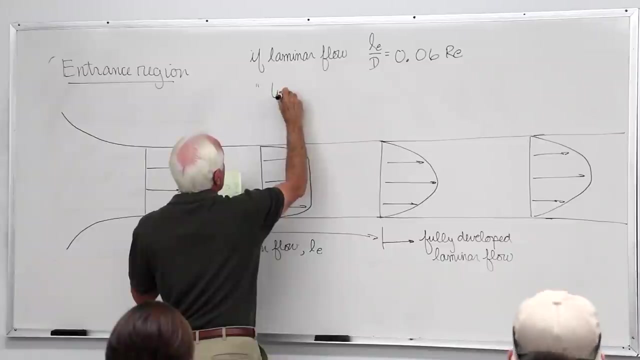 Up here And this distance is given by L, sub e. It stands for entrance alpha length. Now, if it's laminar flow, then the entrance region L e over d, 0.06 times the Reynolds number. If it's turbulent, 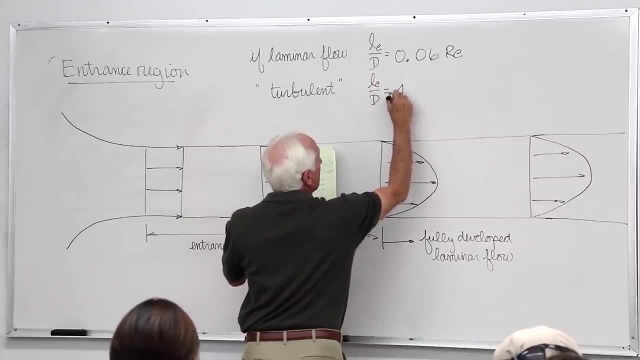 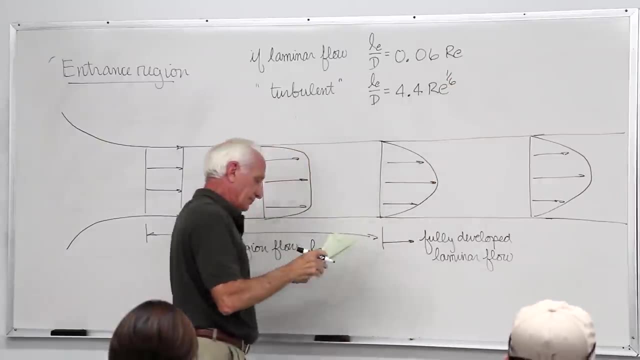 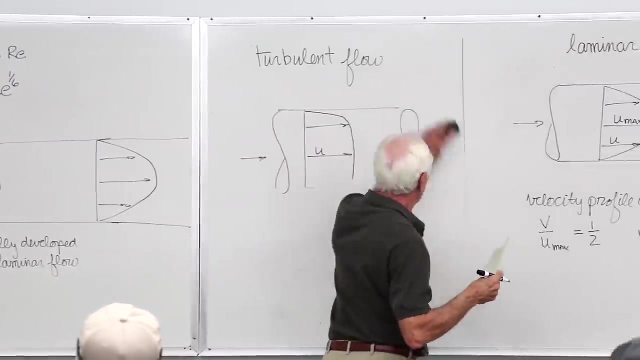 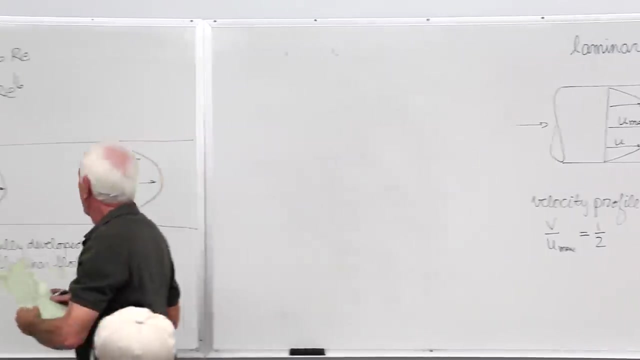 L e over d. these are in your textbook. 4.4 Reynolds to the 1.6.. Where's the d? d is the pipe diameter. Yeah, d is the pipe diameter. Thanks, but yeah, we'll mention that. 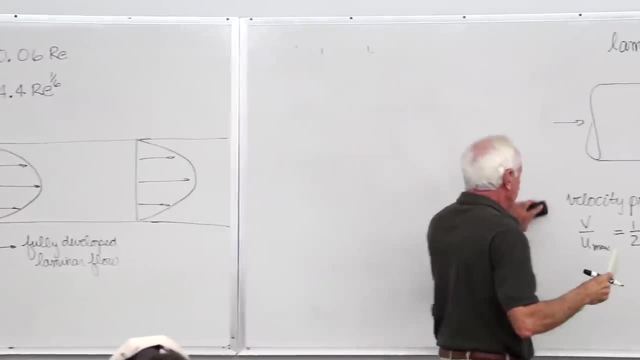 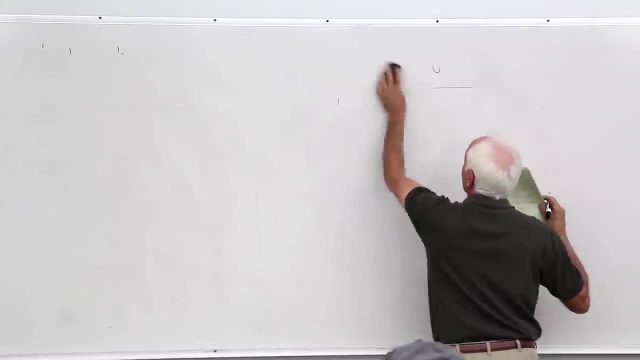 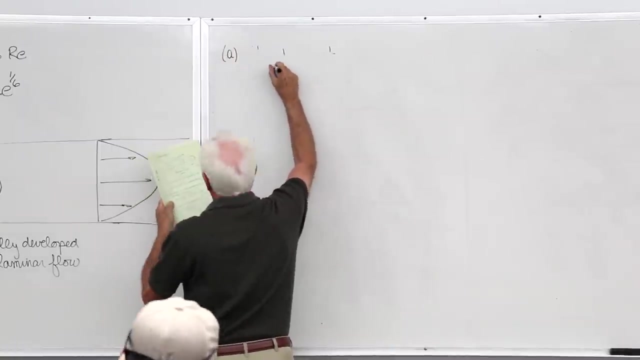 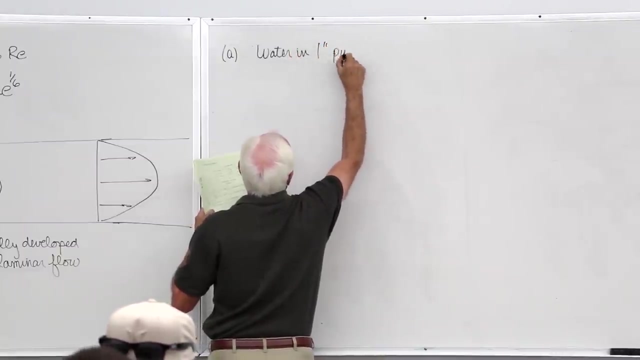 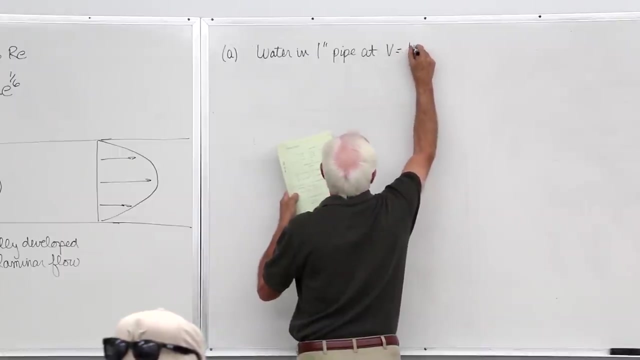 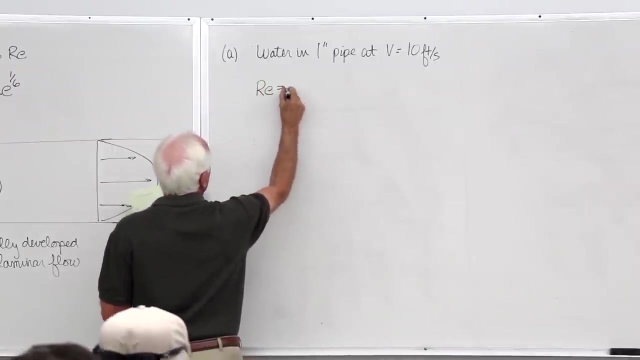 Good, Okay, now How we use this. Okay, Let's take an example of how we use this. Let's take, in this case, a water in a one-inch pipe at an average velocity of 10 feet per second. Okay, water. Reynolds number. 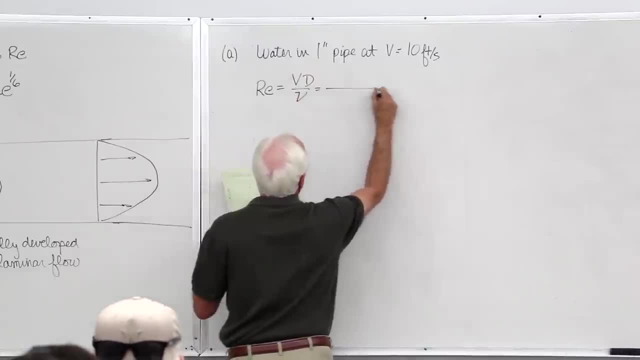 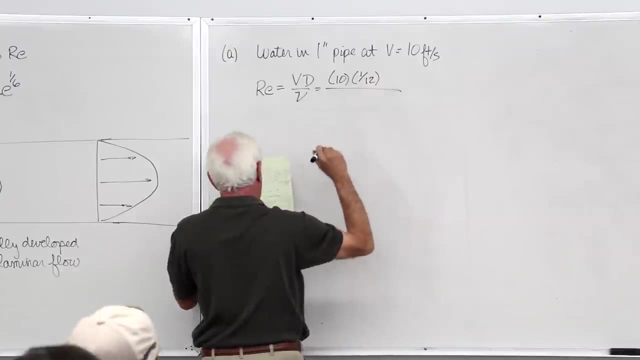 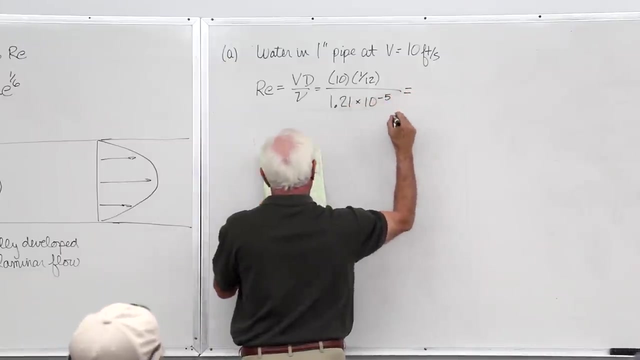 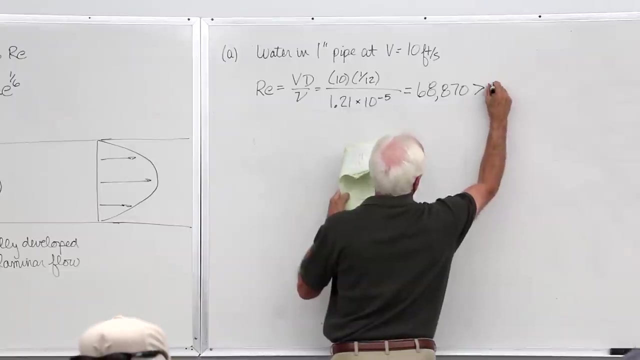 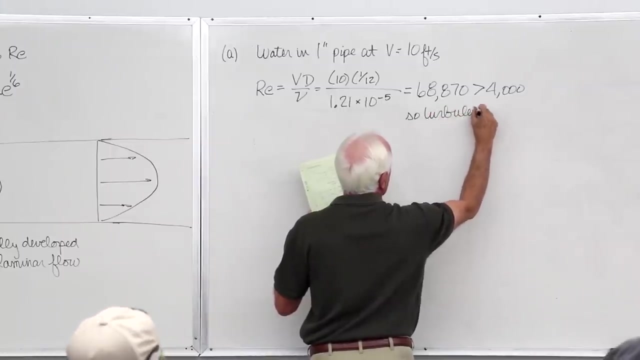 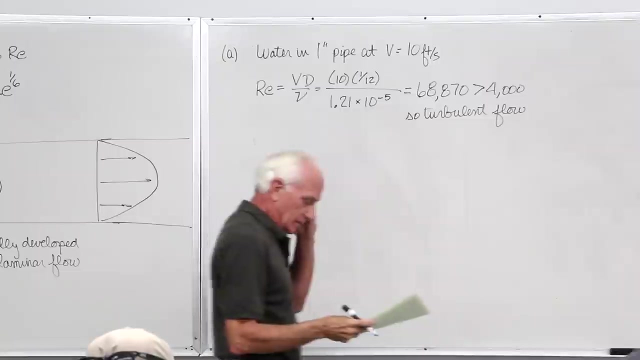 Vd over nu Kinnamac, Wisconsin. inside front cover Reynolds, number 68,870.. Greater than 4,000.. So turbulent flow, Turbulent flow of water in the pipe. Okay, and we're asked to find the entry length, L, sub e. 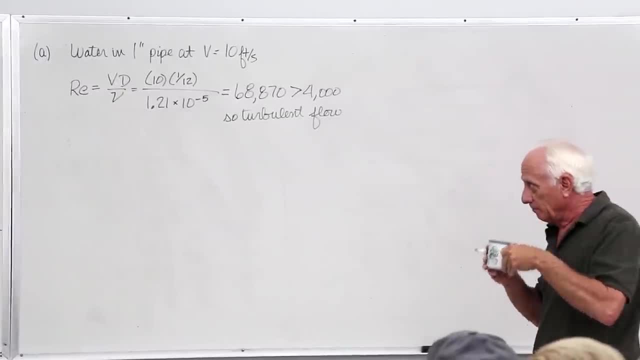 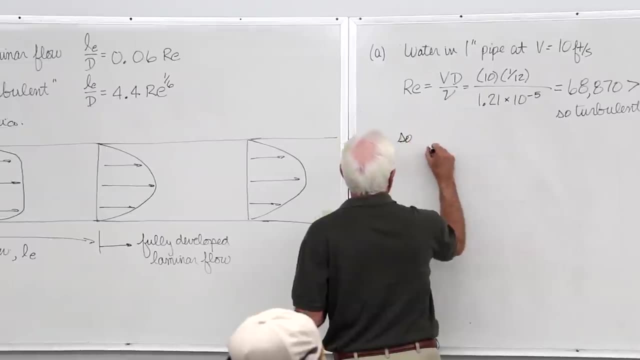 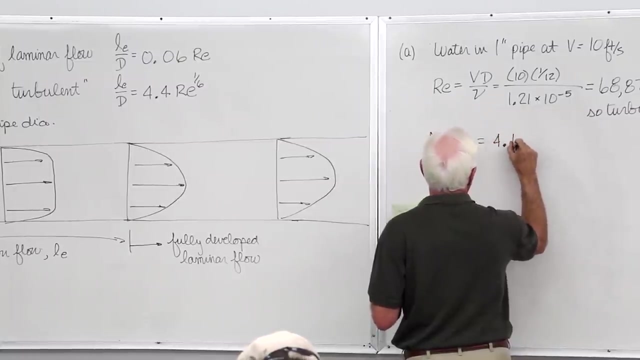 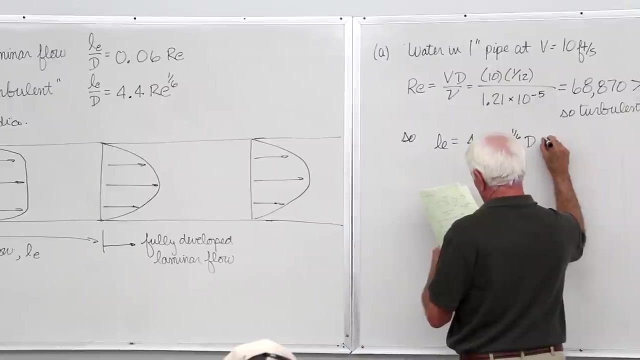 1.3. 1-inch pipe length, L sub e. there's the equation over there: Turbulent flow L sub e equal 4.4. Reynolds number to the 1.6. Times the pipe diameter. And let's see: 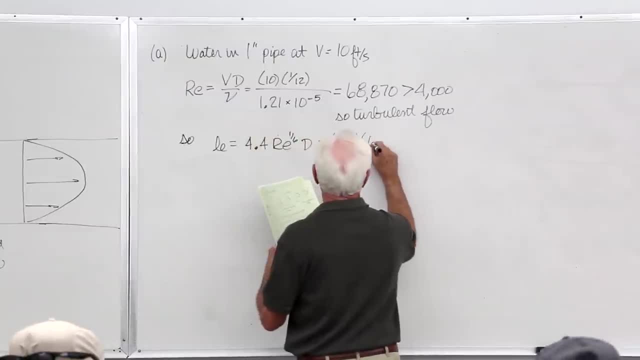 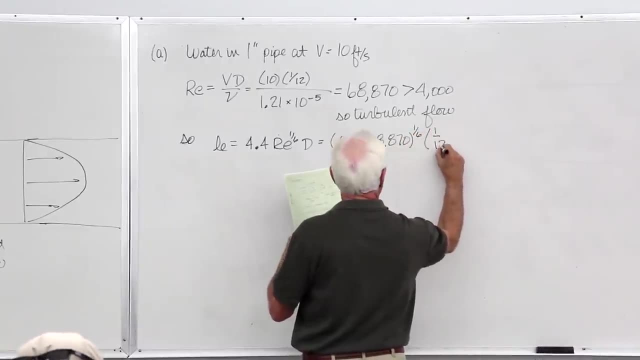 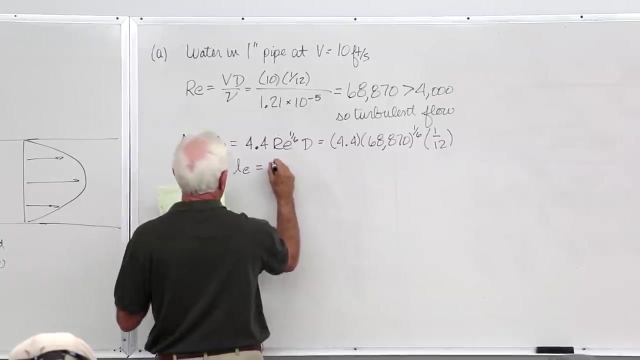 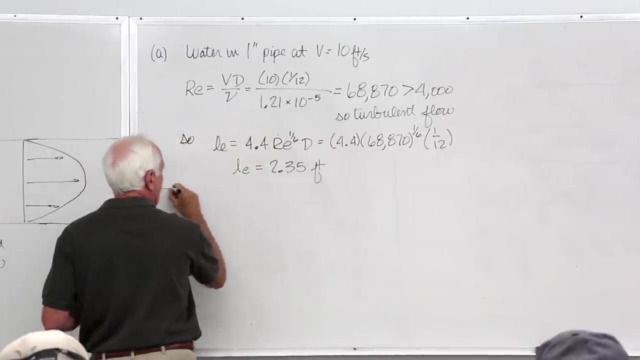 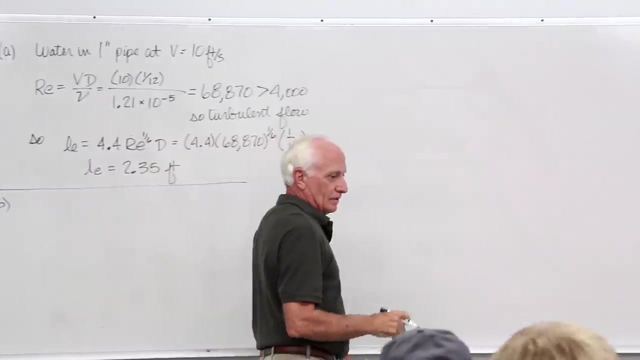 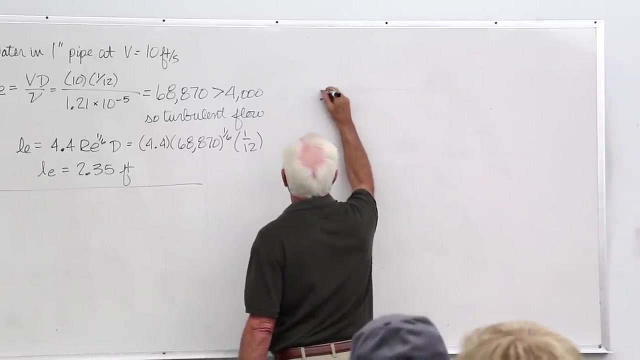 4.4. 68,870.. To the 1.6. Times: 1.12.. L sub e is equal to 2.35 feet. That's about a one-inch pipe right there. Backyard PVC sprinkler pipe. 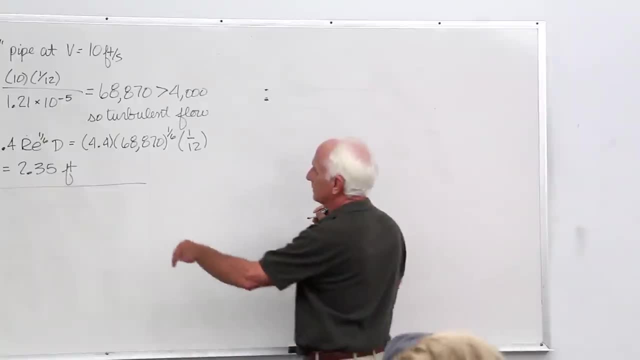 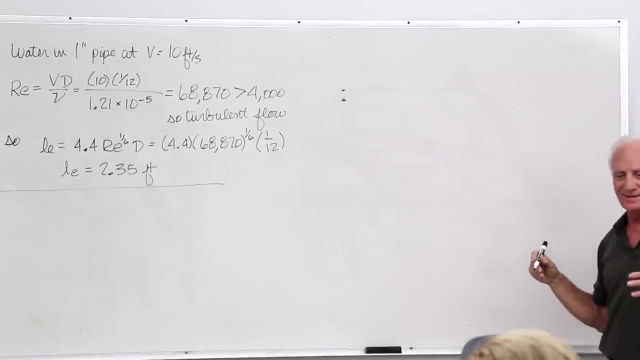 Where people are loading behind one inch. That's a typical velocity, 10 feet per second in a pipe. Most of the time water in pipes is turbulent. It takes a really, really slow flow to get laminar flow in a pipe of water. 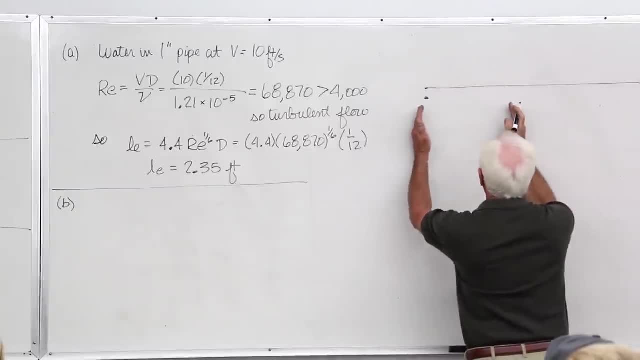 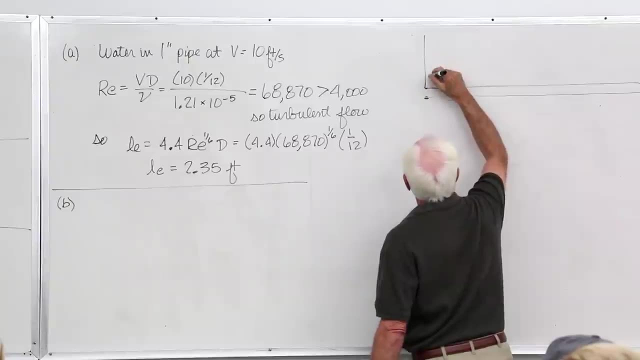 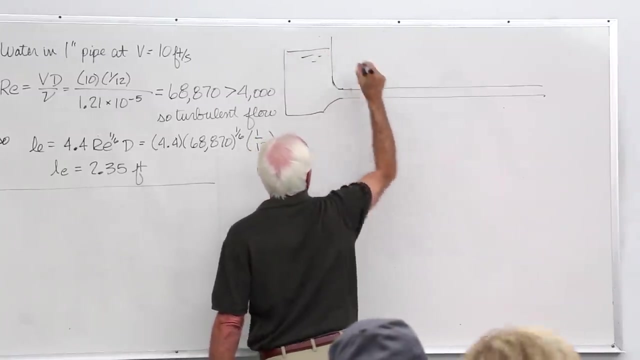 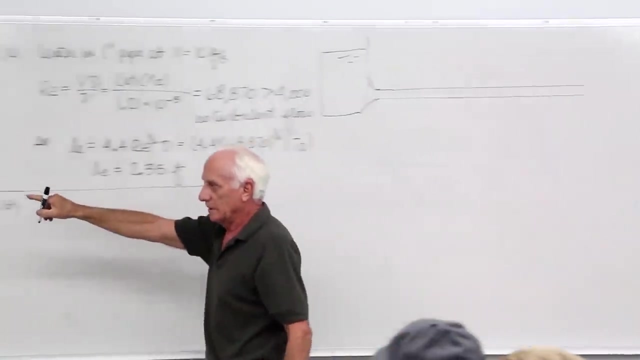 Two and a half feet. 12 feet, 12 feet and a half, That's about right. So if water comes in from a reservoir here, it takes that long for a one-inch pipe, with 10 feet per second. When it gets down here, it looks like this: 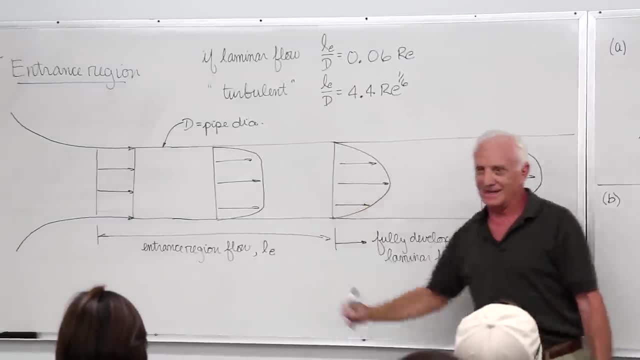 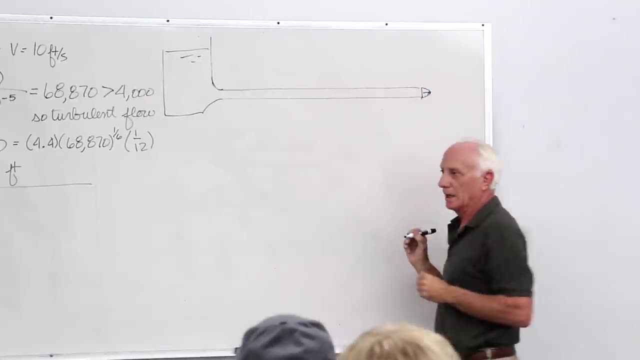 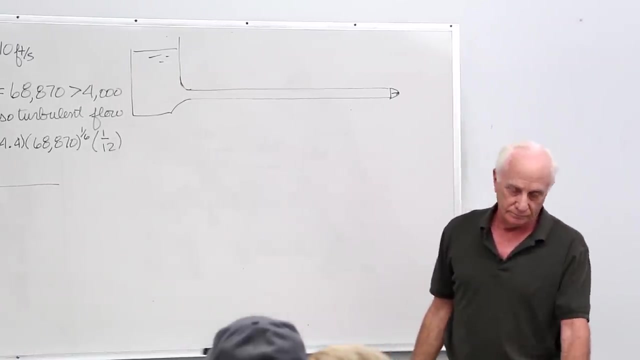 A parabolic shape. Before that it looks like this: A developing flow. It takes this long before that velocity profile shape is parabolic. It takes a while. It takes a while for water, Professor, Come on. So this is. this is turbulent flow. 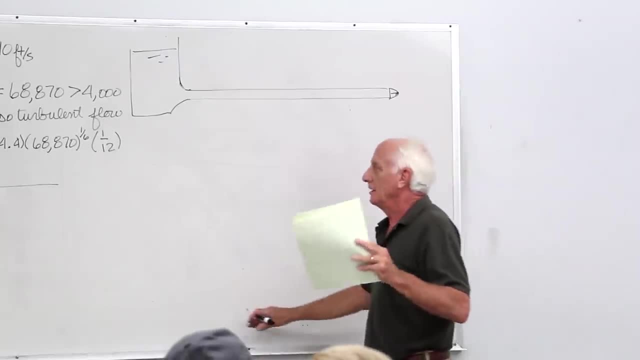 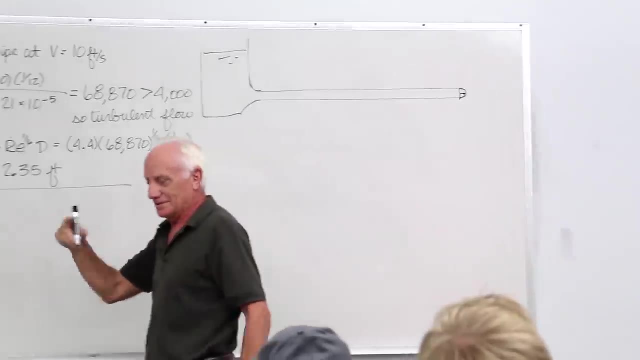 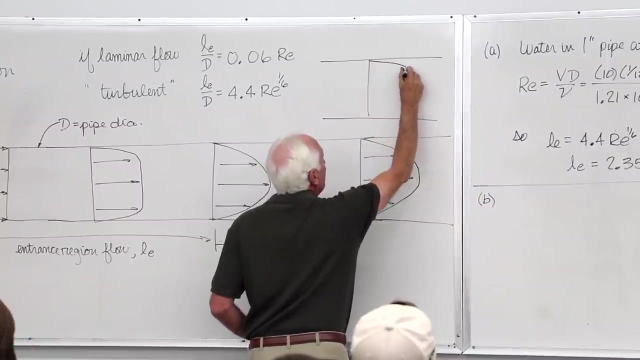 But it looks like that, Oh, okay. No, It looks like flat, Fully developed, turbulent. If it's turbulent, good question. If it's turbulent, it won't look like this. at that point, It'll look like this And it won't change anything. 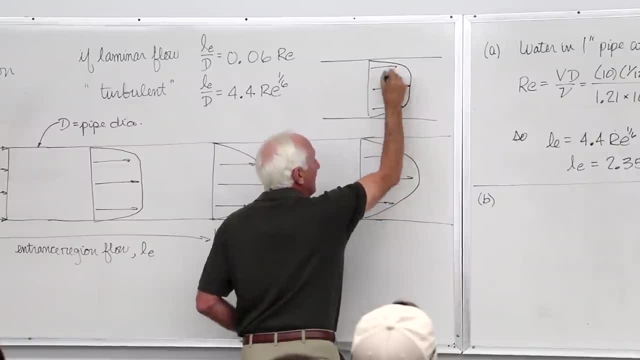 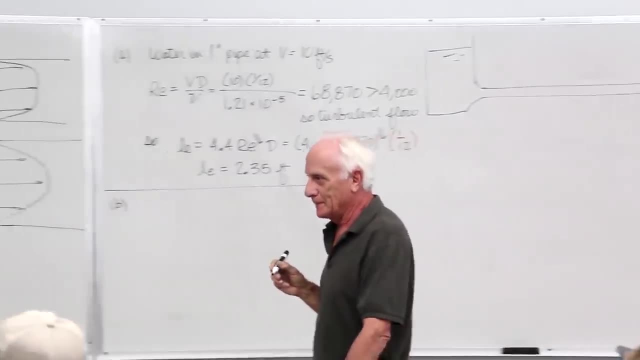 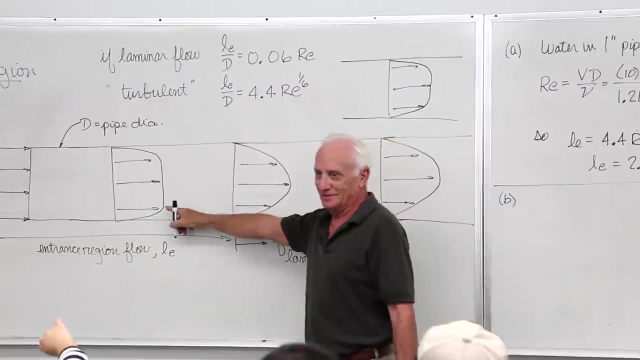 It won't change anything anymore. Yeah, good point. So the momentum flow transforms to that, to that, So it also passes through that stage. No, This is not turbulent. This is not a turbulent flow. Yeah, but that's the momentum. 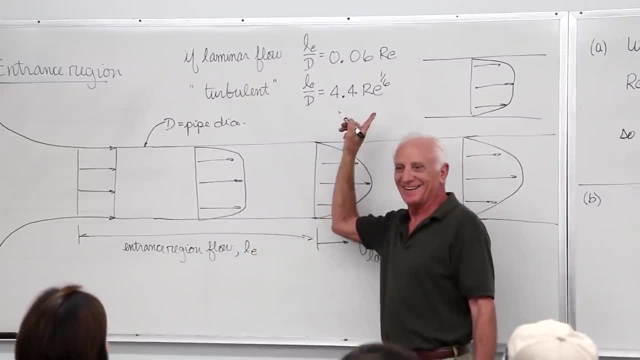 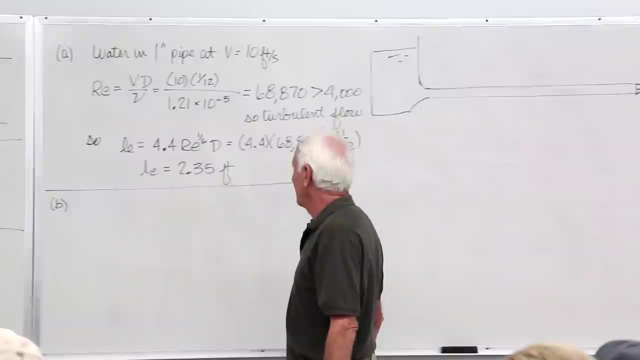 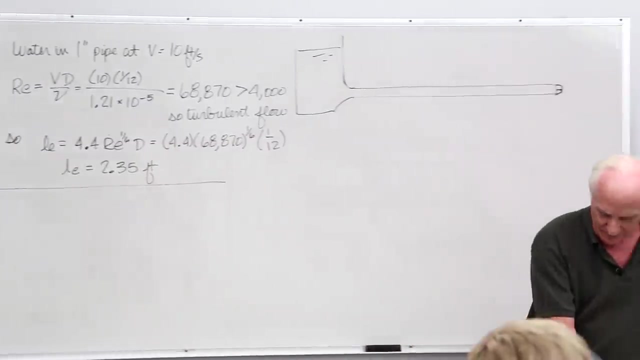 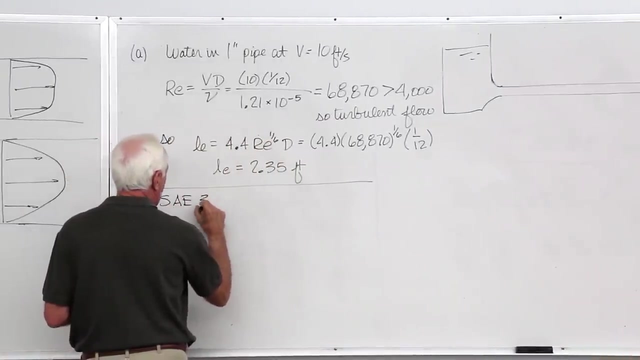 But it also passes through. Yeah, yeah, It looked like this before it gets to that. It just finally gets that final shape. Yeah, Good point, Dan, Both good points. Okay, All right, Let's take case B. Case B- SAE 30 oil. 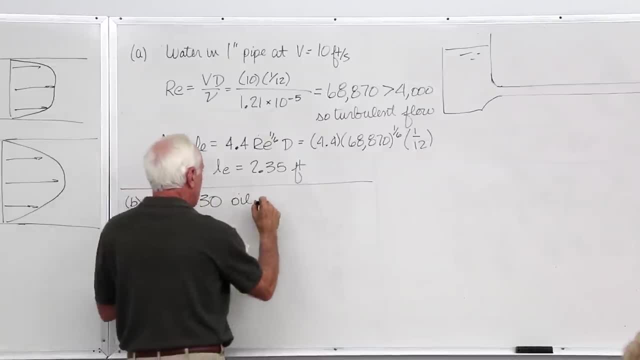 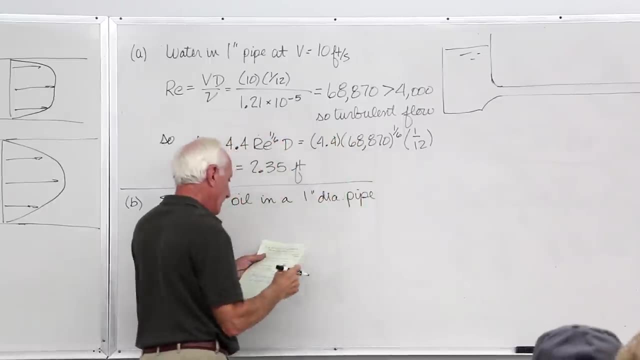 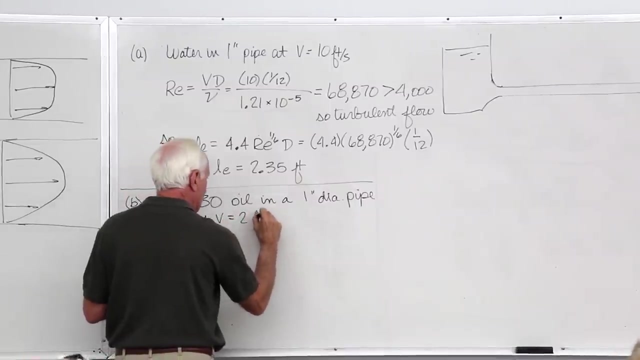 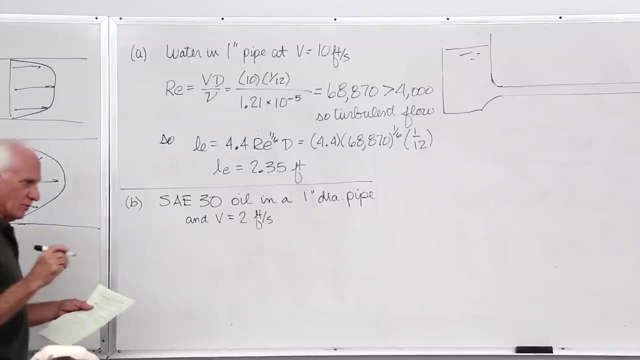 Properties are in the inside front cover of your book. In a one-inch diameter pipe, Same as the water up here. Average velocity: 2 feet per second, Typically lower for oil. Oil is hard to pump, take more pumping power, So put a little lower velocity in. 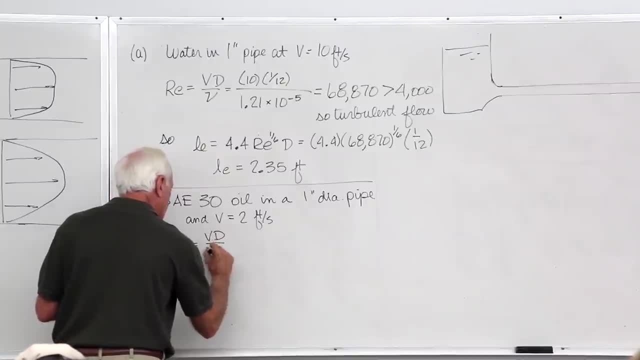 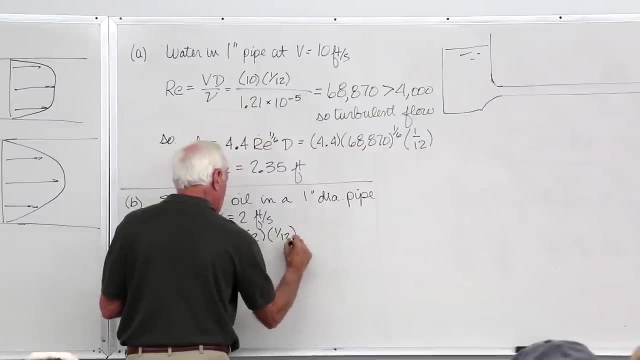 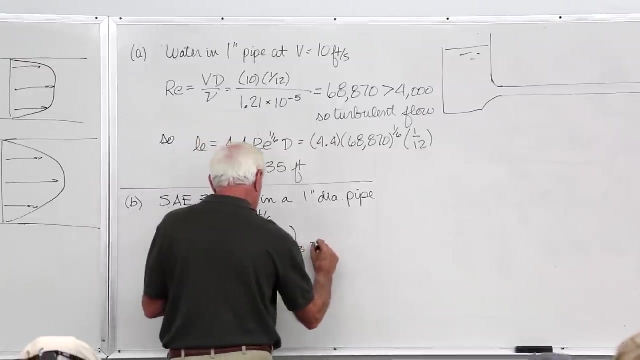 The Reynolds number VD over nu 2 for the velocity, 112 for the diameter, 4.5 times 10 to the minus 3.. 37.0.. Oh yeah, that's a lot less than 2100.. 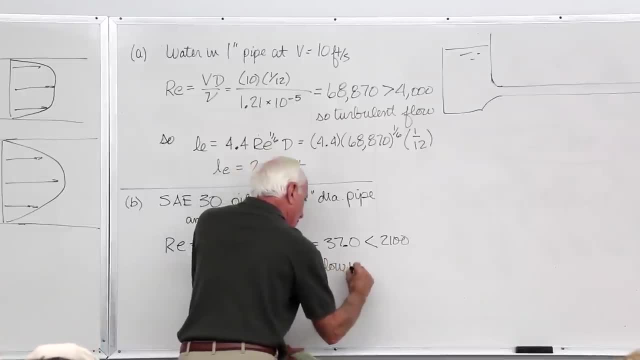 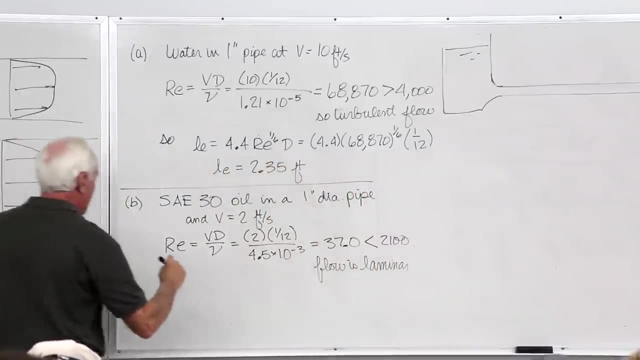 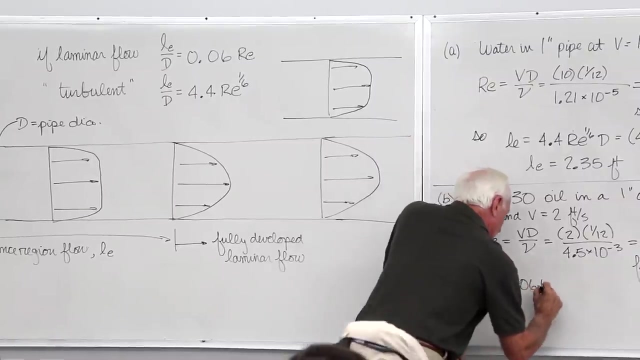 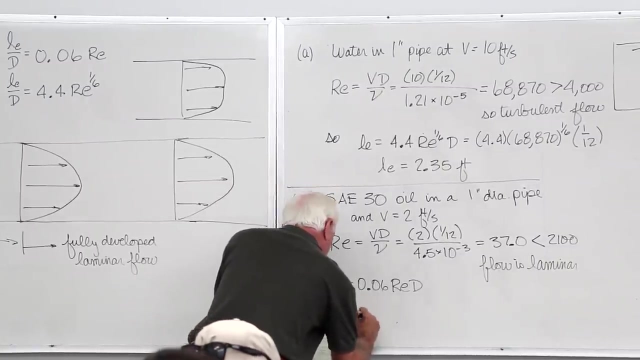 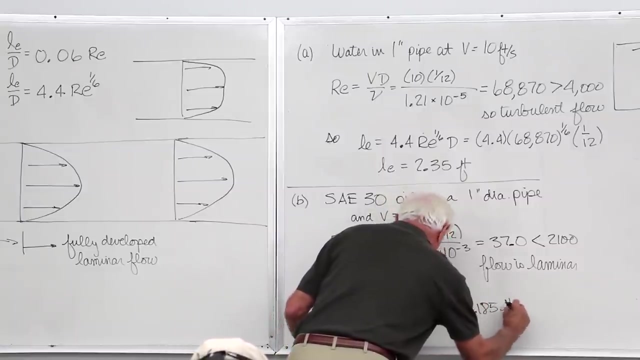 Flow is laminar, Okay, laminar L over E over D: 0.06.. Reynolds number times diameter: Okay, so we have 0.06, Reynolds number 37, diameter: 112, 0.185 feet. 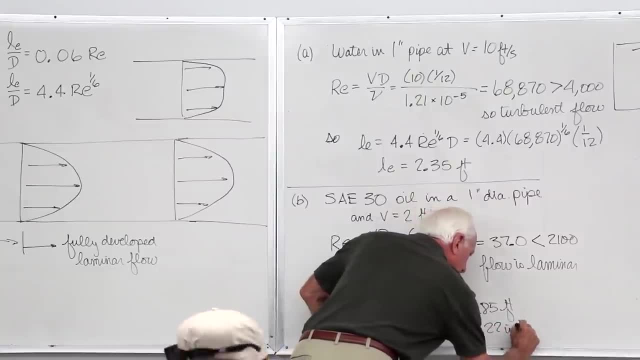 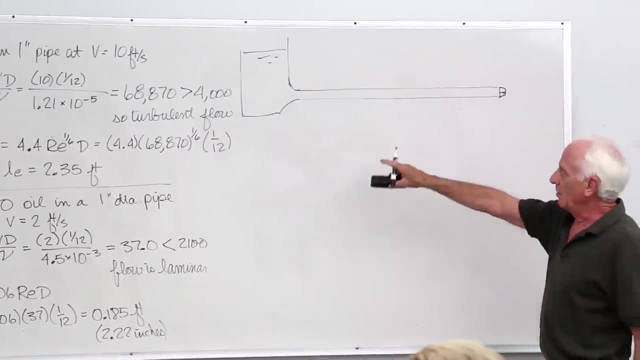 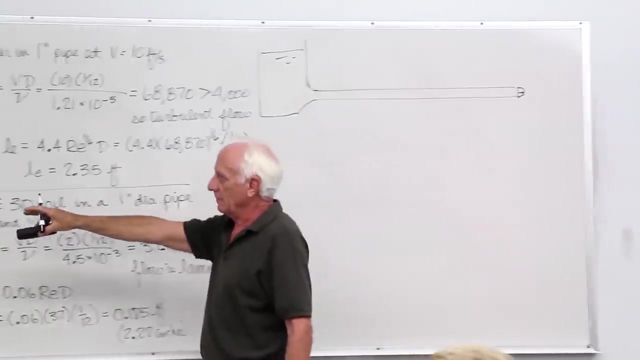 0.22 inches. So now we have turbulent. we have oil- 30-way oil- in that pipe. Same diameter, one-inch diameter pipe. Now it's carrying oil. When does it reach fully developed velocity profiles? After only 2.2 inches. 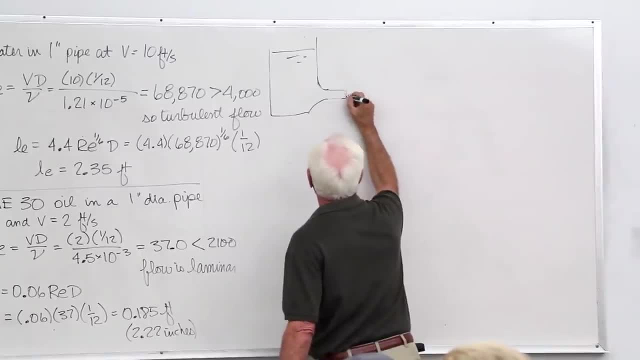 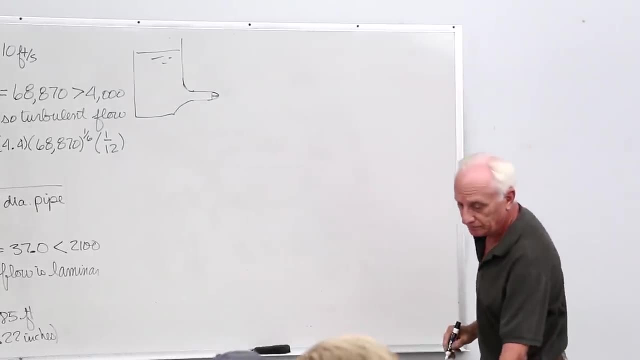 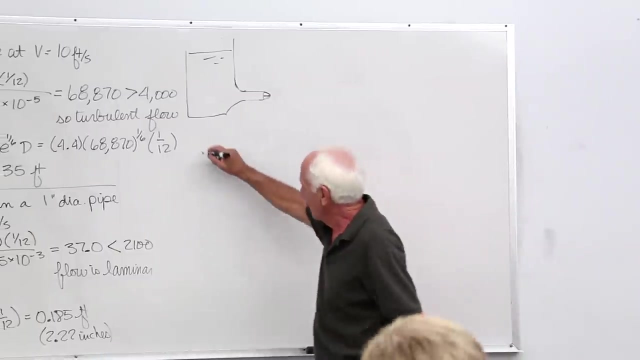 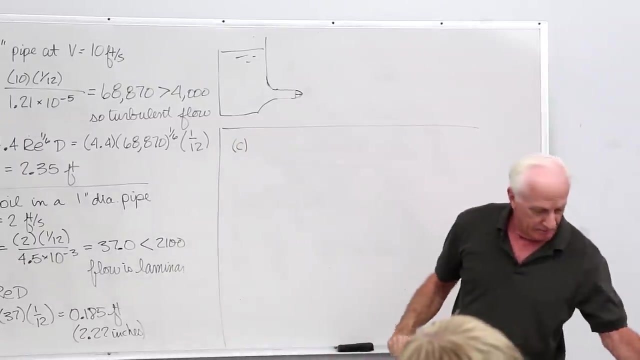 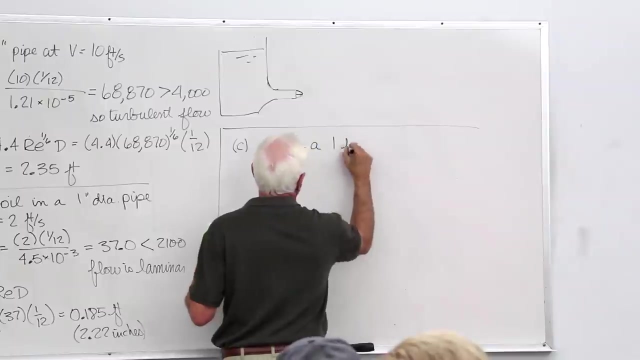 That's a one-inch pipe. That's when the oil finally reaches a parabolic velocity profile. 2.22 inches- A lot less than water. Okay, Now we have Kc Kc Air now in a circular duct. 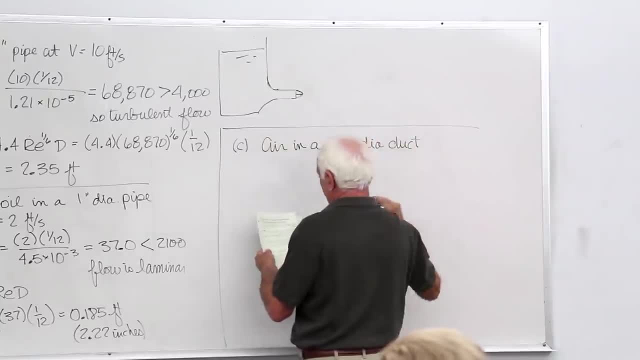 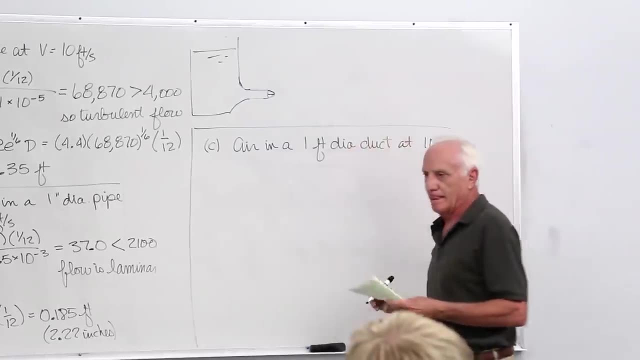 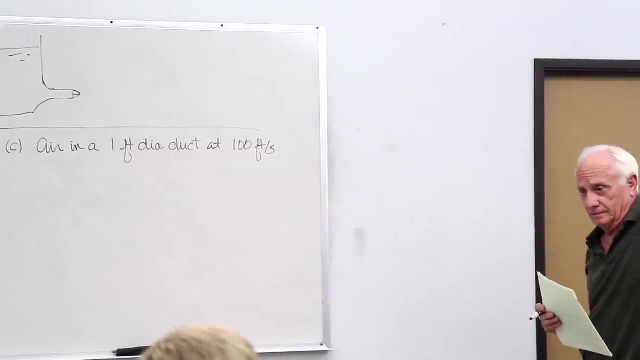 One foot down a duct At 100 feet per second- Pretty fast. but air can move pretty fast In a wind tunnel. Oh yeah, Yeah, Not up in these guys, up here in the ceiling. That's not unreasonable Reynolds number. 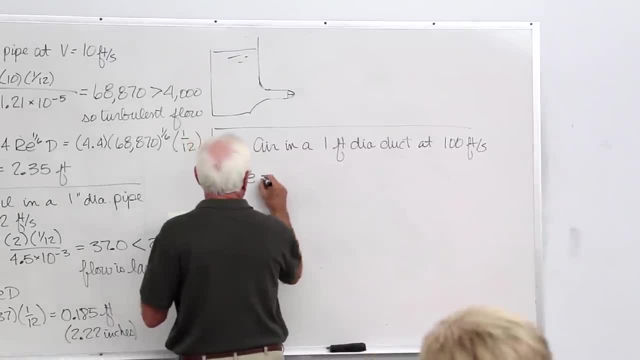 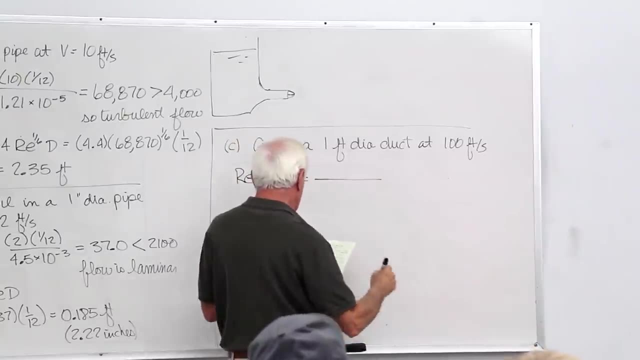 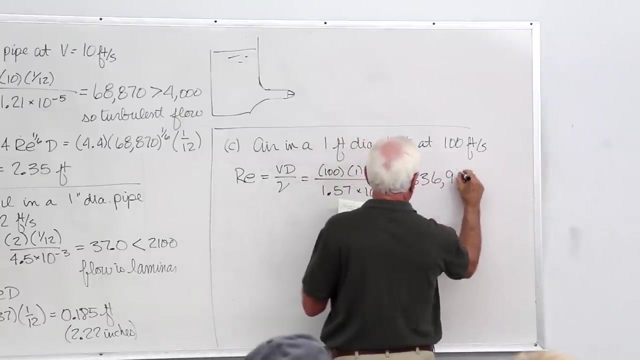 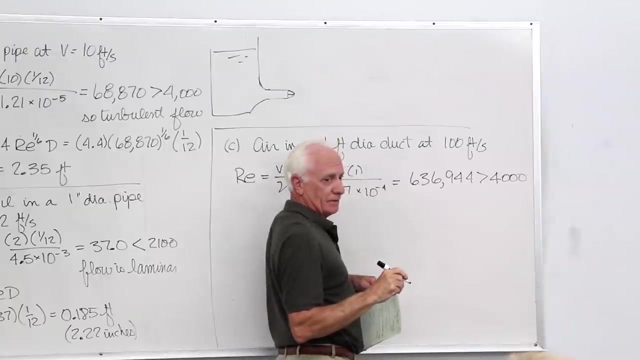 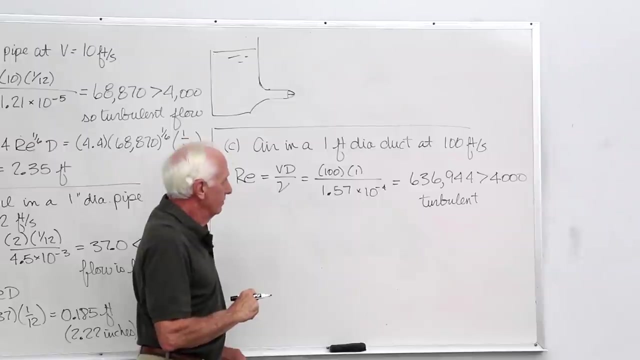 VD over nuke Inside front cover. Kinematic viscosity of air at standard temperature. Velocity 100, diameter 1,. kinematic viscosity: Oh yeah, it's really turbulent- Six times 10 to the 5th. What if air is going really slow? 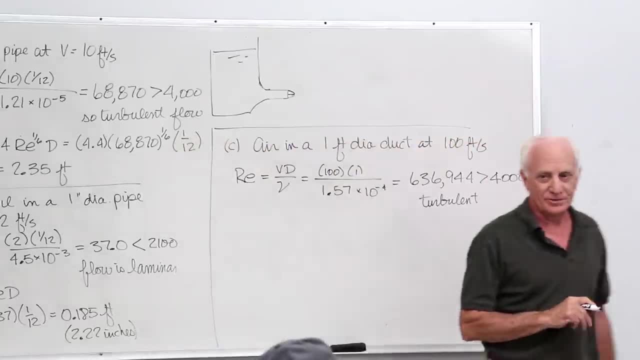 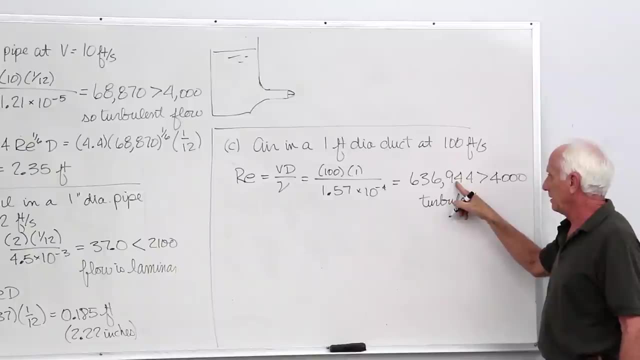 One foot per second. One foot per second is really slow. Okay, Divide this guy by 100.. Right here, 6,000.. It's still turbulent. It's almost impossible to get laminar flow. It's going to be turbulent. 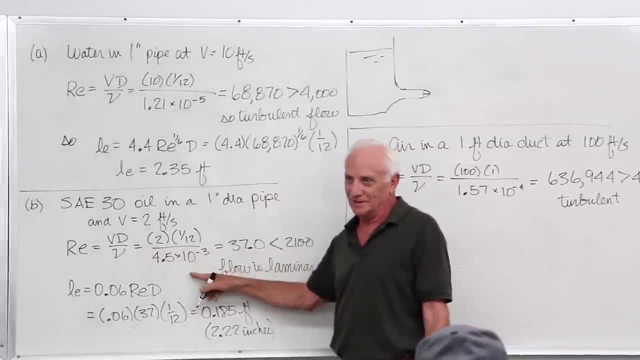 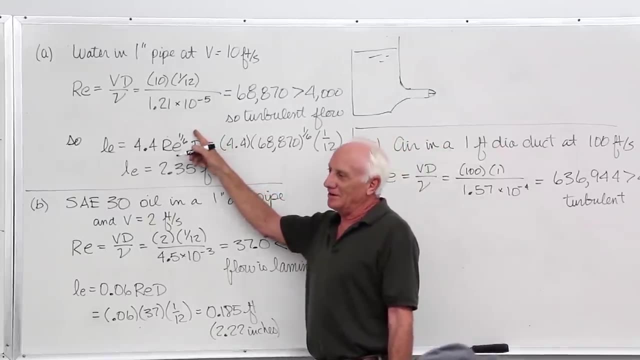 It's almost impossible to get turbulent flow. It's always pretty much going to be laminar Water. it's pretty hard to get laminar flow. It's probably going to be turbulent. but you could get laminar for slow enough flow rate. 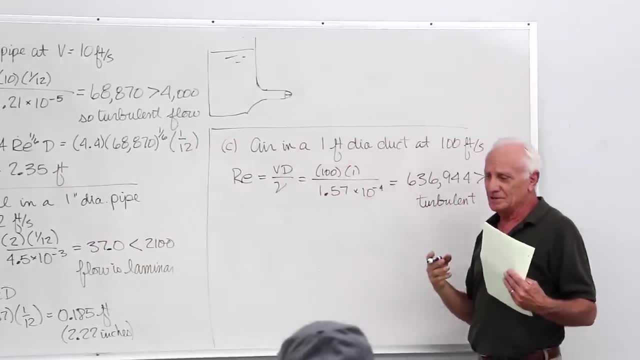 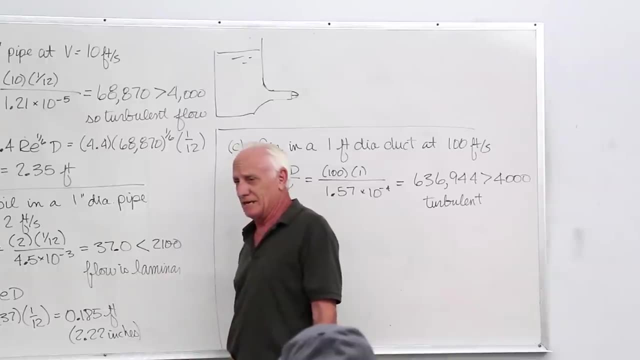 So we engineers know what to expect. Because we know what to expect if I get a Reynolds number for oil greater than 4,000, I'm going to say I think I made a mistake in my calculations. It's a big red flag. 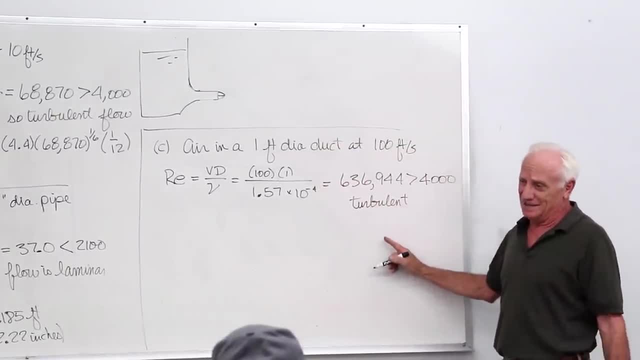 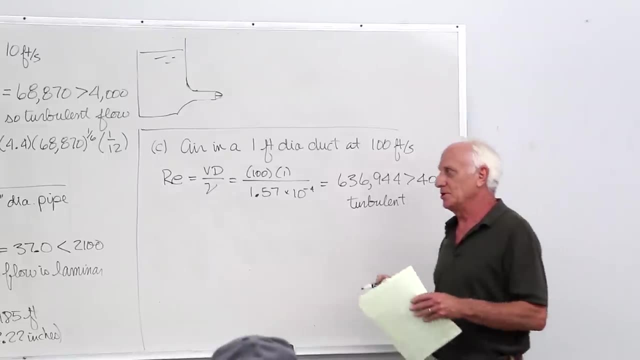 If I get air in a circular duct and it's laminar, I think you know that doesn't seem right. I think it should be turbulent. I better check my calculations. So these are warning signs, red flags that tell you what you should expect. 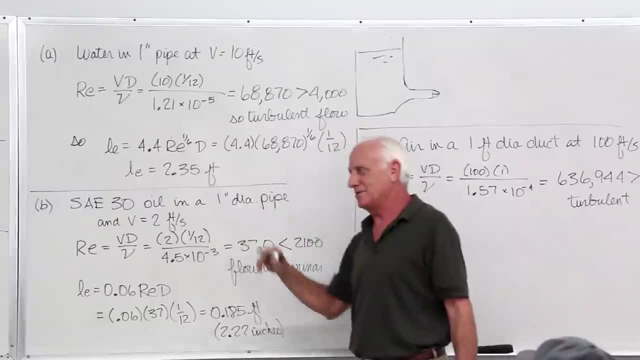 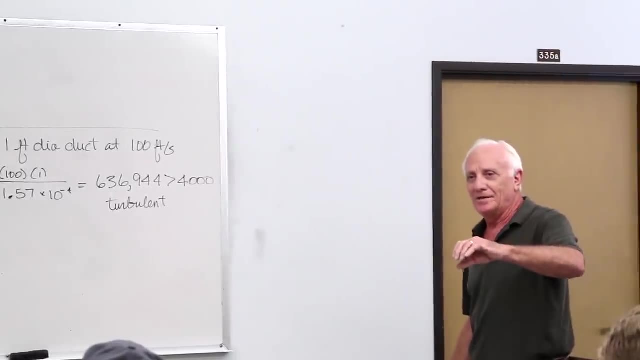 Water. I suspect turbulent, but there's an outside chance it could be laminar. You open your fossil kitchen. it's turbulent, Unless you barely open it and the water comes out beautifully smoothly out of that nozzle. it's probably getting down to where it could be laminar. 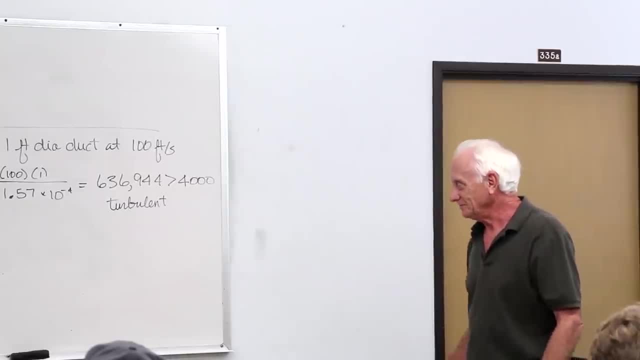 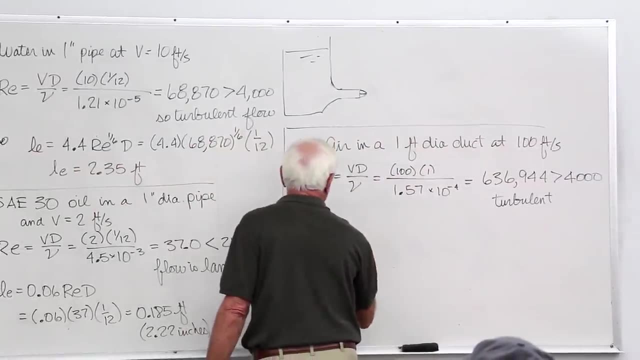 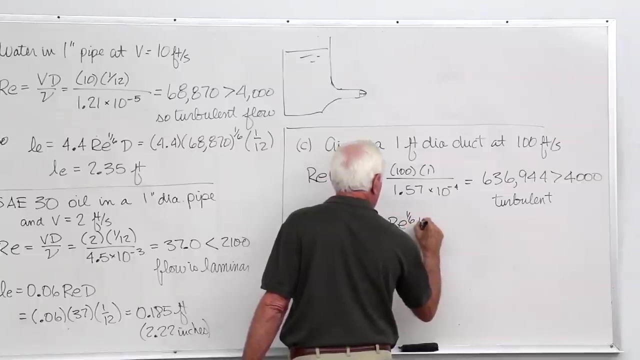 but not generally Mm-hmm. Okay, so let's go ahead and calculate this guy. He's turbulent, Okay. turbulent LE equal 4.2.. 4.4 Reynolds to the one-sixth times diameter. 4.4 Reynolds to the one-sixth. 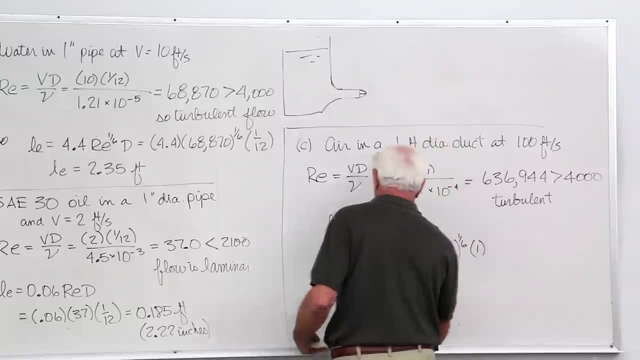 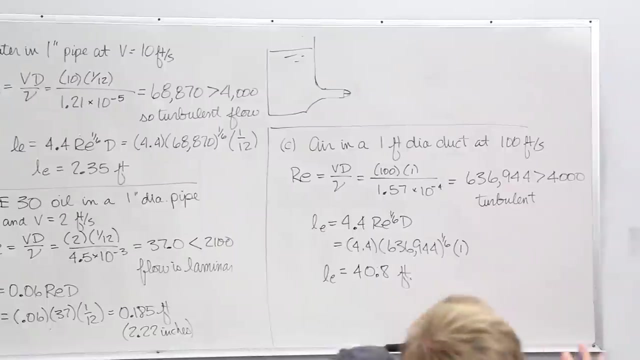 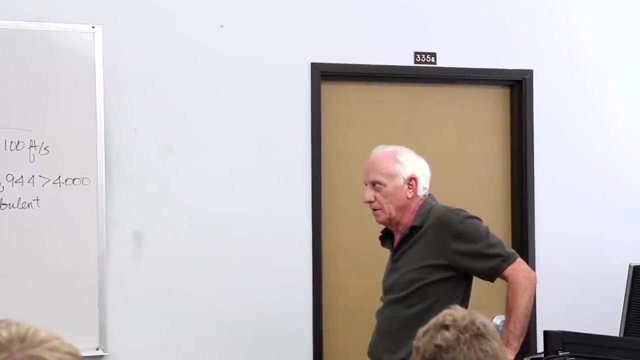 Diameter is again, it's one foot, So LE is equal to 40.8 feet. 40.8 feet- I can't draw on the board, You know. one foot diameter, 40 times longer than its diameter before those profiles reach fully developed turbulent flow. 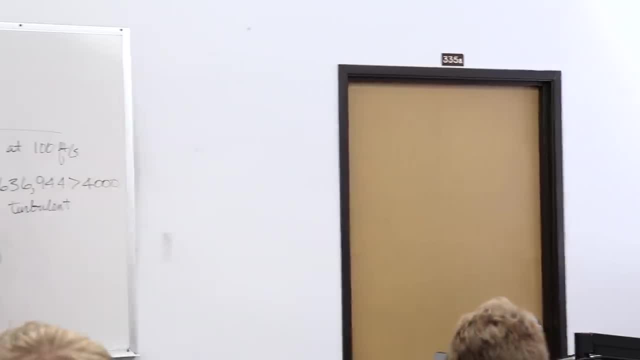 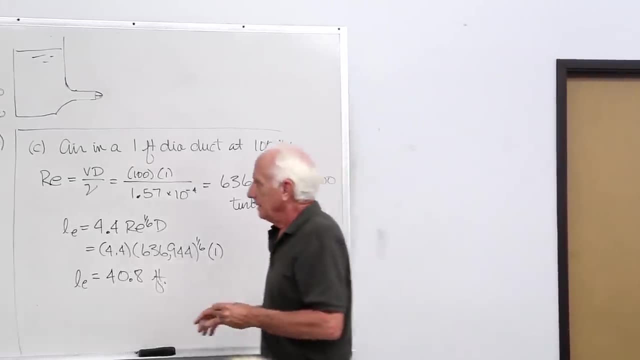 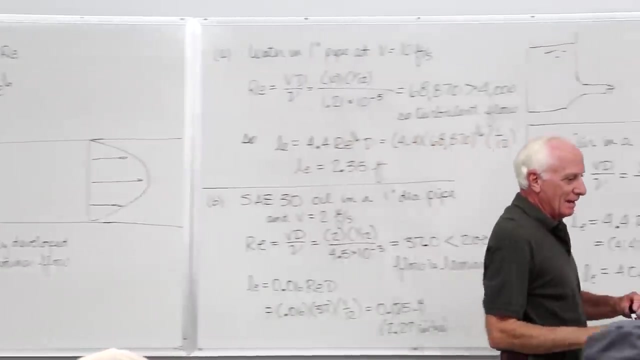 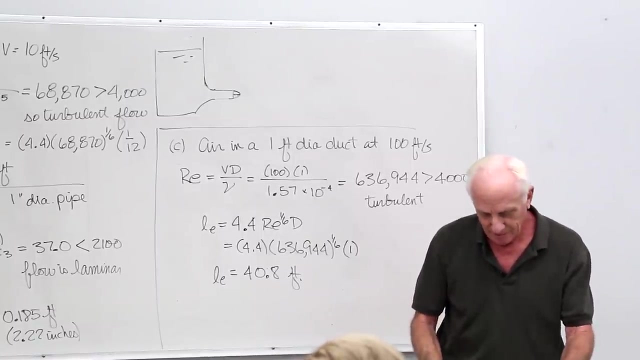 So it can vary from things like a couple inches to 40 feet, And these are the equations. you need to calculate that. Now let's talk about what happens if we put something like a valve in the line. So now I'm going to 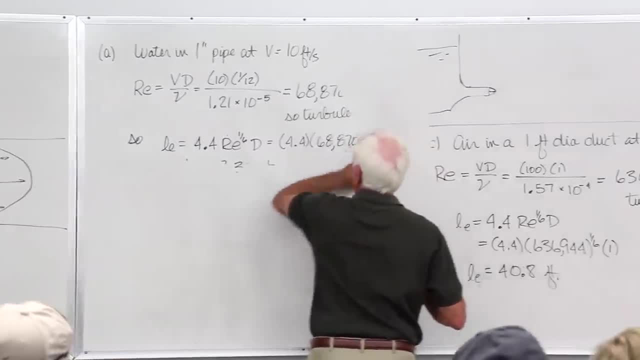 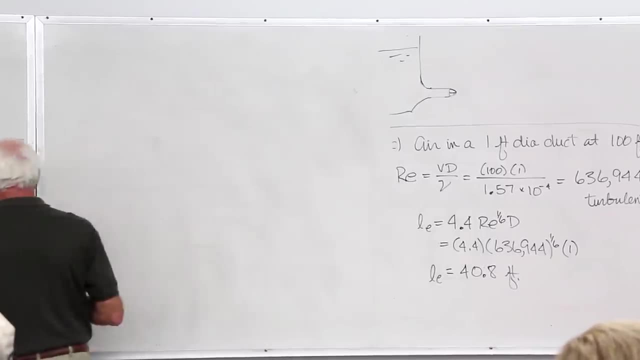 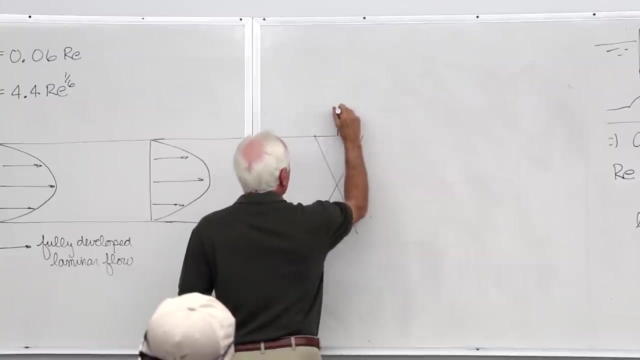 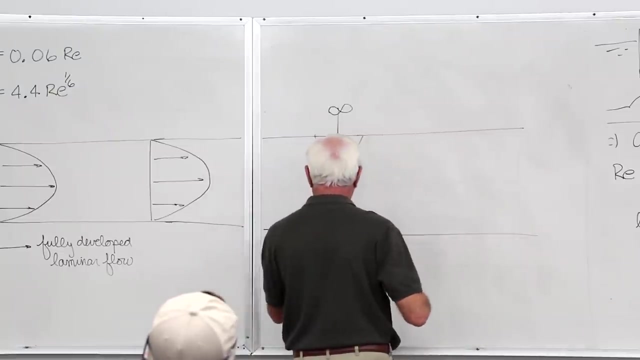 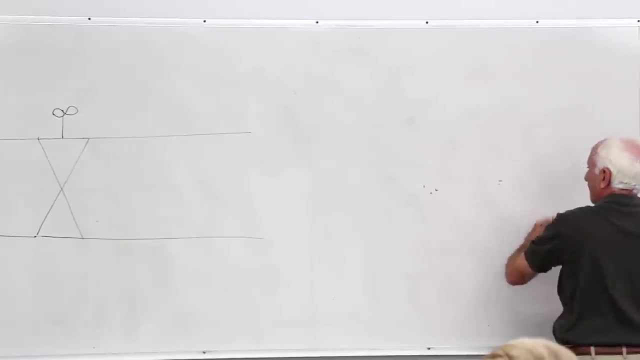 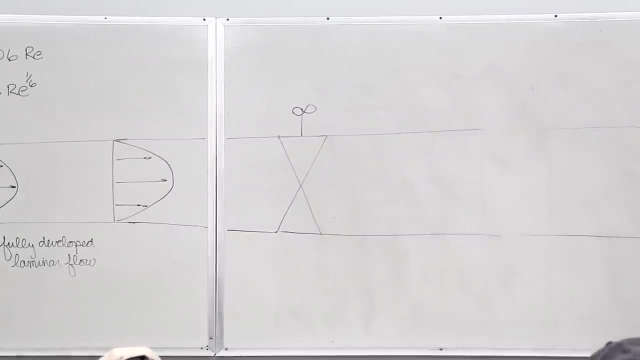 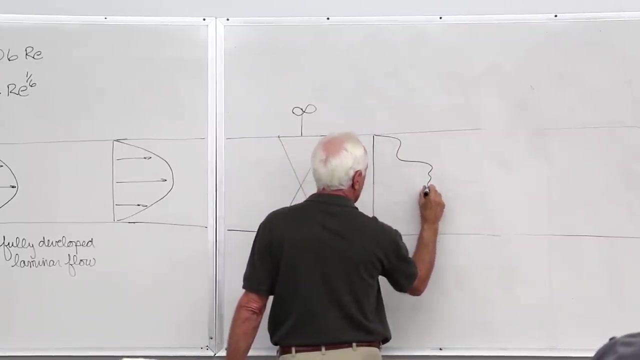 put a valve in that line. There's a valve in the line. Okay, we go down here After we have the valve in the line, And it depends what kind of valve it is, and so on and so forth. But we're going to get some strange velocity profile. 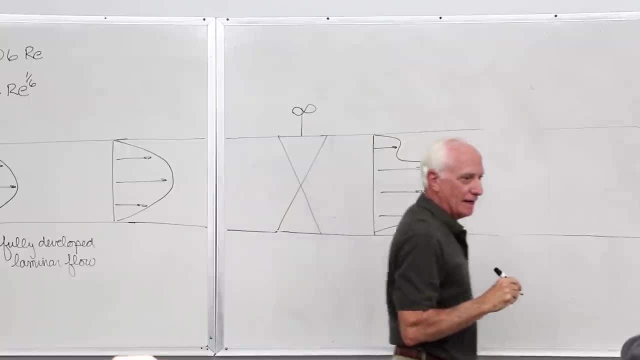 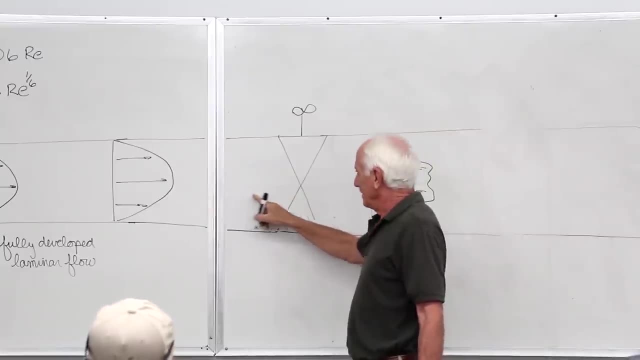 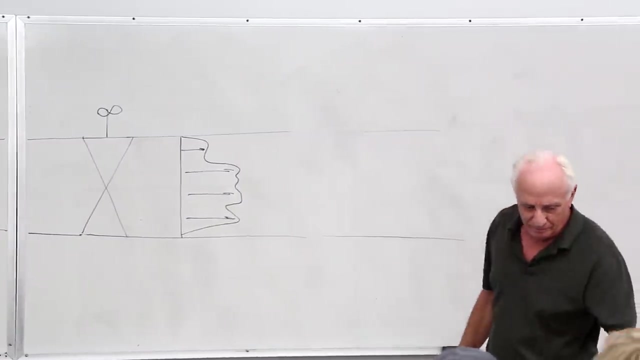 On the downstream side of the valve There's upstream and downstream. Upstream is to your left, That's called upriver Upstream. downstream is to your right in the direction of flow of the fluid. But if you go down past the valve long enough, 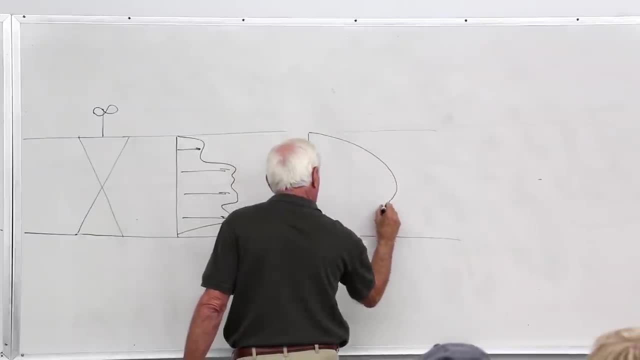 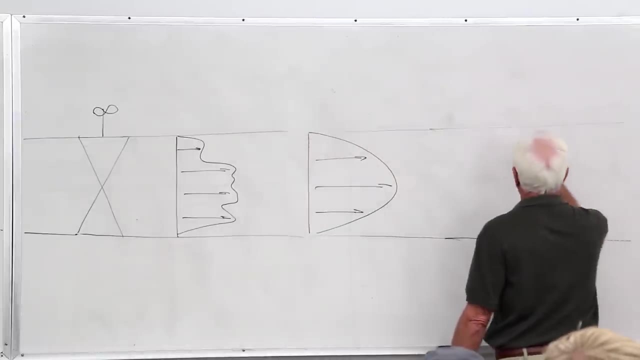 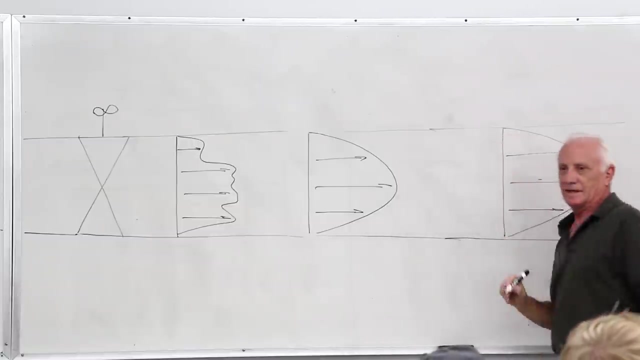 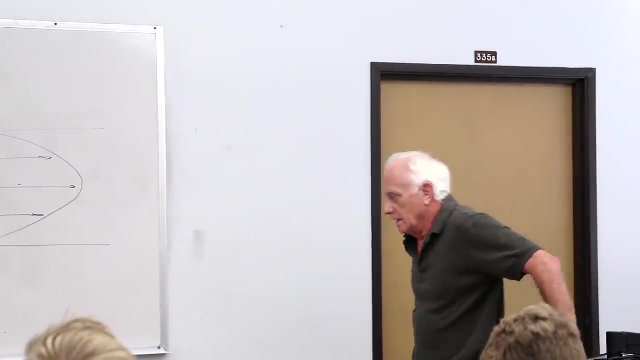 you're going to end up back here with a paramod velocity profile If you go down. this is the Alaska pipeline, I don't know. it's 300 miles long between pumping stations. So at the north smoke it looks like this. 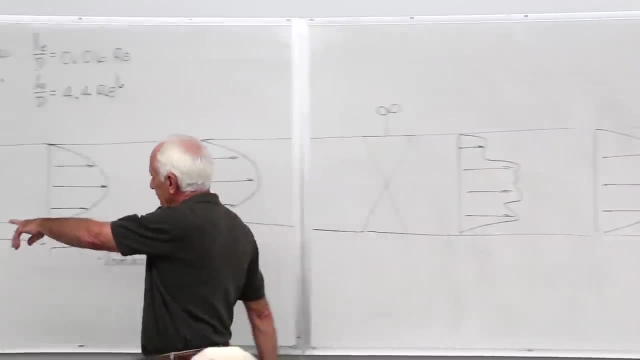 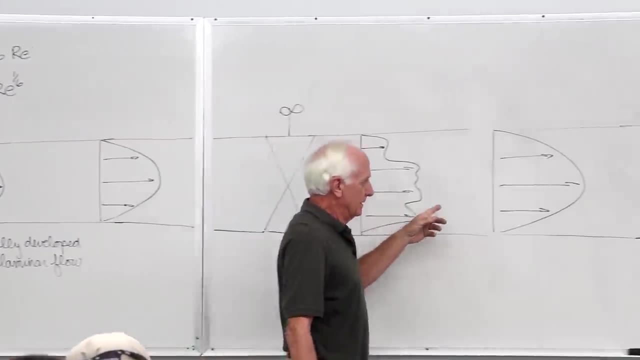 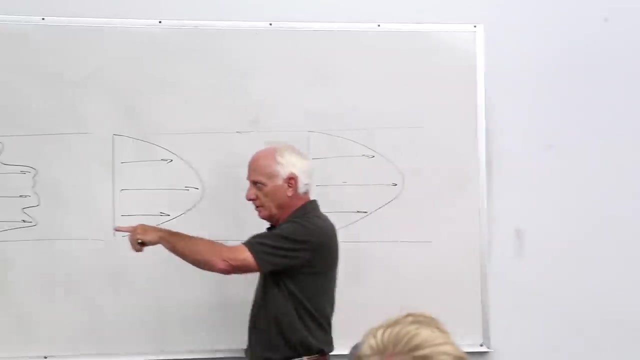 If it goes across the mountains down to Valdez, it looks like that, But if you go down to the north smoke, it looks like this, It looks like this, It looks like this. Guess what? It didn't change, Because here's the word, right here. 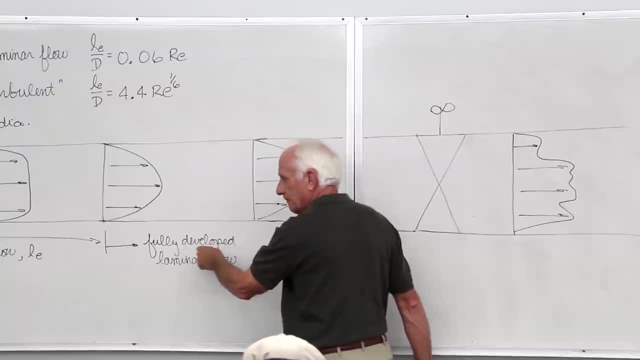 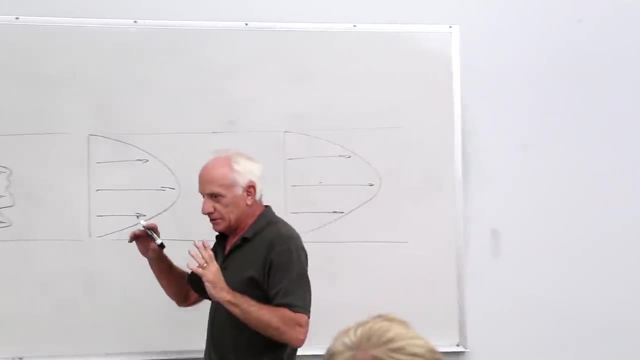 It's fully developed. Once you reach fully developed, it'll always go back to its fully developed shape. Oh, it'll never go turbulent If the dimer's the same. this flow here, I don't care how long the pipe is. 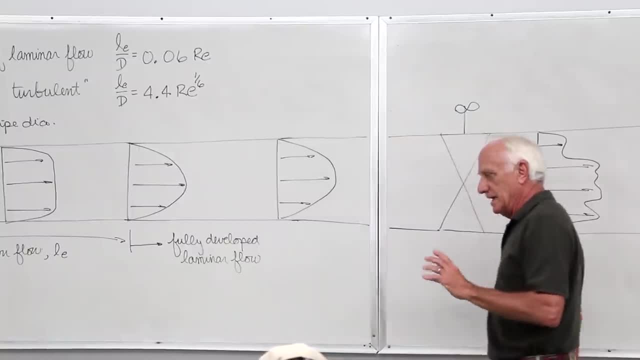 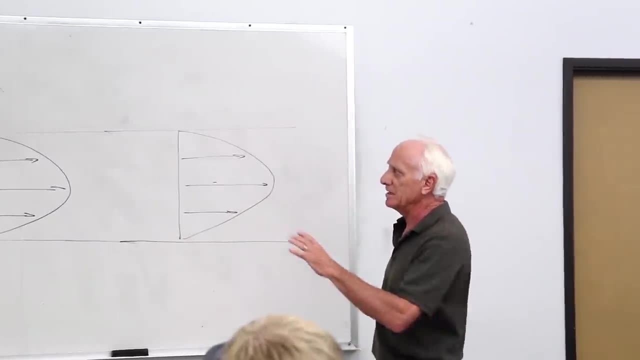 it's never going to go turbulent. If the dimer's the same, the temperature's the same for properties, then once it's fully developed laminar flow, it will stay that way. Now it could be tweaked If you put a valve in or an elbow in. 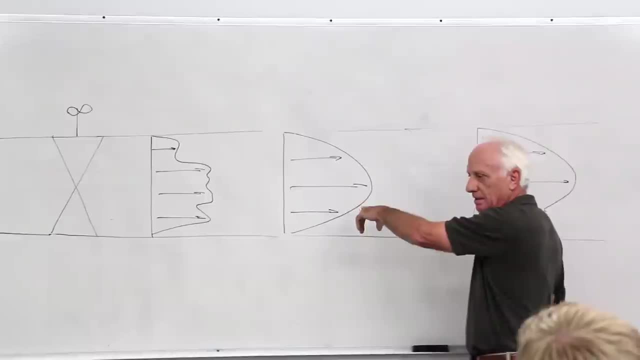 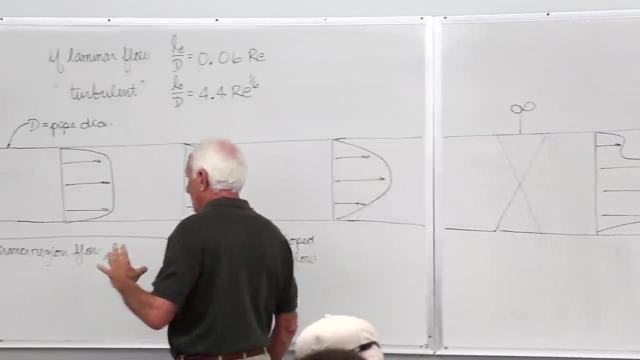 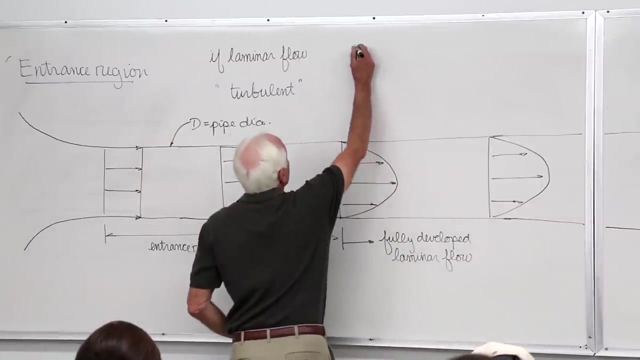 it'll come back to its shape again after it passes. that See, sometimes people get the wrong idea about this. I'm going to put this stuff down for you and make sure that you see what's going on here. I'm going to put down the M dot. 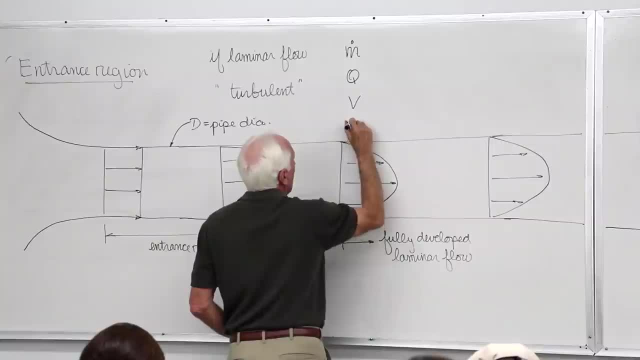 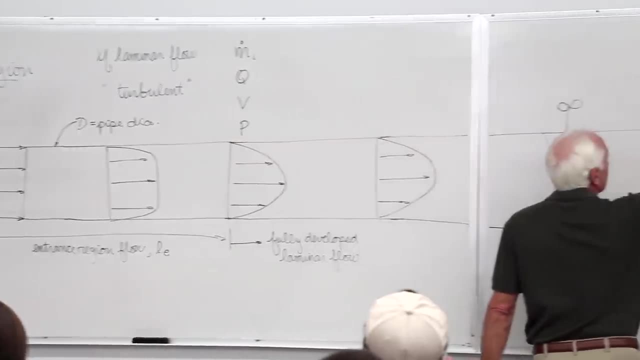 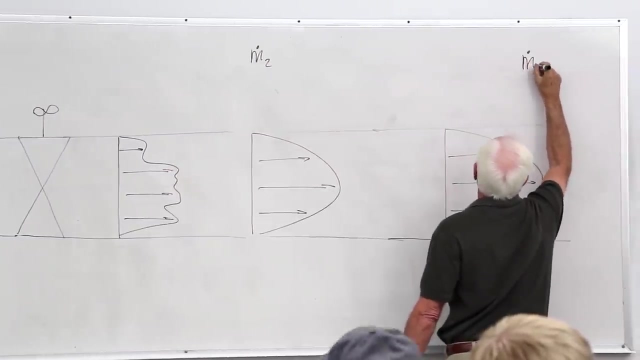 I'm going to put down Q, I'm going to put down B, I'm going to put down P. This is station one- M dot one. This is station two- M dot two. And this is station three- M dot three. 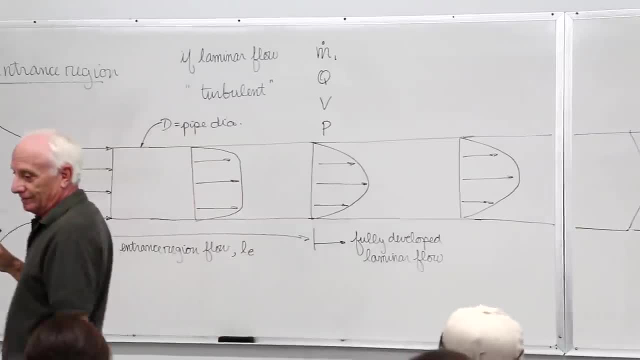 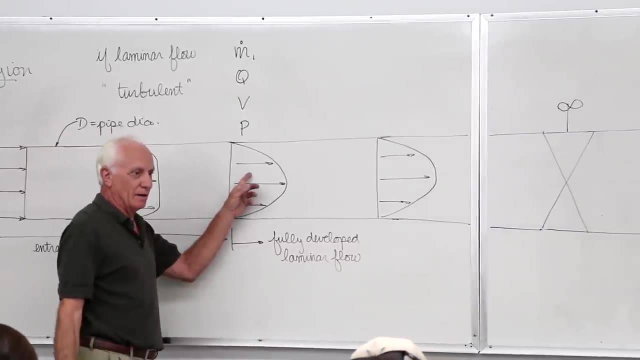 Well, you know what happens. Conservation of mass steady state. This is the Alaska pipeline Runs 24-7. Pumping so many gallons per hour here, so many pounds per hour of oil here. All the other end, pretty much the same amount. 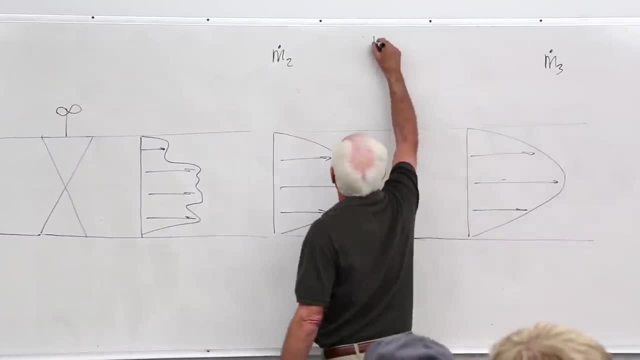 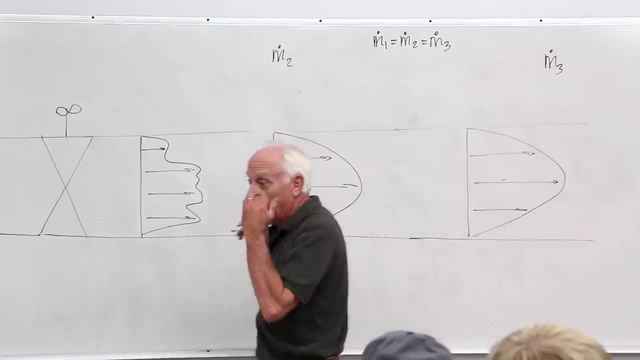 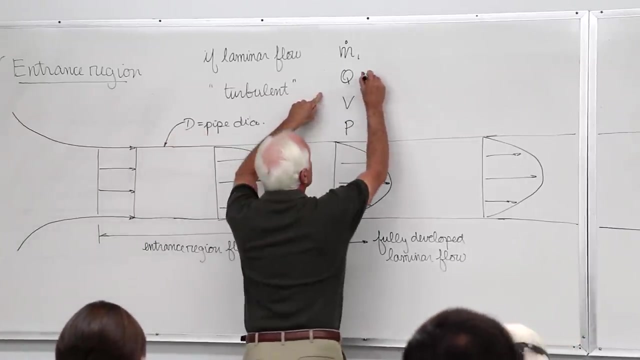 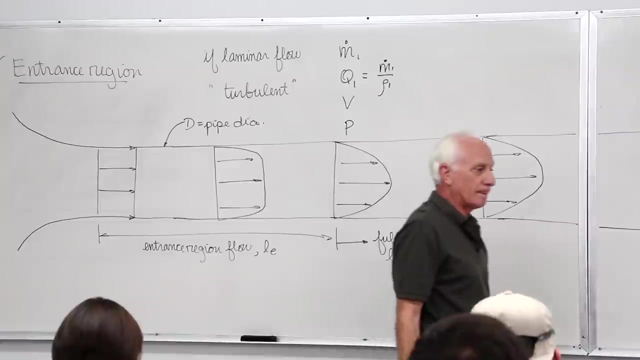 Steady state. So M dot one equal M dot two equal M dot three. All right, got that Steady state. Conservation of mass. Now we do Q. To get Q, of course, we take M dot at one and divide it by the density at one. 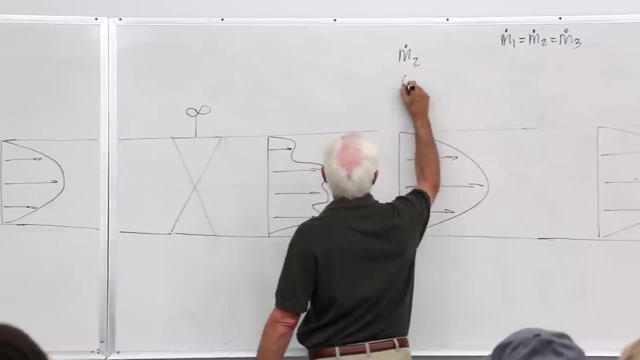 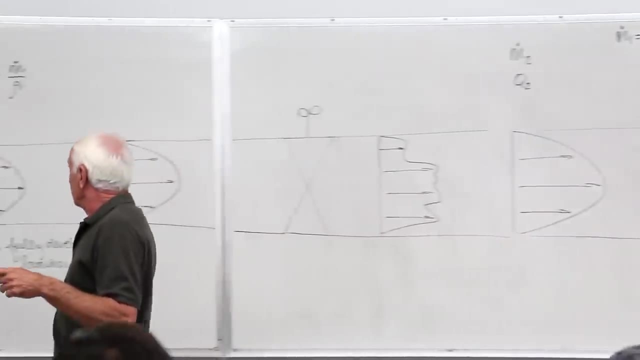 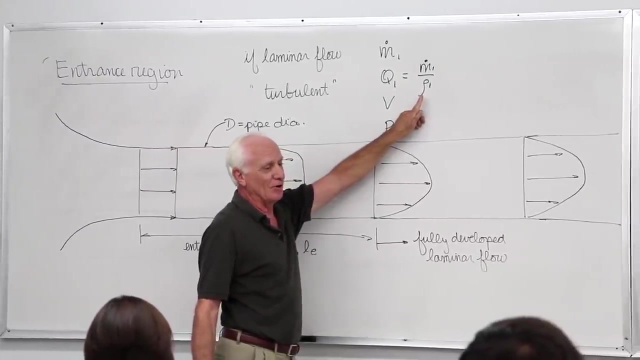 And this becomes Q two, And this becomes Q three. Now our rules are: same diameter, same temperature. Okay, Same temperature. We're not assuming the density is varying. Oil is pretty much incompressible. Okay, Constant, constant. 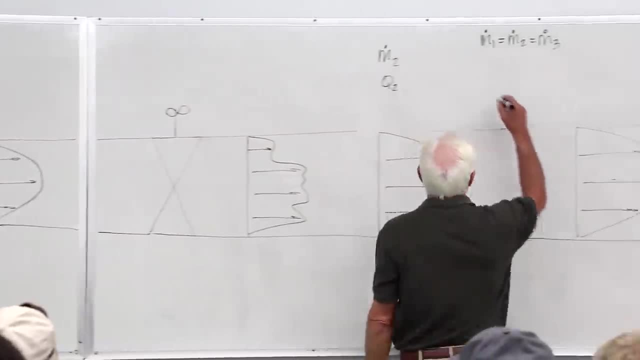 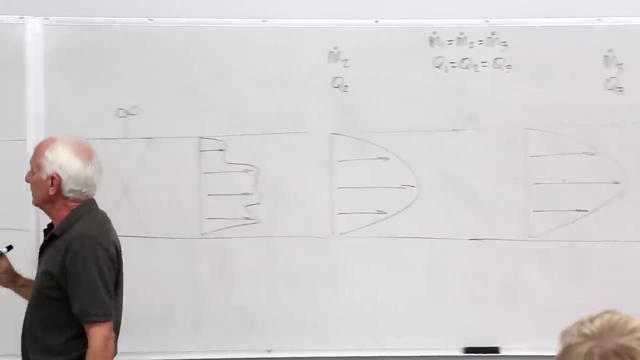 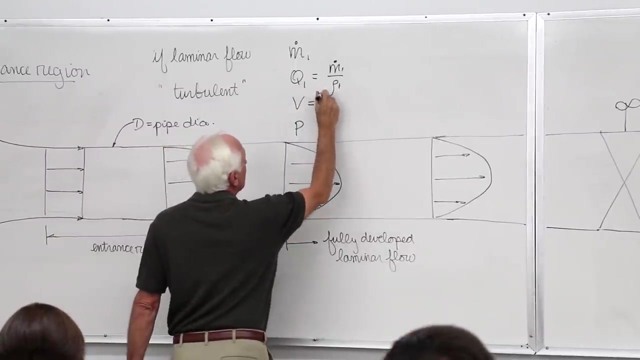 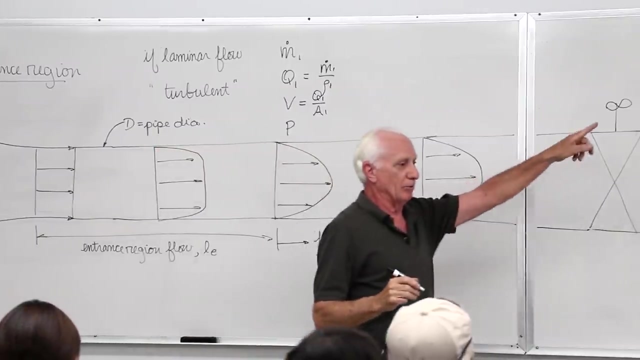 Q one equal Q two equal Q three. Okay, Let's take it one step further. If I have Q and I want V, Okay, Q equal V times A Q one over A one Dimers are same: A one equal A two equal A three. 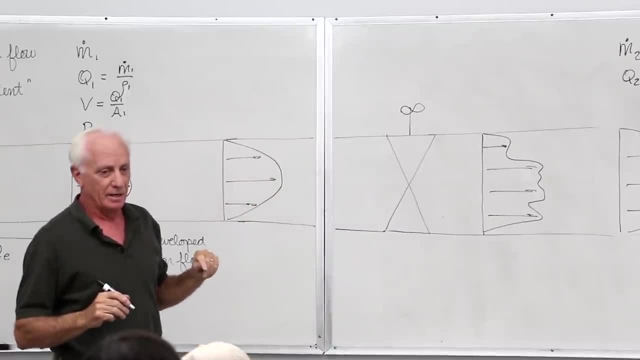 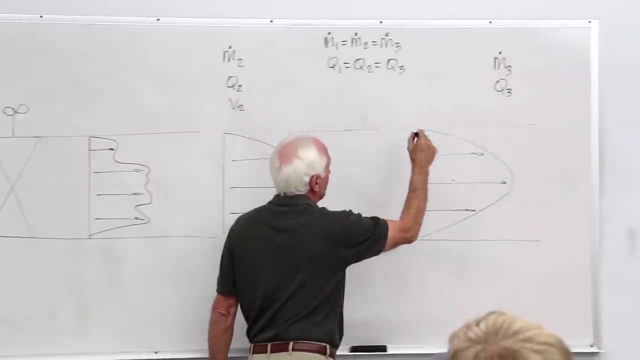 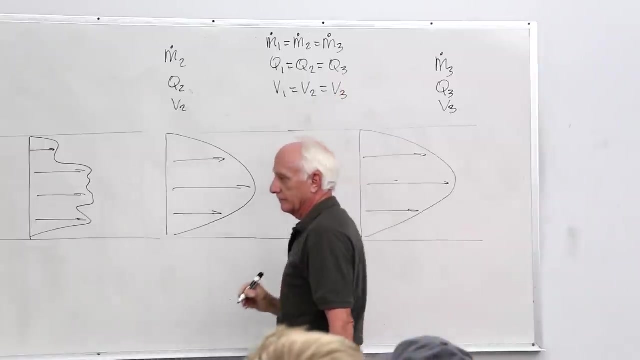 Q is the same, Q one equal Q two equal Q three. So guess what that says: V one equal V two equal V three, The average velocity. This is where some people have a little disconnect. They say: well, you know what? 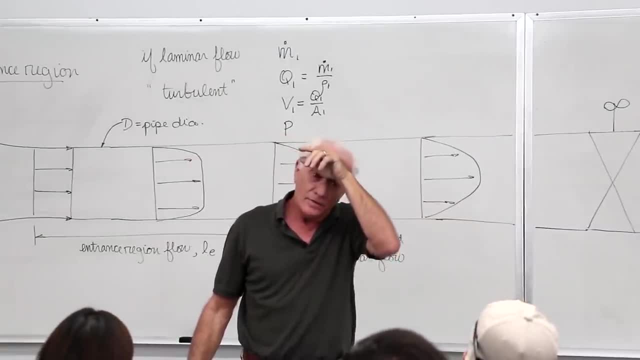 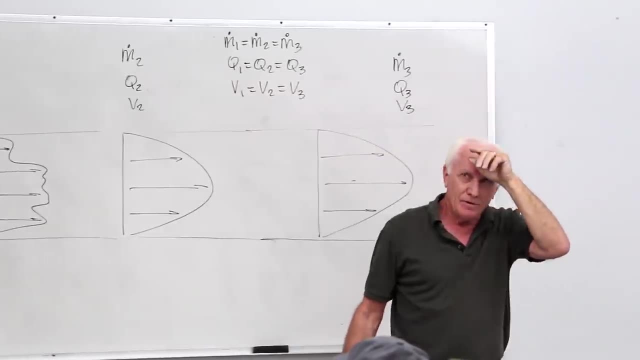 That pipeline's really long. I think the velocity doesn't slow down. I think the oil slows down. Oh no, it doesn't. And they say, well, why not? I say, did you ever hear about something called the conservation of mass? 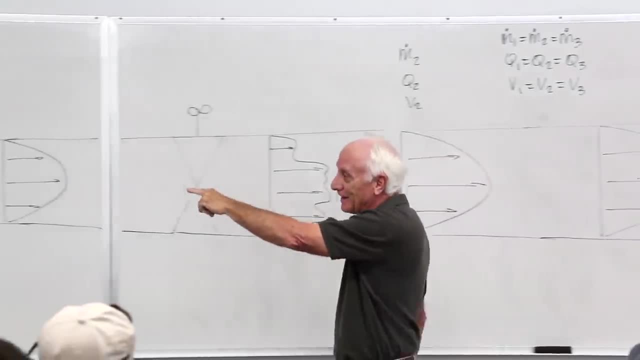 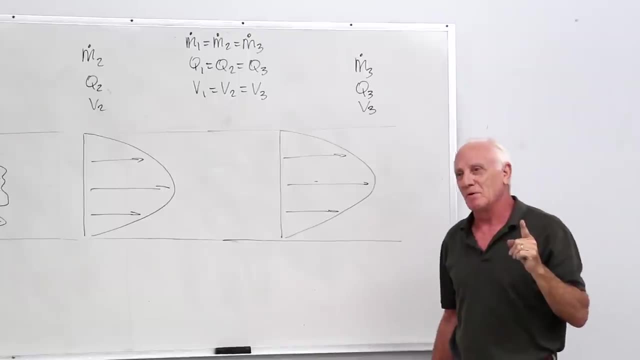 The steady state. Yeah, What comes in that side goes out that side in steady state Mass flow rate. Oh, no, no, no, The velocity does not go down, Don't get that wrong. Some people make that wrong assumption. 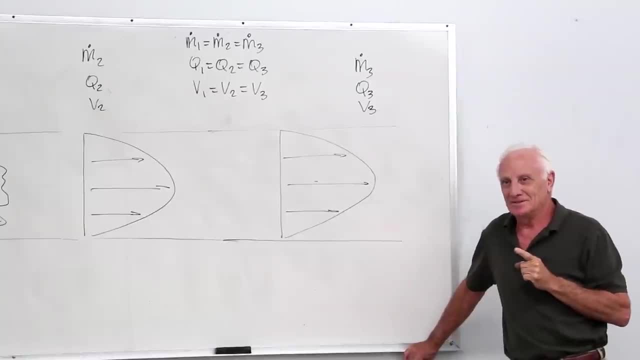 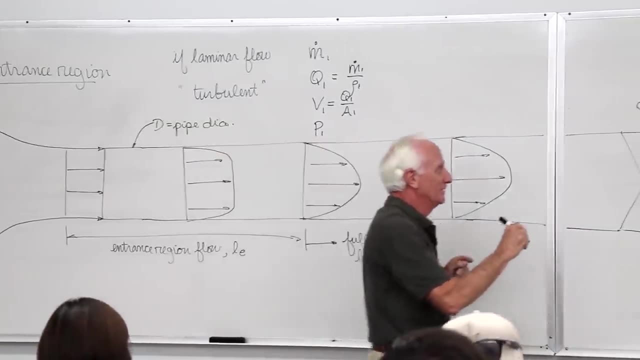 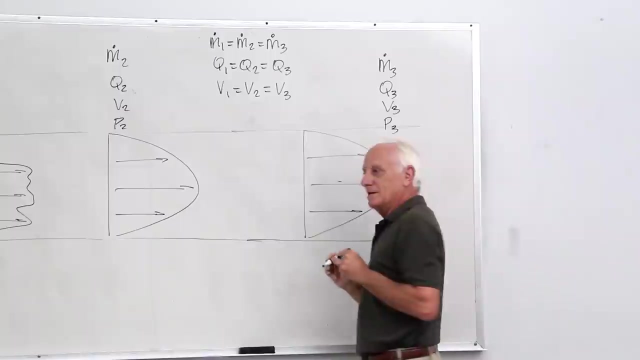 Now I put on the board the big, major clue. Guess what goes down with friction in a pipe? There it is High pressure, Lower pressure, Lower pressure. So guess what happens in the elastic pipeline After the pressure gets down too low? they go through a pumping station. 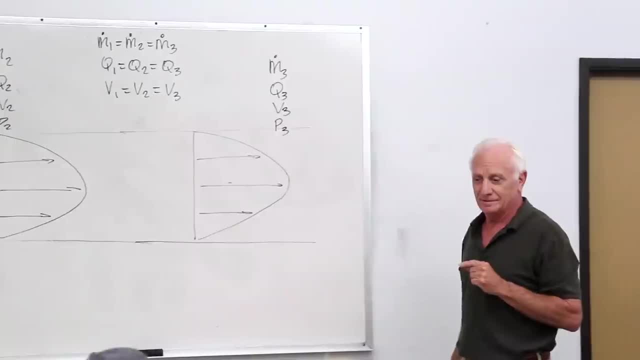 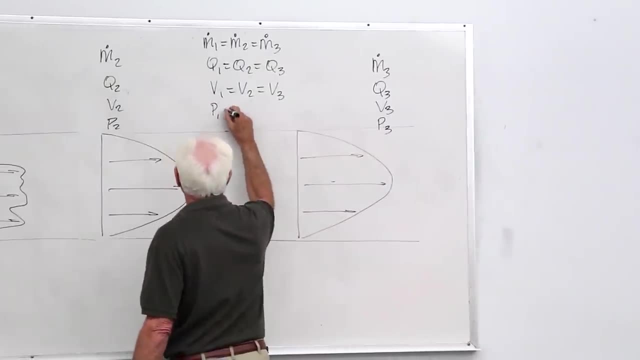 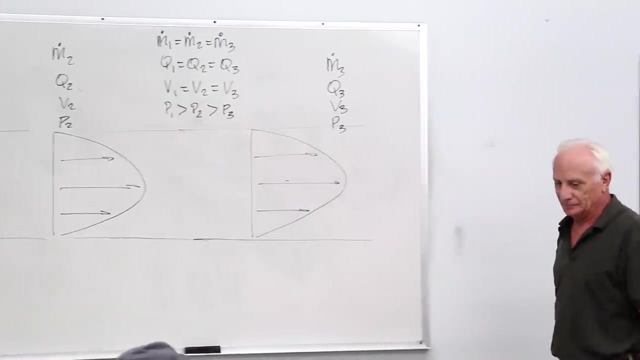 Why? To increase the pressure. That's what a pump does And that pumps the oil to the next pumping station. So what goes down? P one is greater than P two is greater than P three- And what causes the pressure to go down? 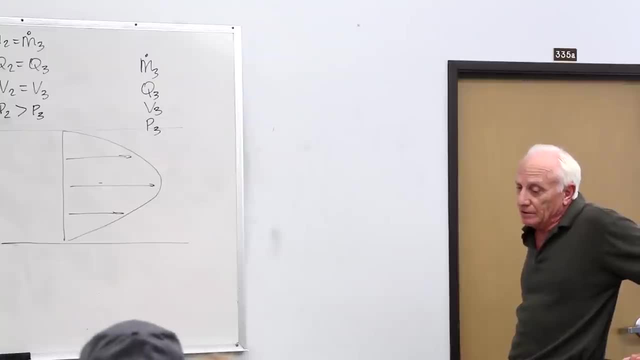 I'll tell you. Bernoulli's would say: for a horizontal pipeline, if V one equals V, two equals V three, and Z one equals Z, two equals Z three. Bernoulli's would say: V one equals P two equals P three. 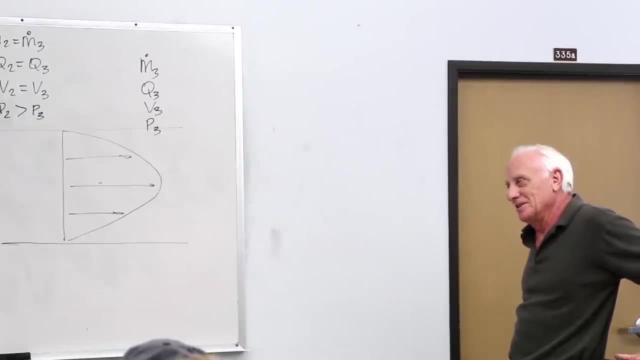 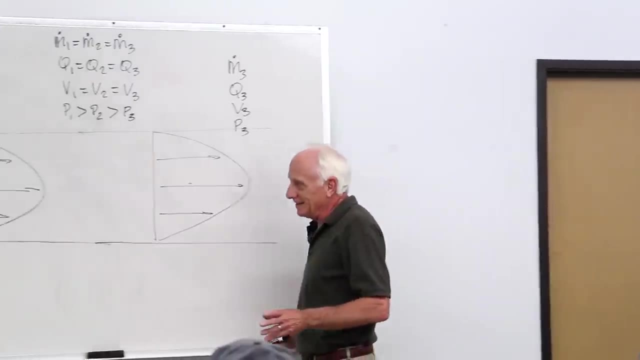 This is not in Bernoulli's world now. Now we have friction, What does friction do? It takes energy out of the fluid by shear stress on the walls. So yeah, this is the energy equation: The pressure goes down. The pressure goes down as you go from left to right here. 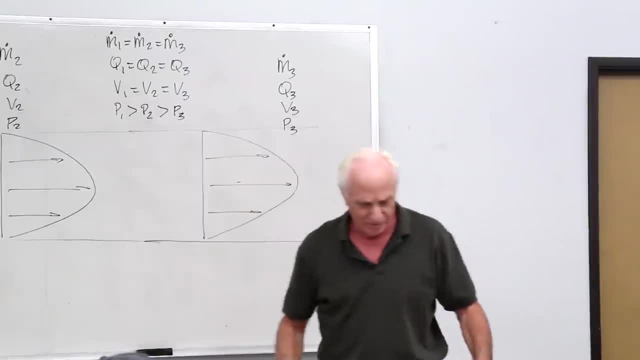 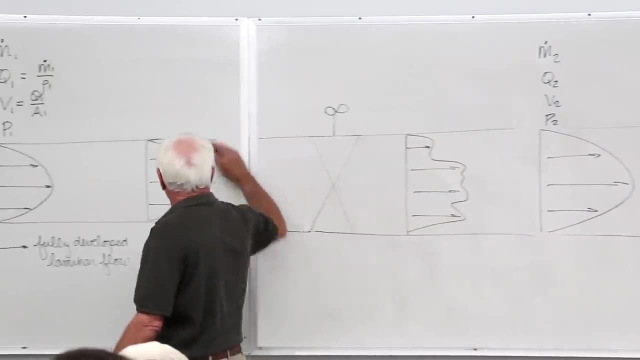 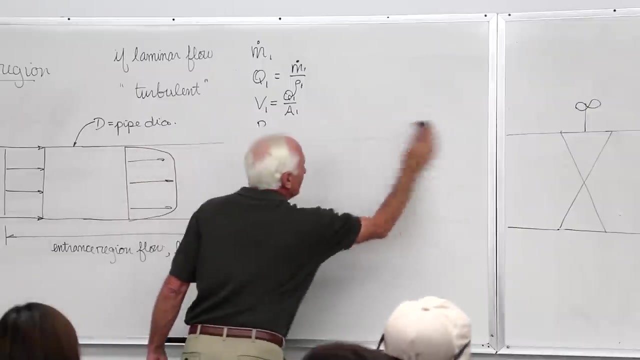 Okay, so just to avoid any misconception about, does the velocity go down in the pipe as you go down in the flow direction? No, no, Conservation of masses cannot happen for a steady state. Okay now we talked about the flow being parabolic for a fully developed glamour flow. 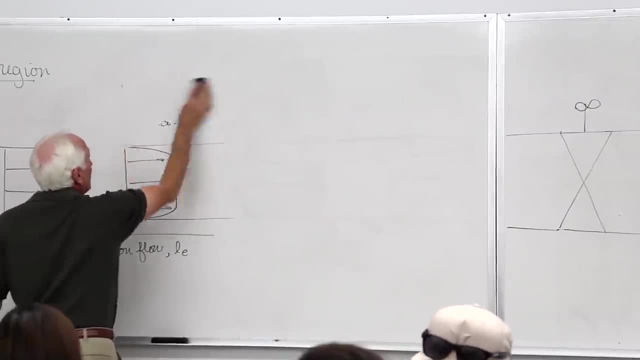 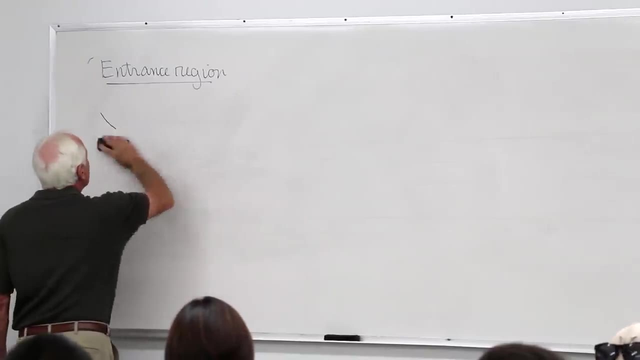 All right, How do we know that? All right, we're going to prove the velocity profile shape. now We're also going to find out something about the friction, Friction loss in a pipe. So now we start off to show that the velocity profile is in fact parabolic. 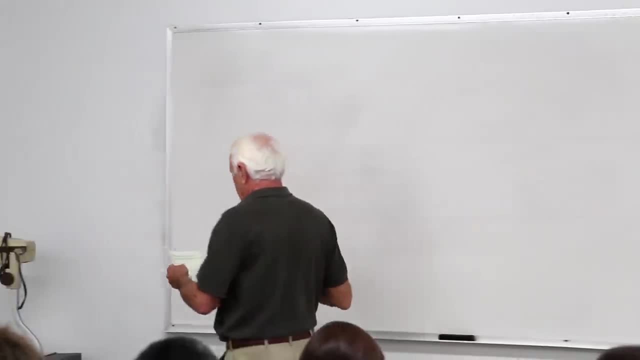 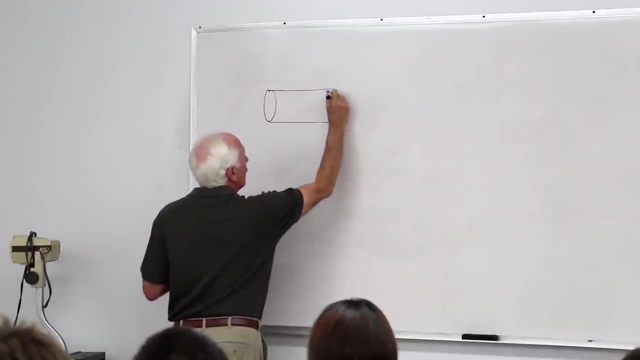 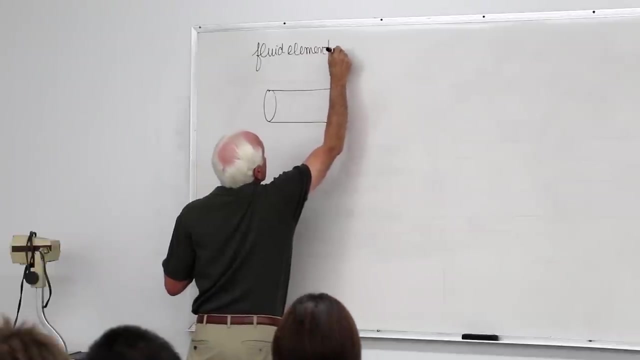 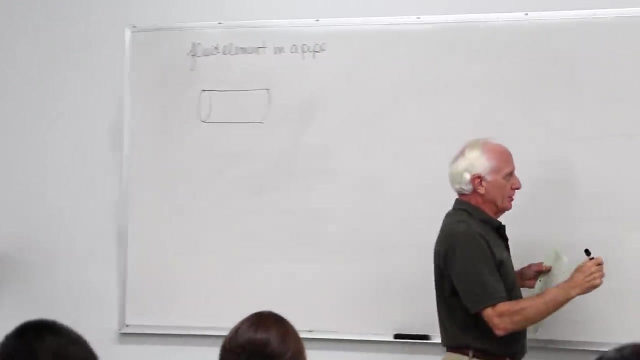 All right, let's see To do that. we take a little cylindrical element of fluid in a pipe. So here's the fluid element in the pipe. So I'll just show you over here real quick If this is a pipe. we take a little fluid element out. 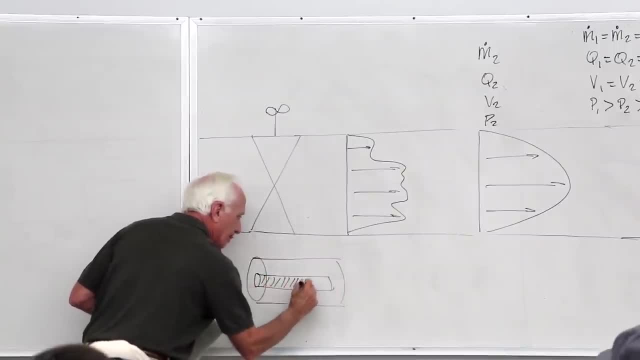 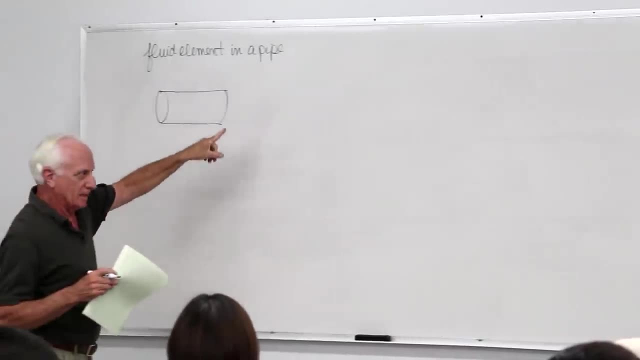 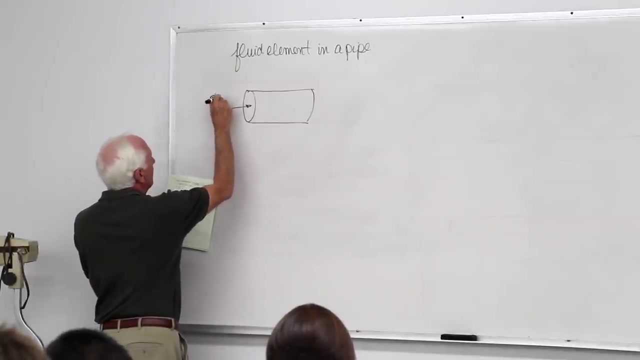 It looks like that. Take it out of the fluid. That's the fluid, A little fluid element taken out of a pipe carrying a fluid. On the left side there is a pressure force. Pressure force is P1A1.. This side there is a pressure force P2A2.. 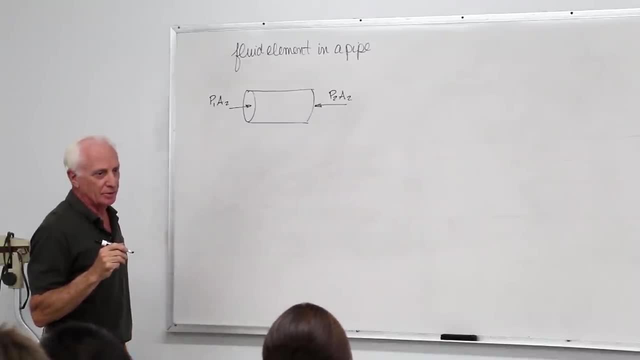 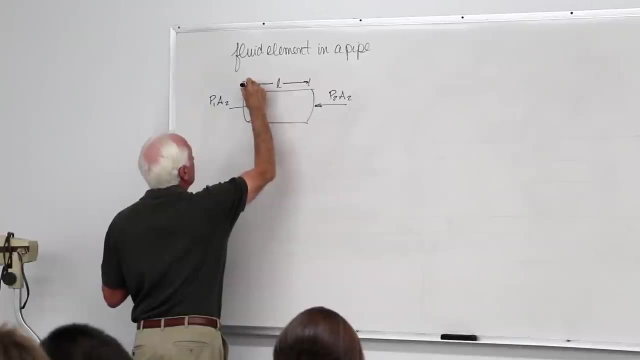 Pressures are compressive stresses. They always point into the fluid control volume. This thing has a length of L and a diameter of 2 times the radius. The shear stress acts this way. This is the force due to shear stress. It acts to hold the fluid back. 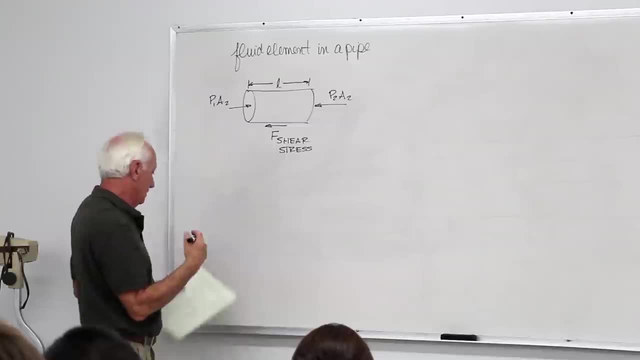 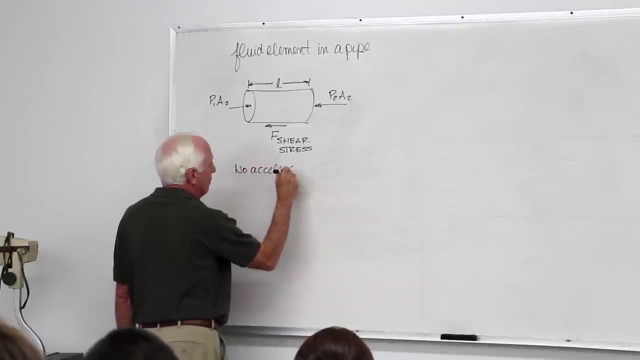 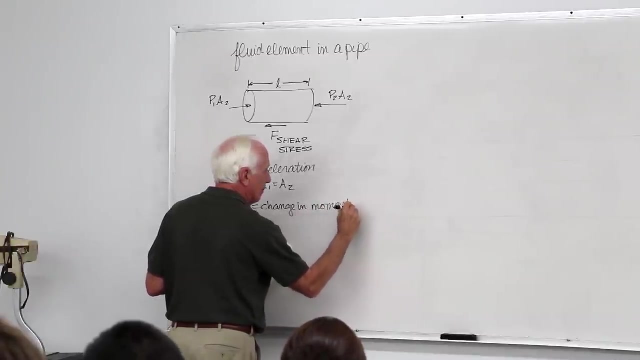 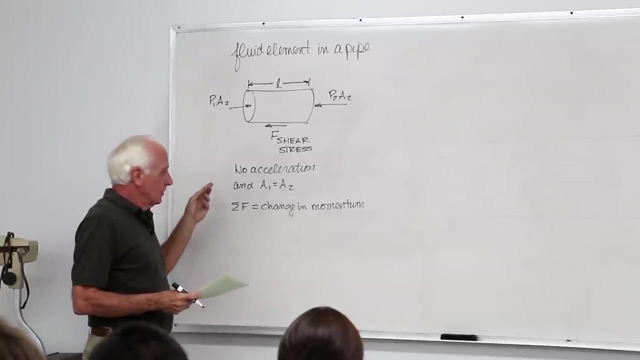 The shear stress wants to hold the fluid back. This is a steady state, no acceleration. So we also note that A1 equals A2 from the picture. So we get summation of the forces equal to change In momentum. momentum coming in rho, Q times B. 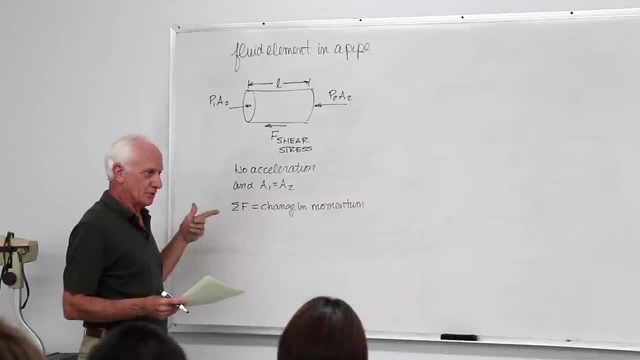 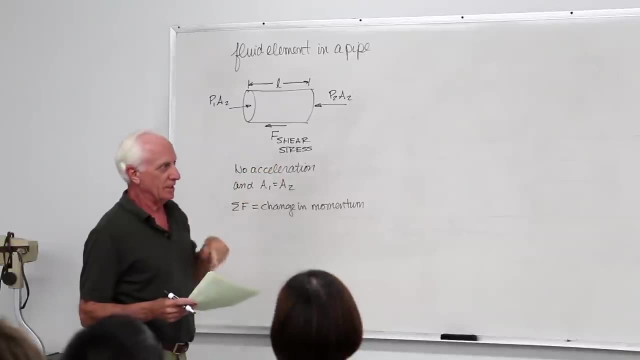 Is rho the same? Yes, in and out. Is Q the same in and out? Yes, it's the same. Is the velocity the same in and out? Yeah, I just showed you, it's the same in and out. 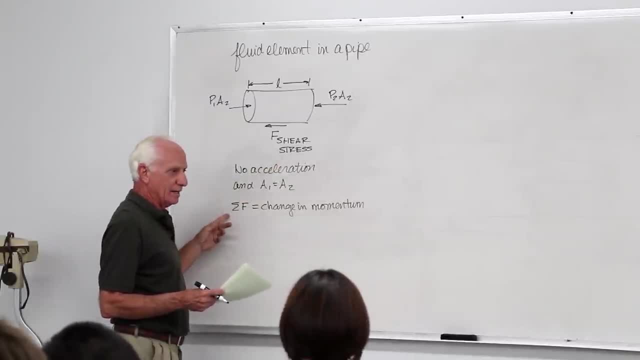 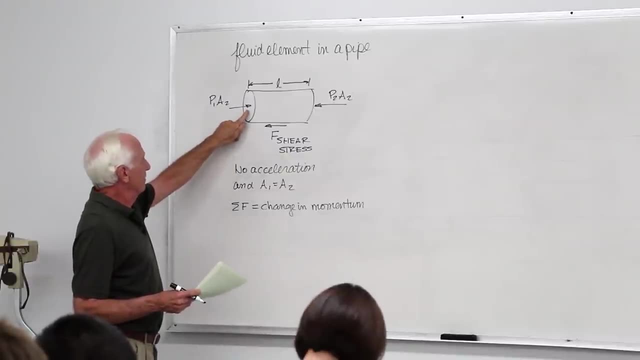 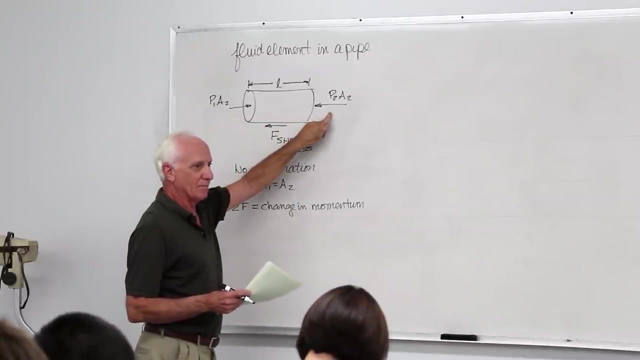 Conclusion: rho QA. rho QA is the same in and out. One's got a minus sign, one's got a plus sign. V dot A negative, The velocity positive. V dot A positive, The velocity positive. Positive times: positive is positive. 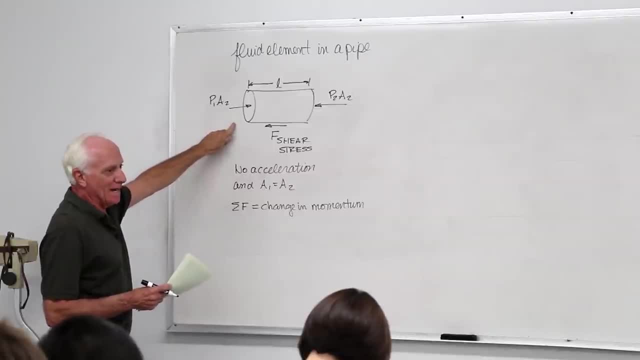 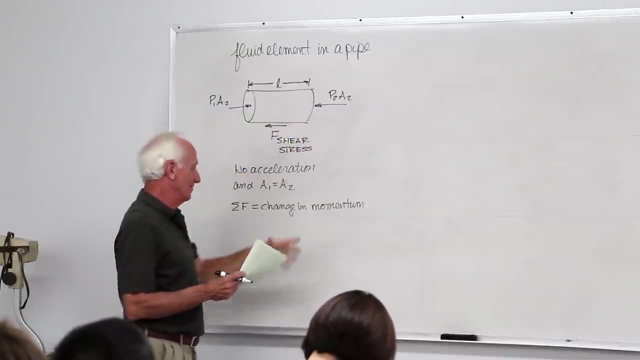 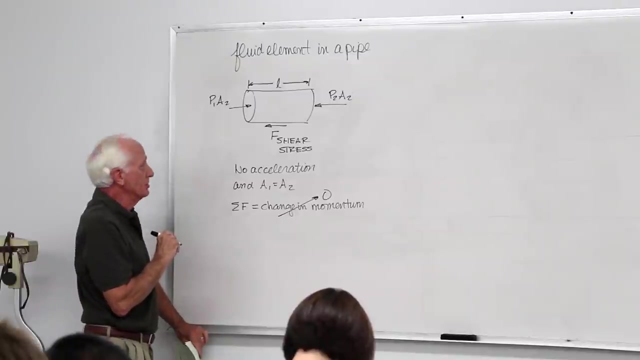 Positive times negative is negative. This is minus rho Q. times B. This is plus rho QB. It's not allowed Zero. What forces act on that load control surface? Obviously pressure and shear stress. To the right is positive P1- A1, to the left, negative. 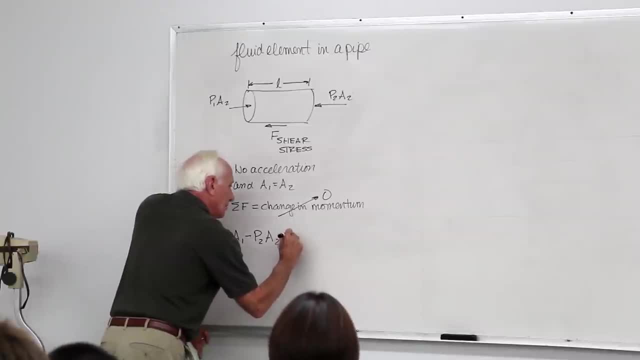 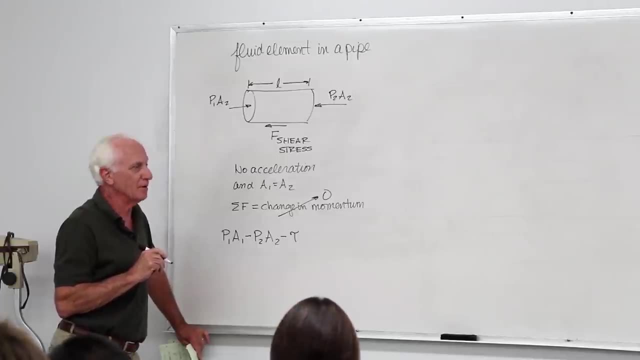 P2 A2.. Shear stress: negative Tau. To get a force for a shear stress multiply by an area. What area? The area where the shear stress acts? Where is that? The circumference times the length, Pi, D times L. 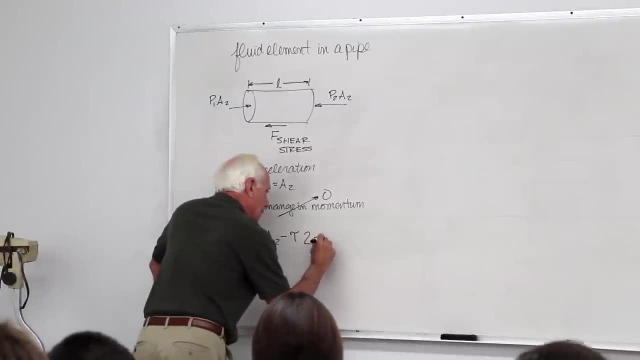 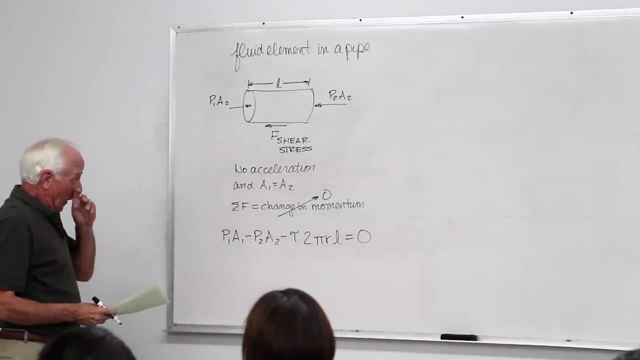 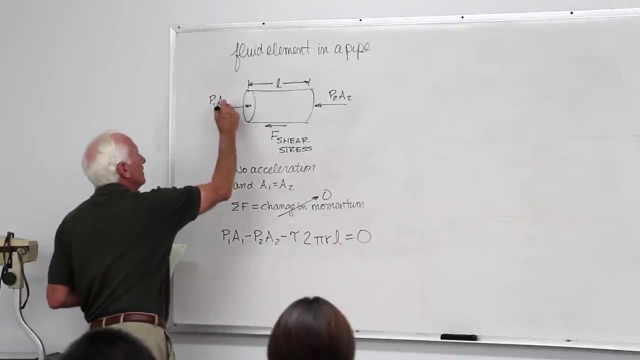 Or 2 pi R L Equal Zero. Okay, That was chapter five. Yeah, chapter five. Oh, thanks, Thank you, I sure do. Thanks so much, Yeah, Okay, Now we're going to Now notice. the areas are the same. 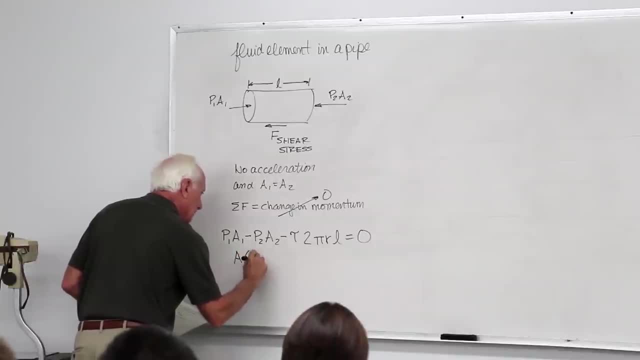 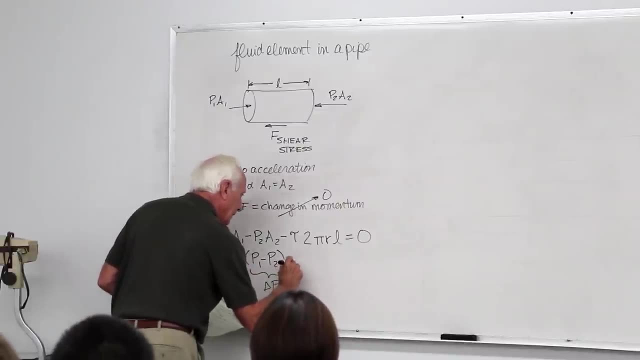 So we're going to say A times P1 minus P2.. And we're going to call that delta P in our equation And that's equal to the shear stress. Let's put it this way: Tau, That's okay. 2 pi R L. 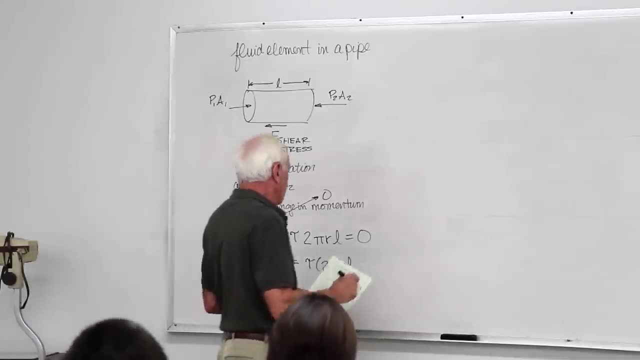 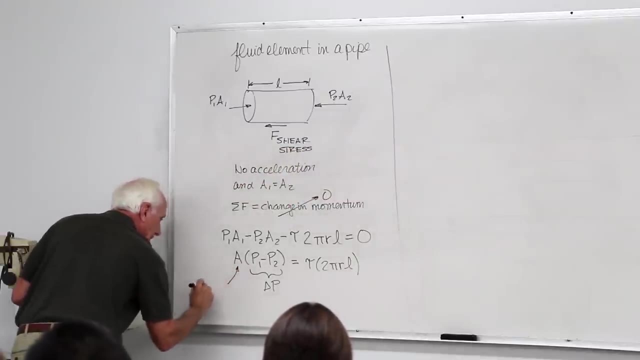 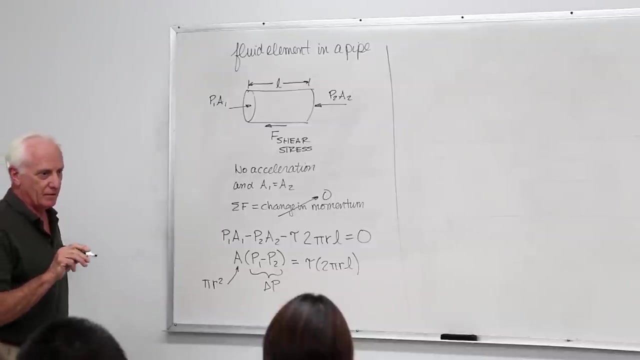 Minus sign gets a plus sign. So if we, If we The area, This area is pi R squared- Get the areas right. There's an area for the shear stress. There's a different area for the pressure force. The pi's cancel out. 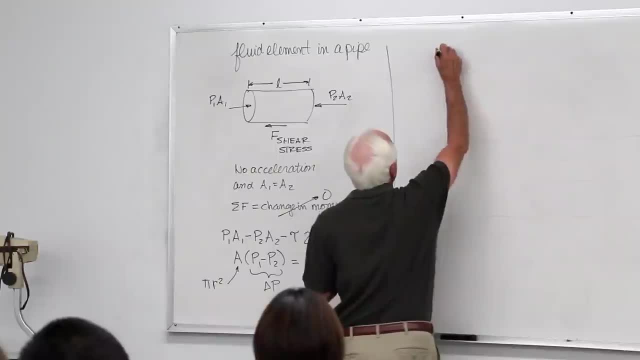 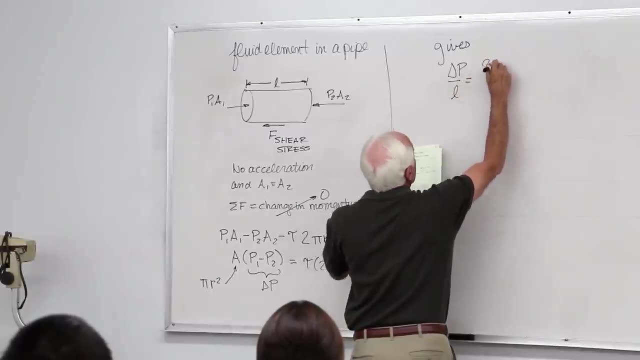 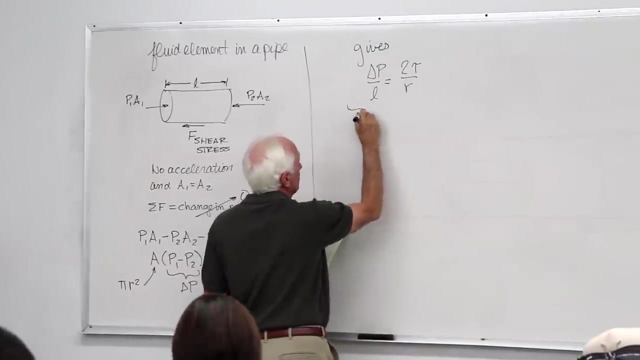 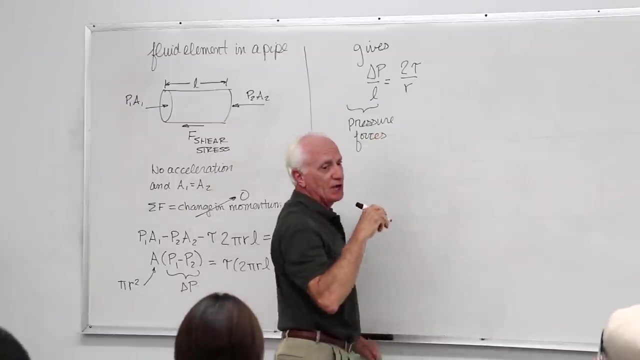 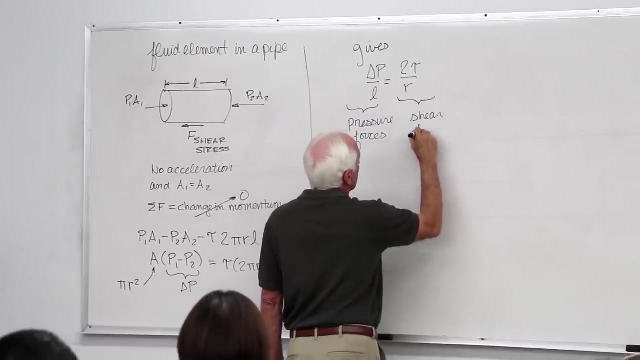 One of the R's cancel out, You're left with this. This side is the pressure forces and the shear forces. What I mean by that is it's related to. It's related to the pressure forces. This is related to the shear forces. 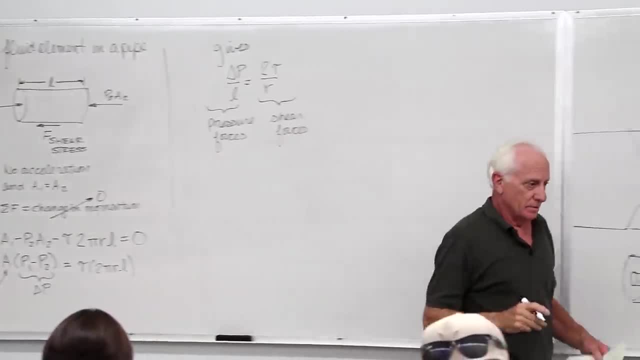 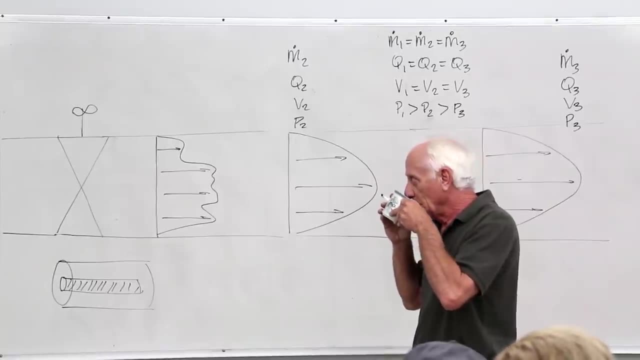 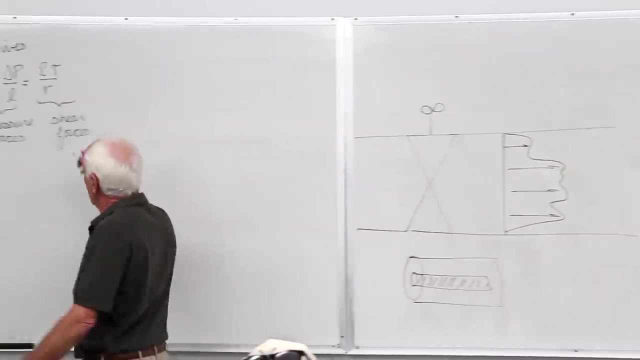 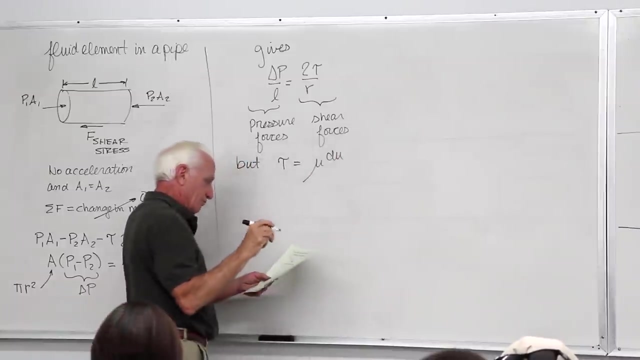 What does that tell you about that little element there? For that little element, The net pressure force equal the net shear force. The two balance each other. They're equal. Okay, Now we bring in tau, Chapter 1. Now we have to bring in the radius, because that's what we're looking at. 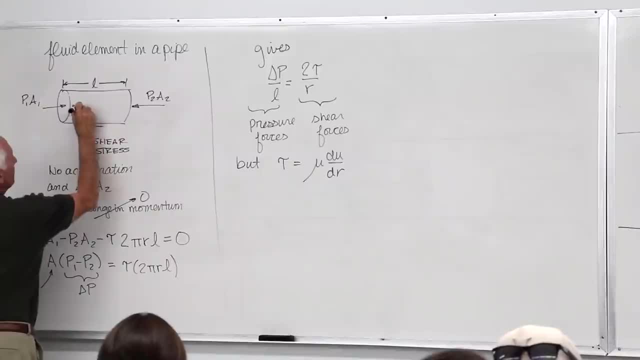 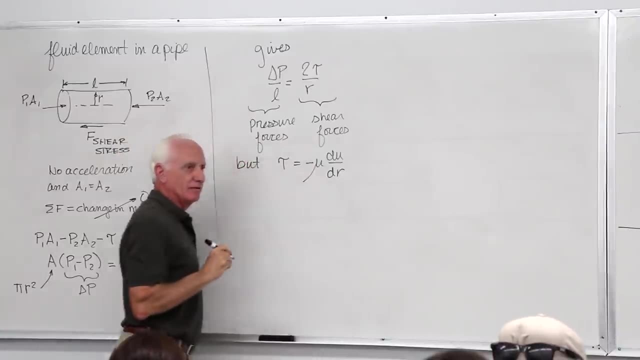 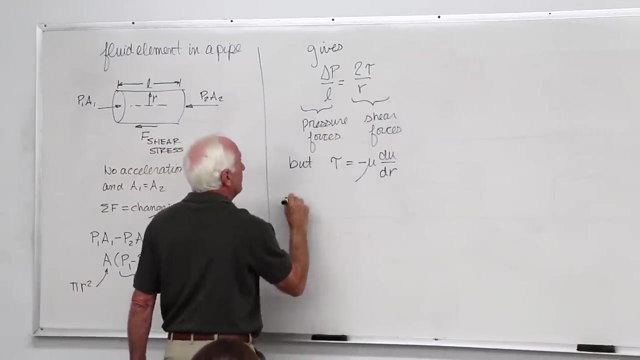 We're looking at the radius. Okay, So we can measure this. This is the radius R, right there. Minus sign in front of it, Minus sign in front of it. So put that up here. Delta P over L, 2 tau over R. 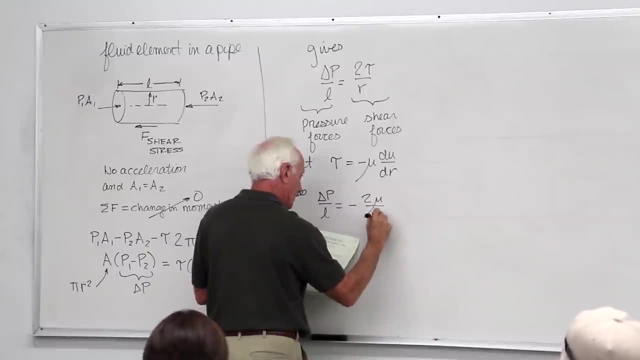 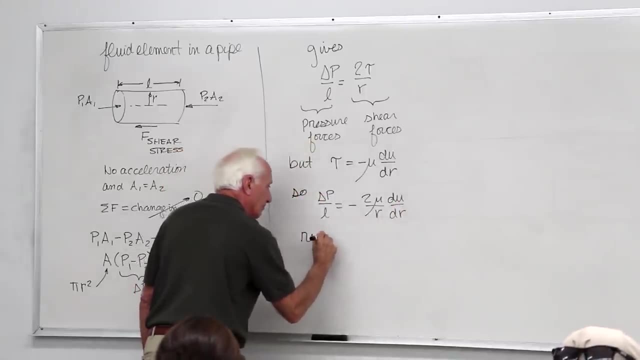 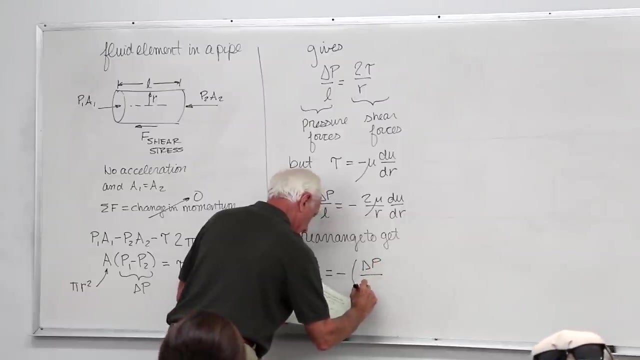 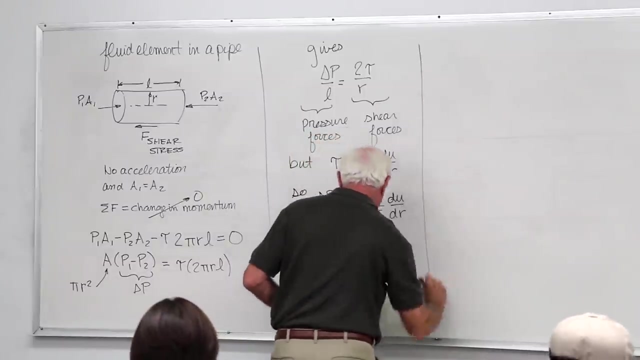 So we have minus 2 U over R D U D R, Rearrange D U D R. And then we have- Let's see, We've got our U D R 2 U L Times R. Put the D? R on the right. 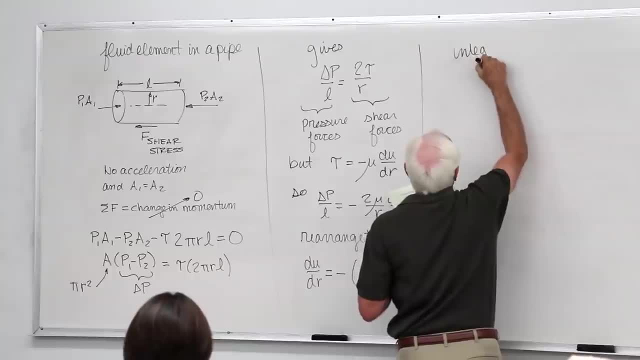 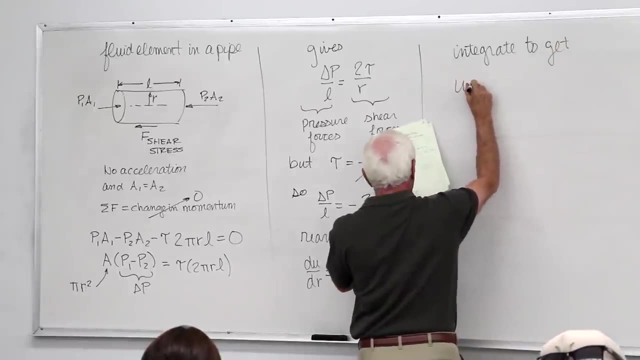 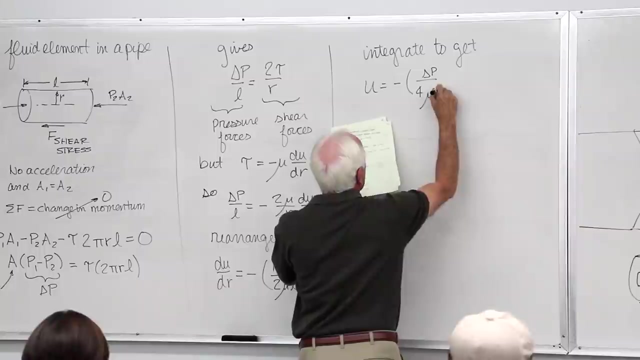 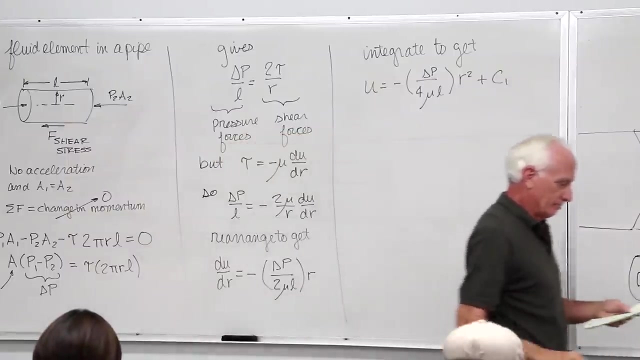 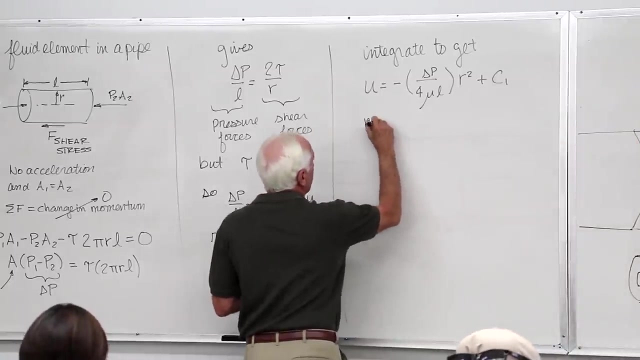 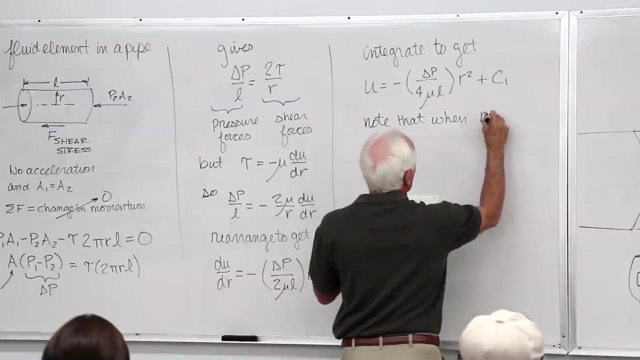 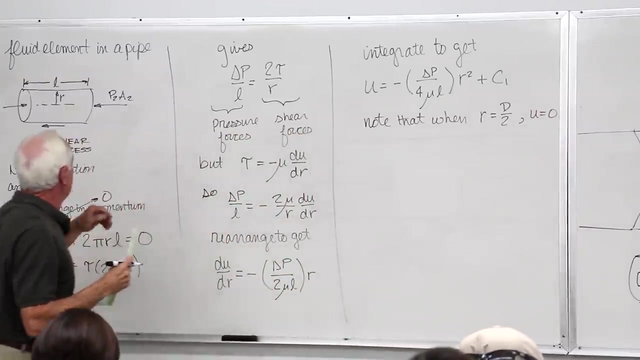 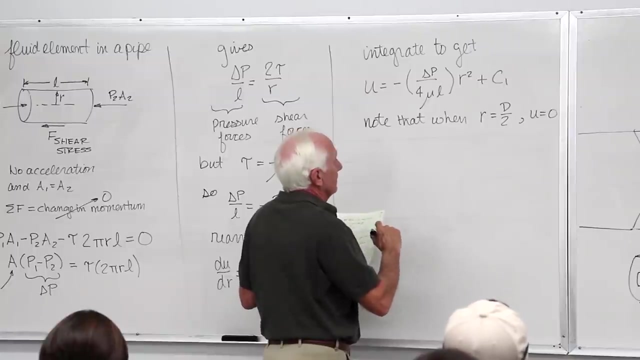 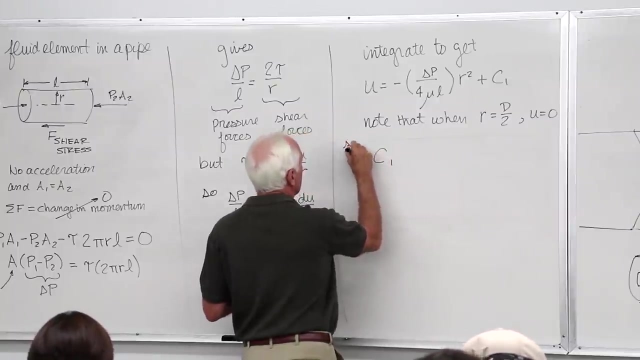 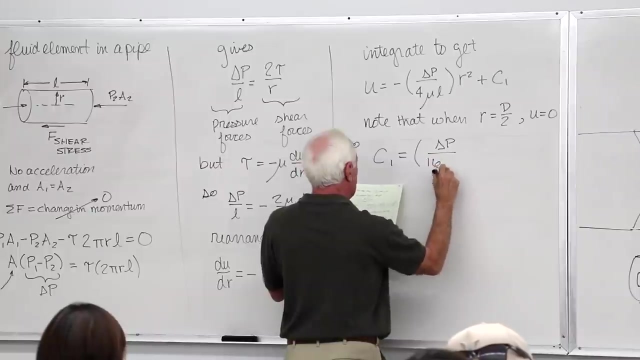 And integrate it. So we have U equal minus Constant of integration, C1.. When the radius is the outside radius, we're going to say that the velocity there is zero. Okay, And so we end up with C1 delta P over 16 mu L D squared. 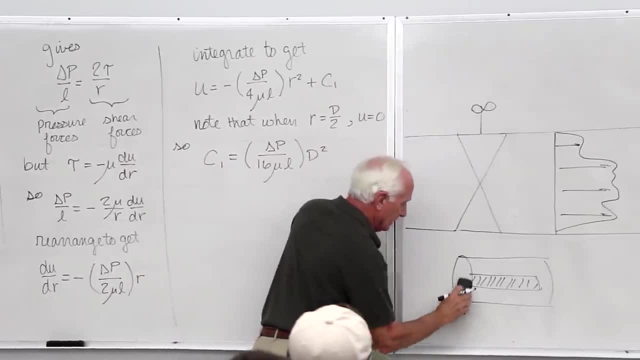 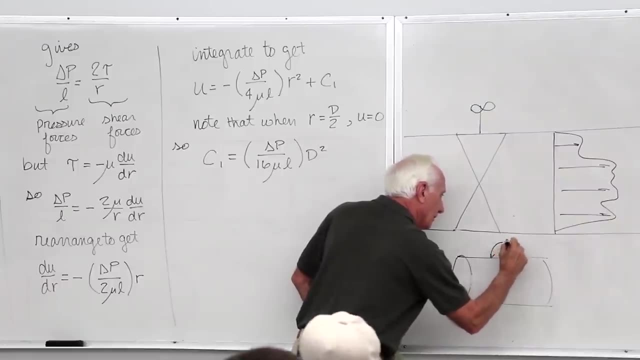 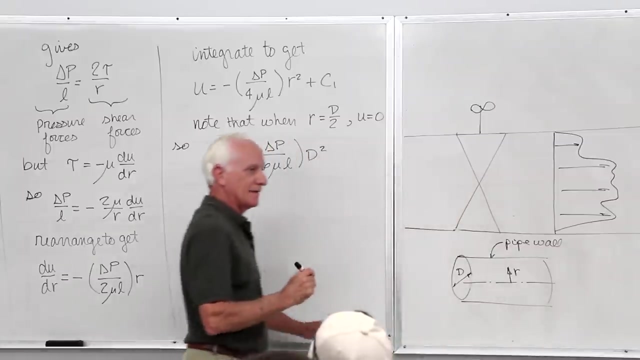 This picture here is not right for that derivation. I'll put it more clearly here for you. This is the pipe wall here, Not a piece that's in the middle. This is the diameter D And this is the radius R. Okay, 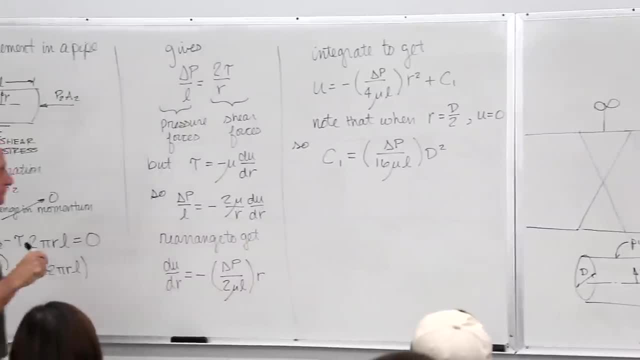 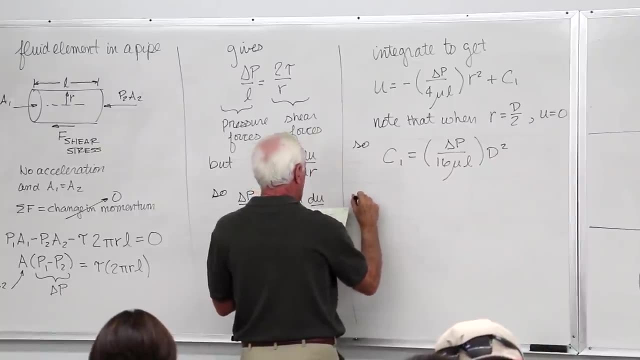 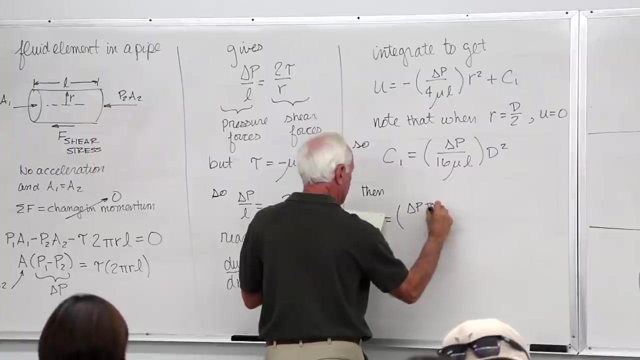 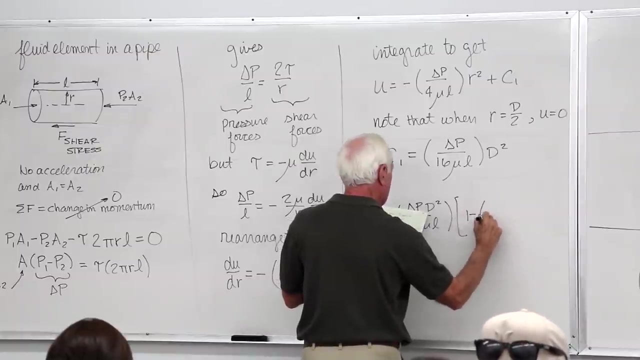 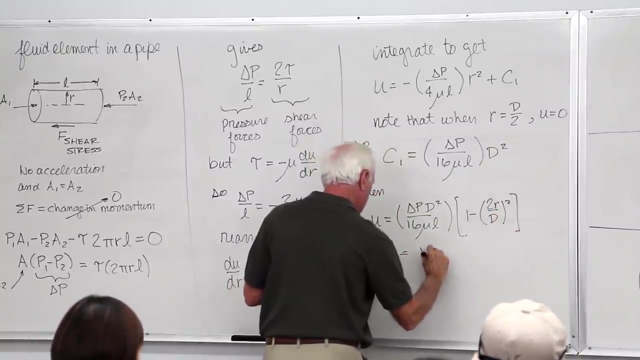 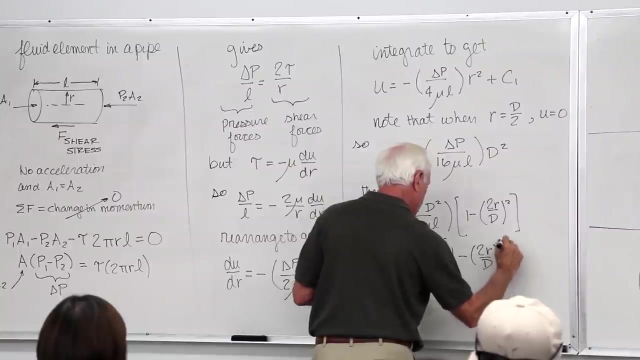 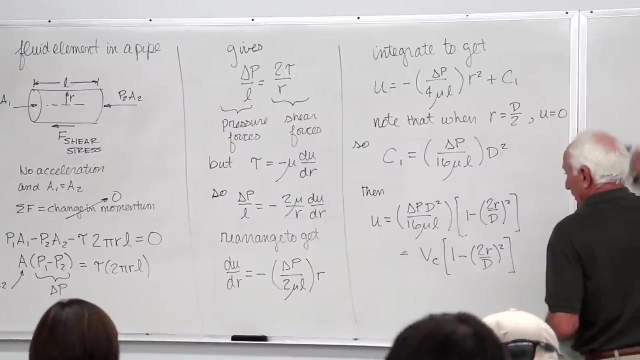 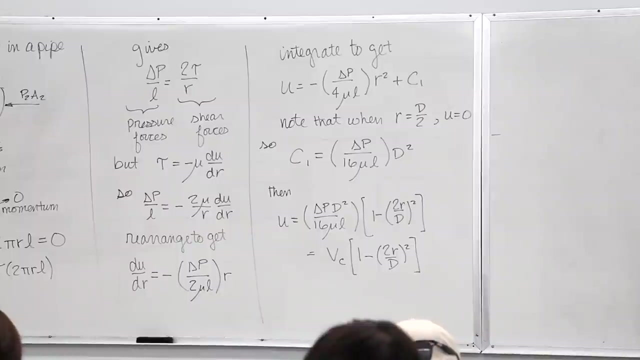 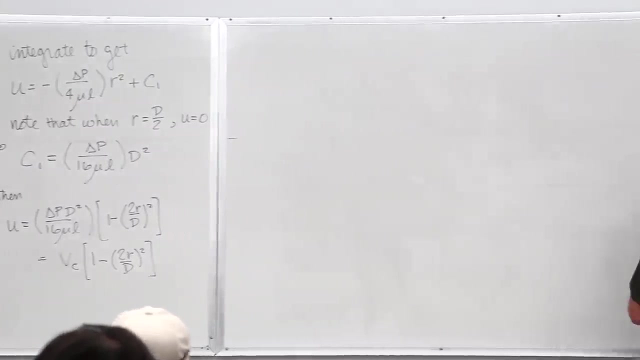 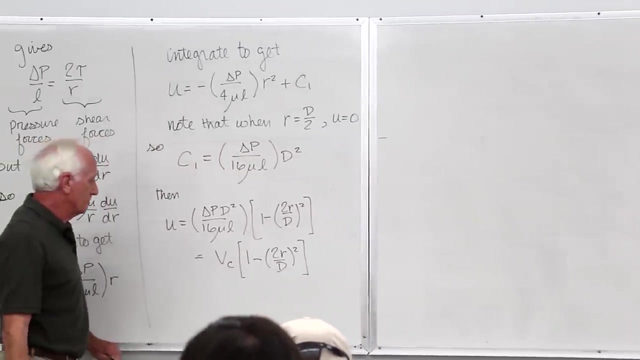 That's the picture that goes with this derivation. Put this guy up in here. Okay, So U then is equal to: And there's the parabolic distribution. Now you can see why. in laminar flow that is parabolic, It's a function of 1 minus a constant times R squared. 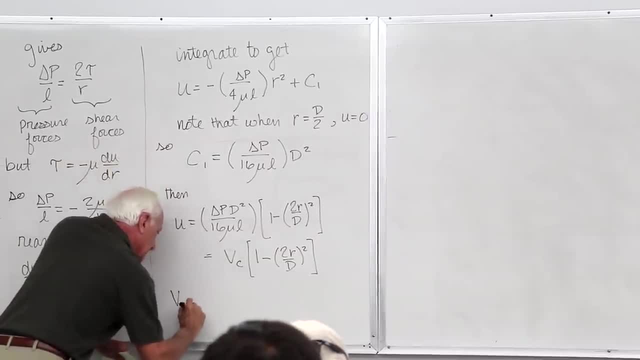 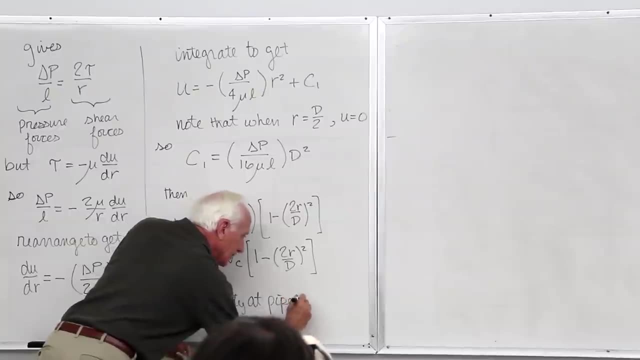 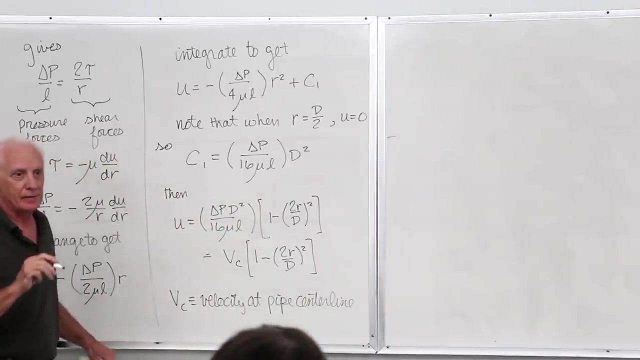 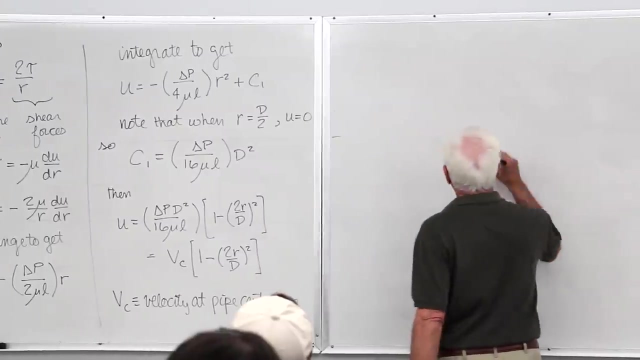 What's this V C mean? This V C is the velocity At the pipe center line. The C stands for center line. Yeah, When would R not be half the diameter? Okay, I want to know, Find the velocity at. This is a 2 inch diameter pipe. 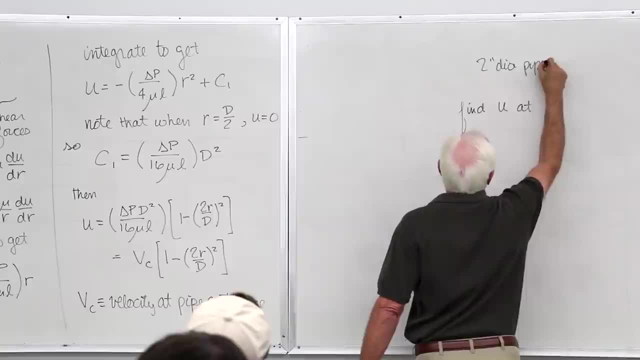 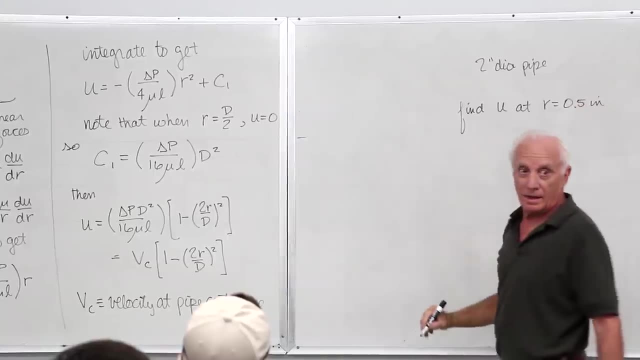 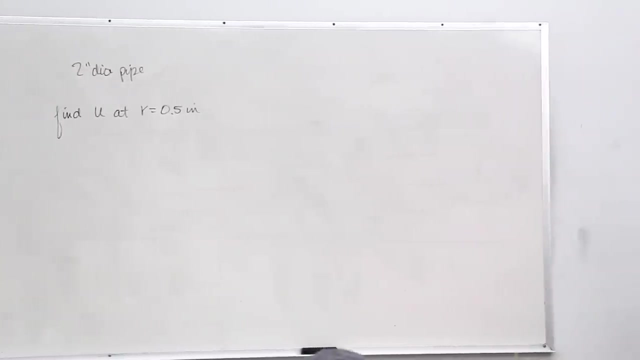 Find the velocity at. This is a 2 inch diameter pipe. Find the velocity at R equal 1 half inch. What's the diameter? 2. What's the outside radius? 1. Where do you want to find the velocity? 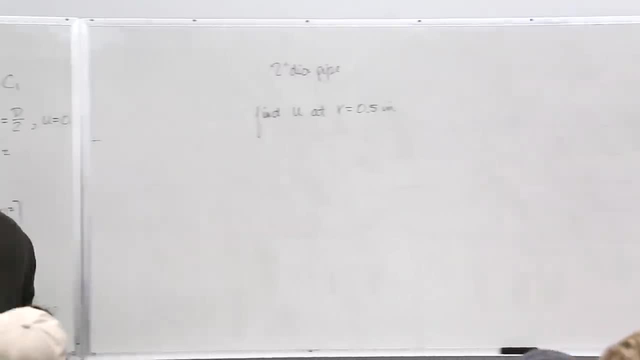 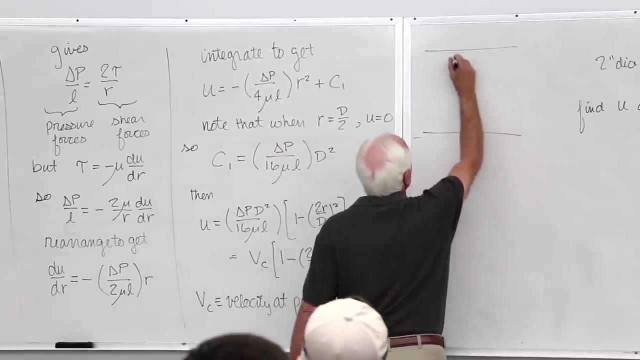 A half inch from the center line. So there's V C. I'll draw a picture here. We know it's parabolic now, So it looks like this: There's V C, center line velocity. Here's the general radius R. 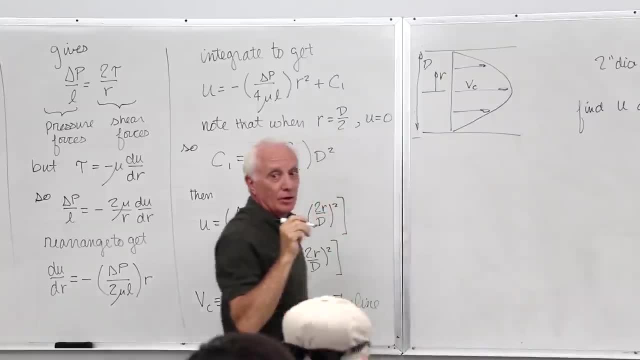 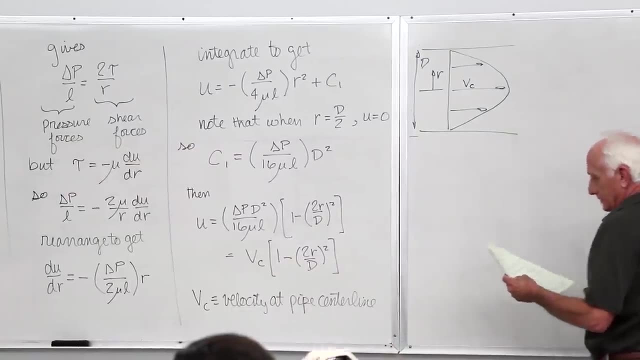 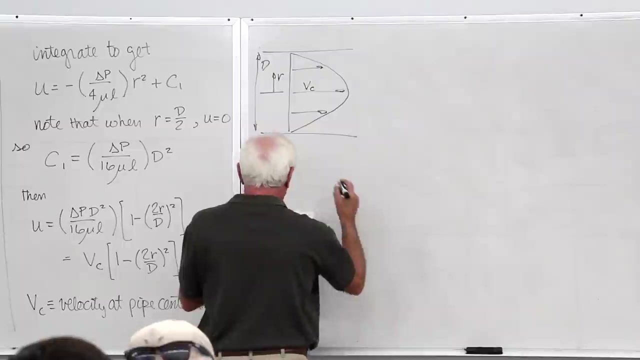 Here's the diameter D. Little R is the radius, Big D is the constant. I want you to find it Okay, So I'm going to use I'll leave it on. I think that was fine. So now there's the. 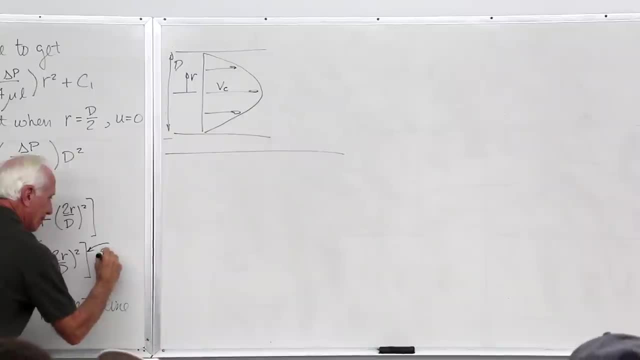 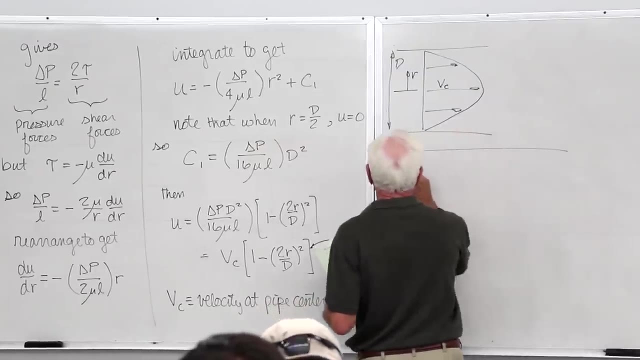 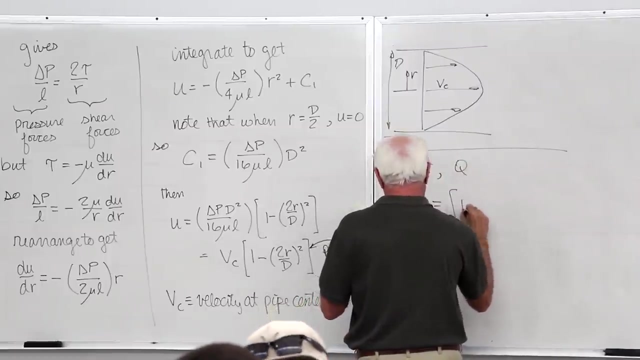 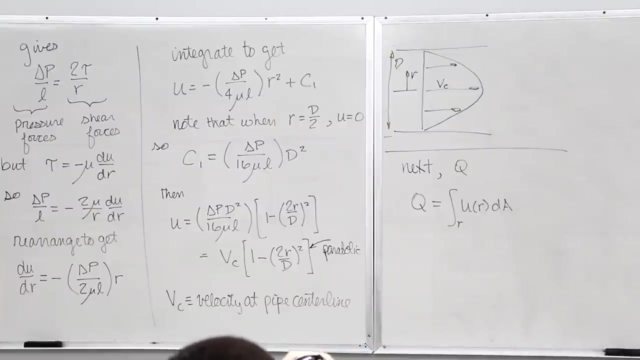 There it is Parabolic. Parabolic- Second one. Next, we're going to find the flow rate. Okay, To find the flow rate, you take the velocity as a function of R, Multiply it by a differential area. Integrate over the total cross-sectional area. 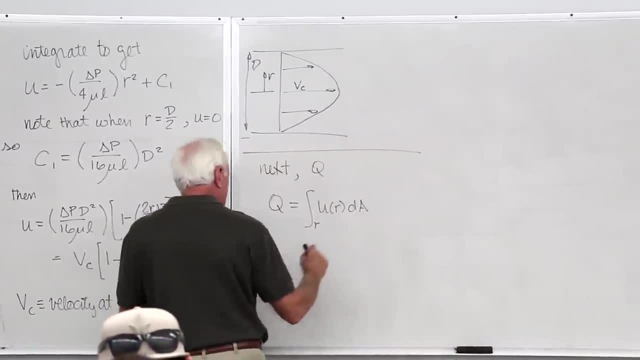 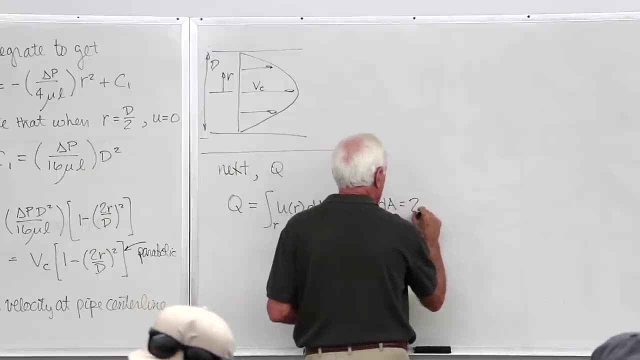 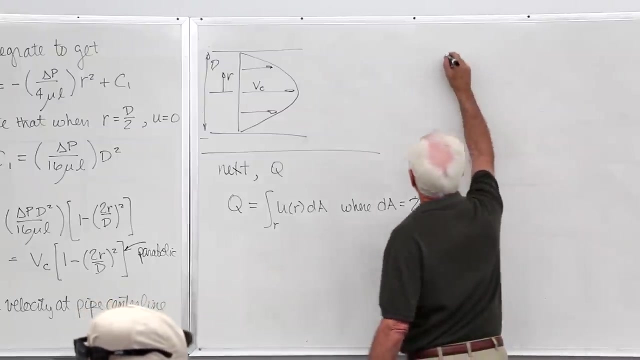 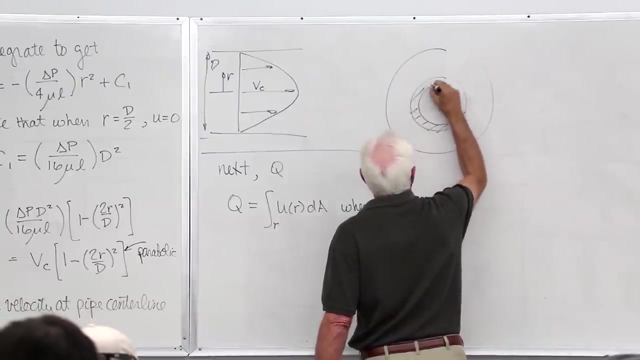 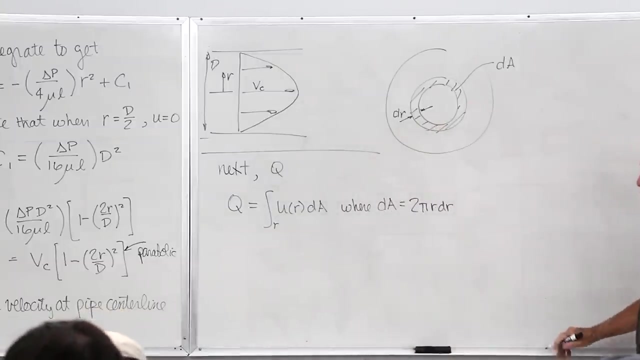 And that gives you Q, Where your DA, your differential area, is equal to 2 pi R DR. Okay, There's your differential area. This distance here is DR. So the area of that little donut shape there is the circumference times the thickness. 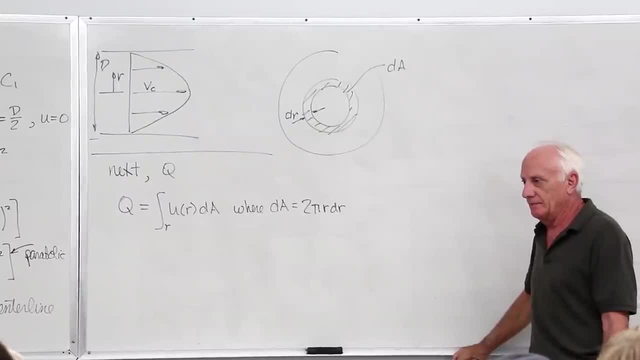 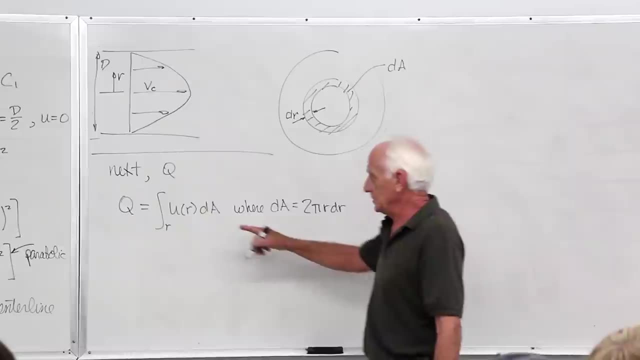 The circumference times the thickness. The circumference is 2 pi R, The thickness is DR. That's how we get the differential element. DA Put this U you found over here in there, Function of R Constant, out in front. 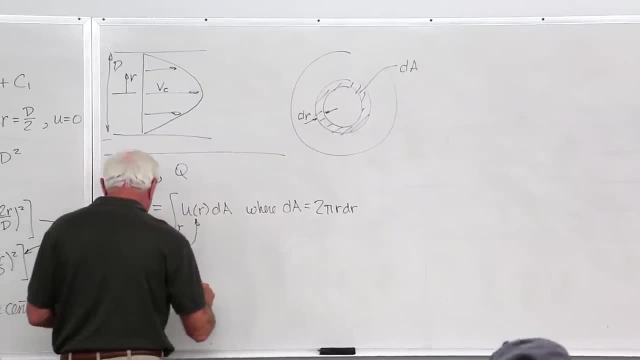 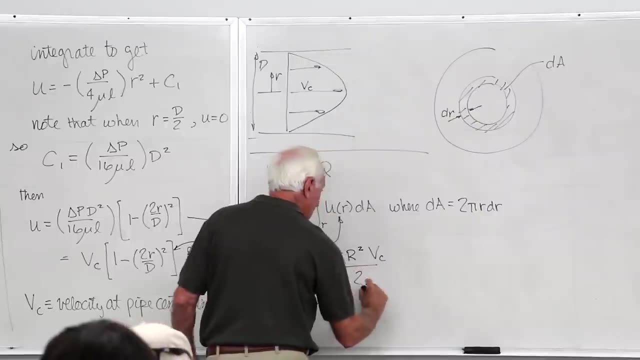 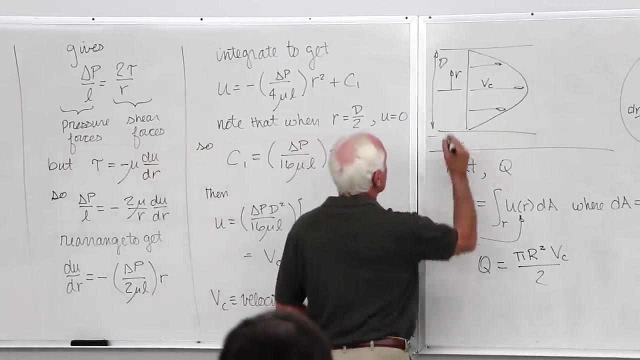 When you do that- we won't go through all the gory details- You get Q equal pi R squared VC over R. Okay, Number 2.. And our textbook calls the outside radius capital R, So here this is capital R. 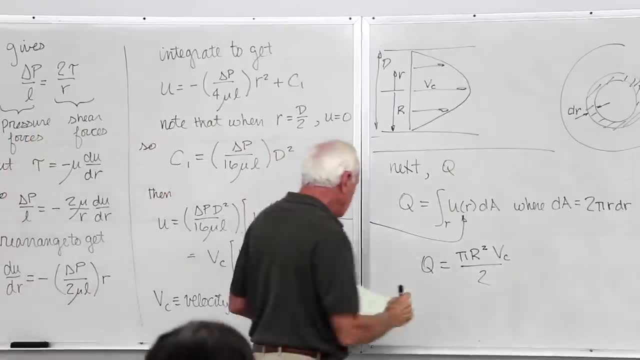 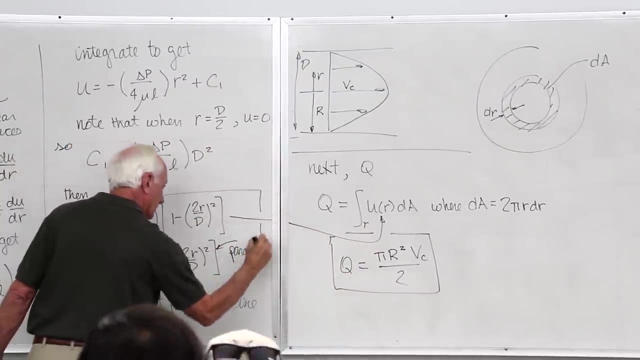 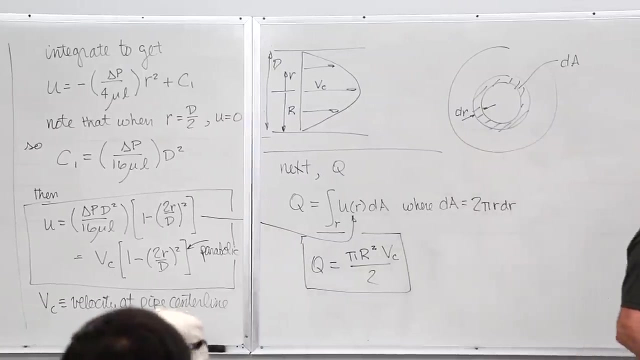 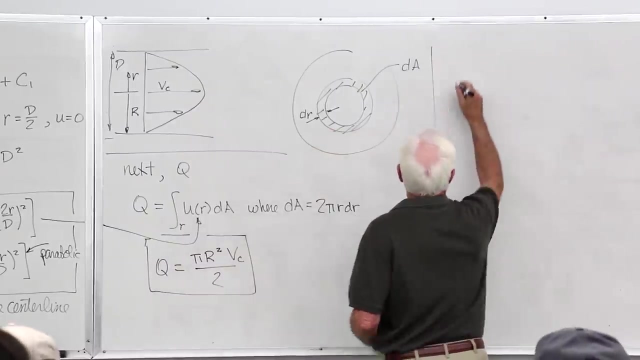 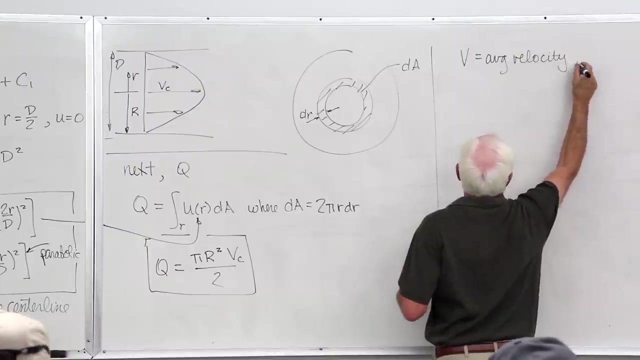 Capital R is 1 half capital D. There's Q. Let's box in the important equations. Okay, We're almost there. Now, if I want to find the average velocity, I take the flow rate Q. I just found it. 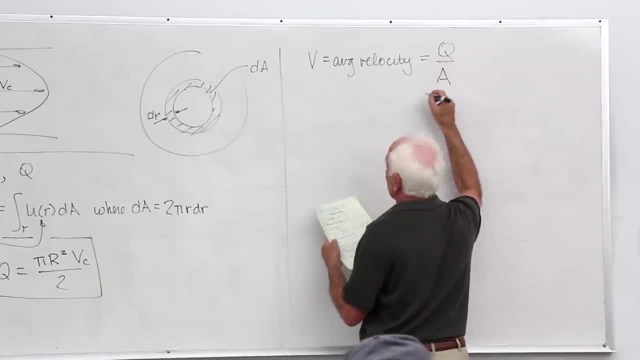 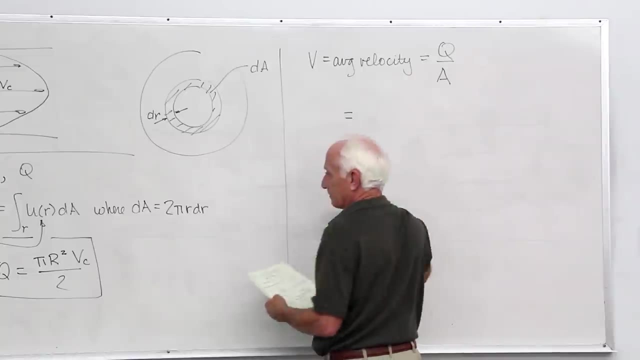 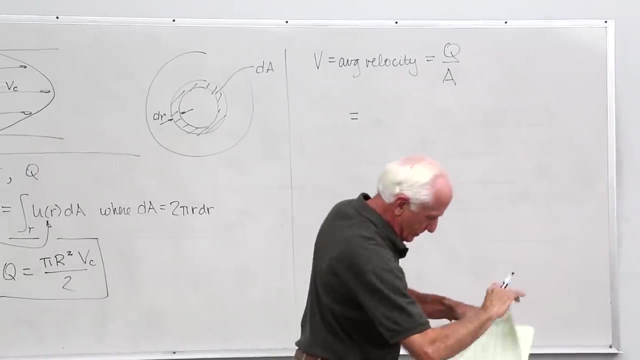 I divide it by the cross-sectional area A, And that's the average velocity. So the flow rate Q. Let's see what we get over there. Let's see where our Q is: Q, Q, Q, Q. We need one more equation, I think. 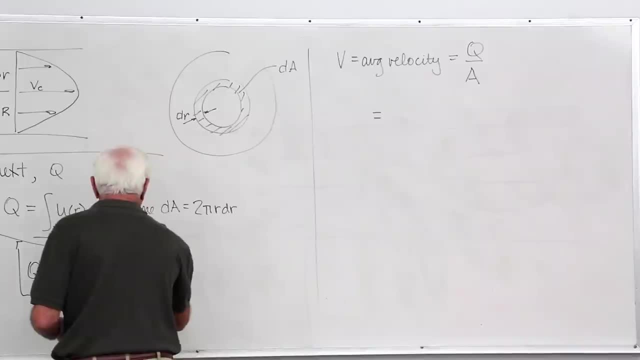 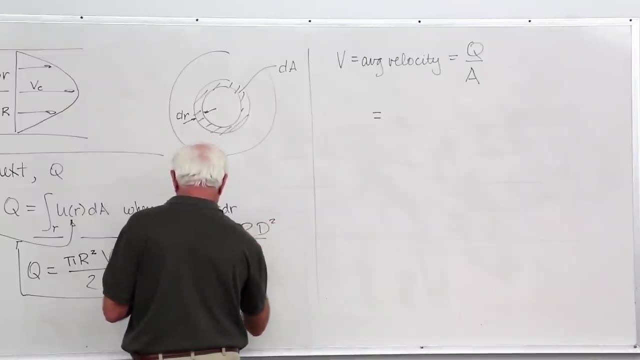 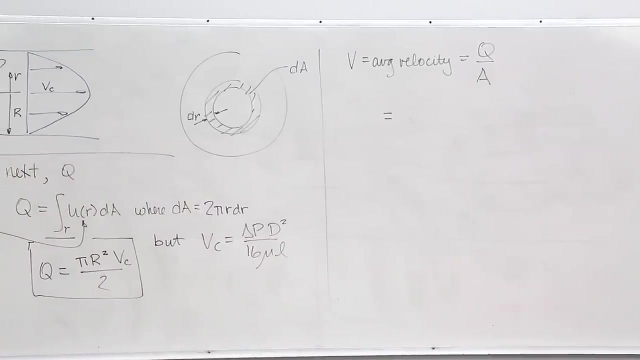 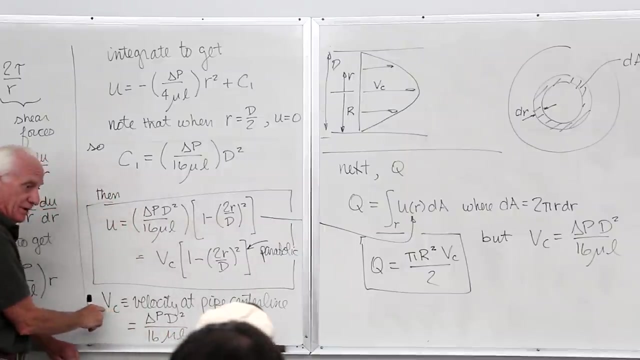 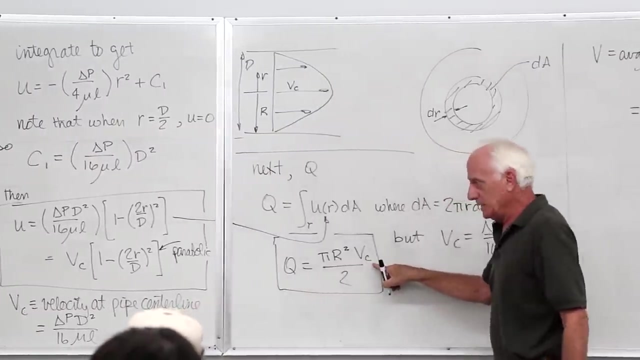 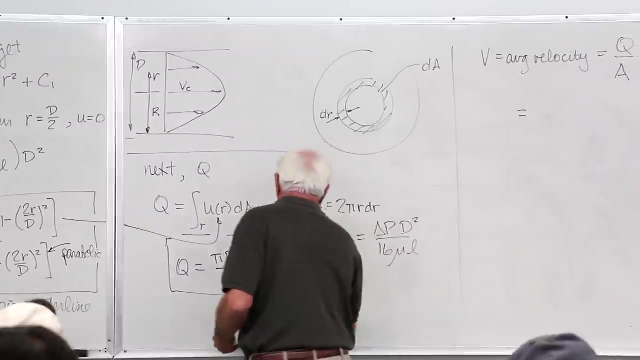 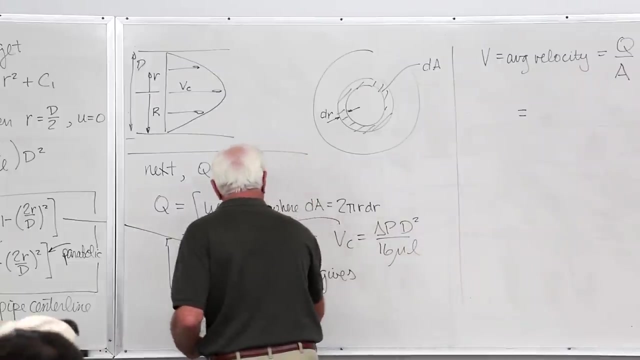 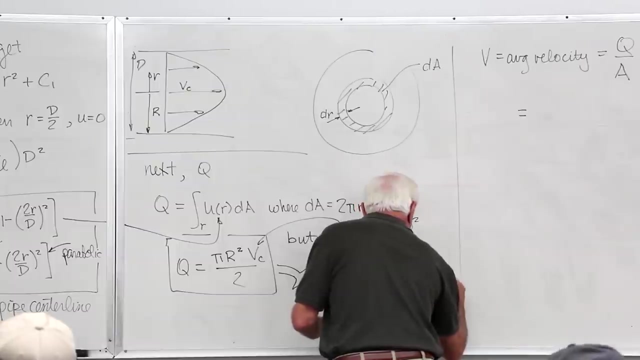 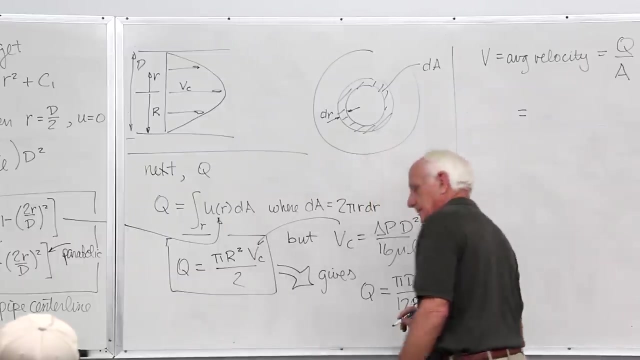 Oh yeah, Okay, That's our Q right here. There's our center line velocity. from here I now, where I see that V sub C, I put in that which is that, Put that in here for VC. That gives, then that gives Q. 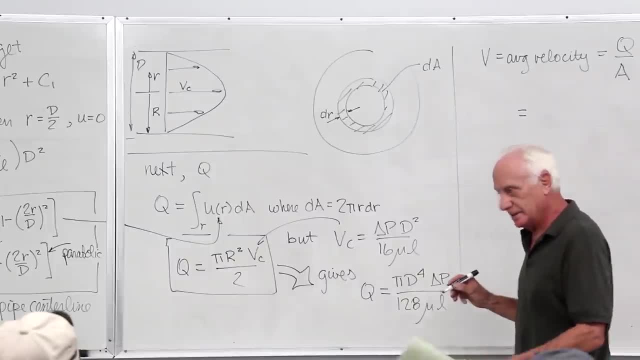 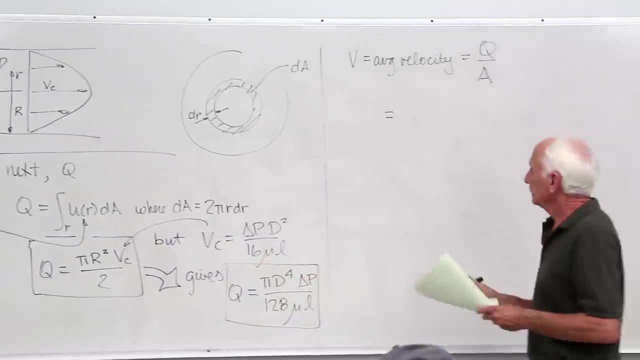 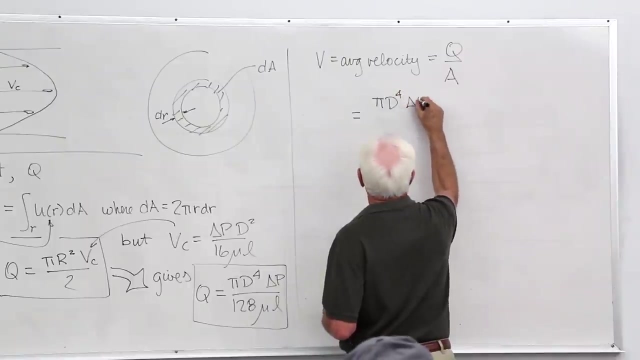 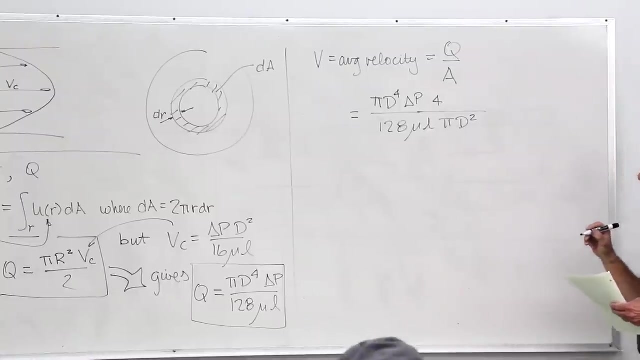 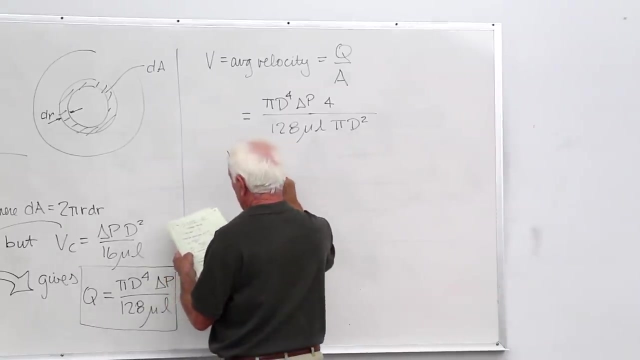 These equations that I'm boxing are all in the textbook. Okay, Okay, Okay, Okay, Okay, Okay, Put that Q up here: Area pi over 4 d squared. Pi over 4 d squared, So we end up with the average velocity then.